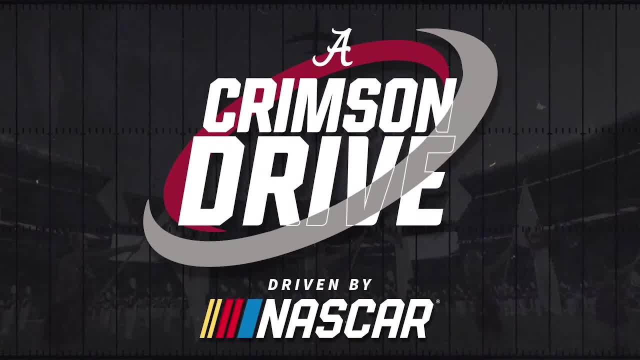 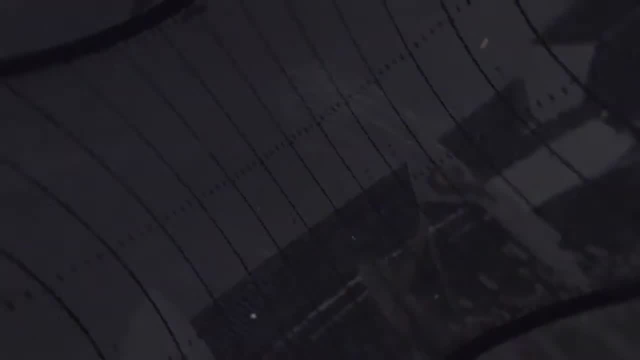 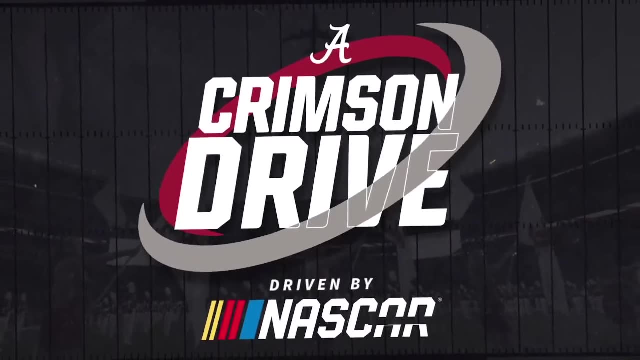 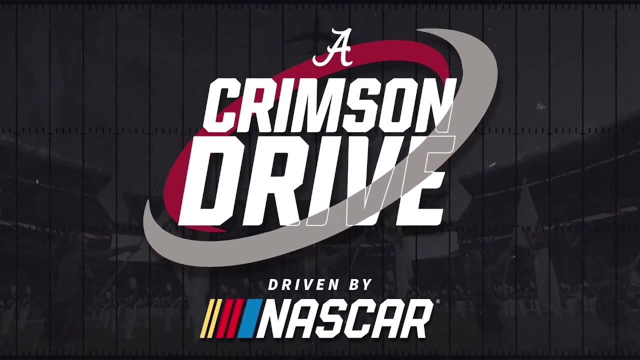 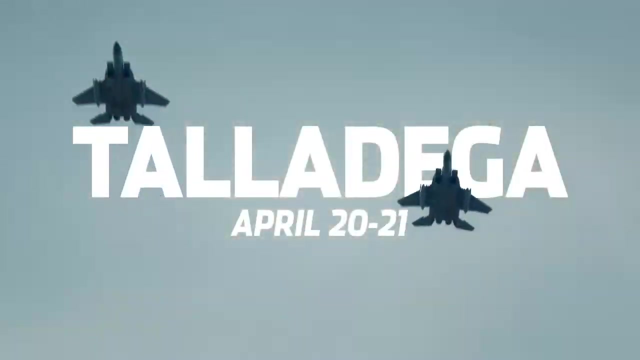 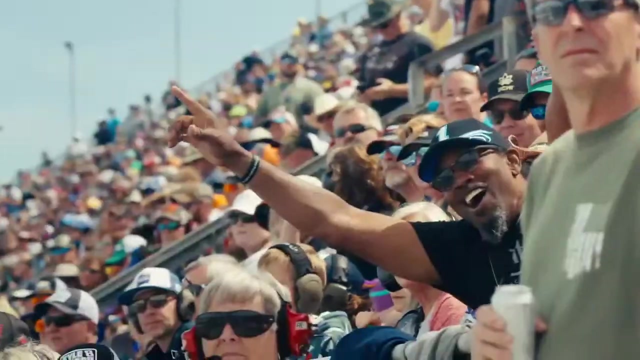 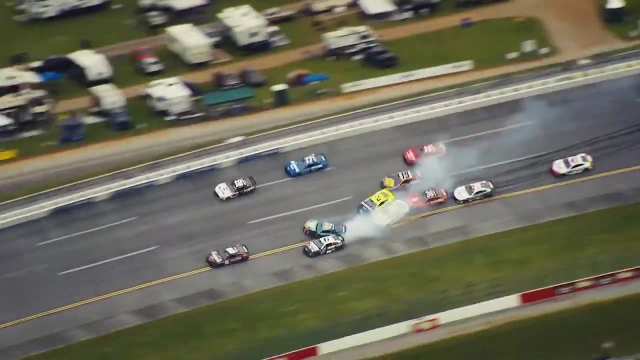 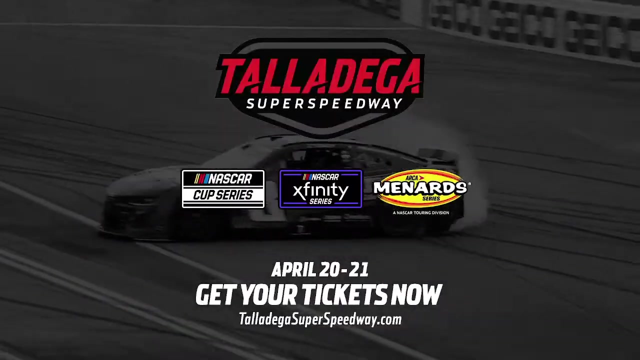 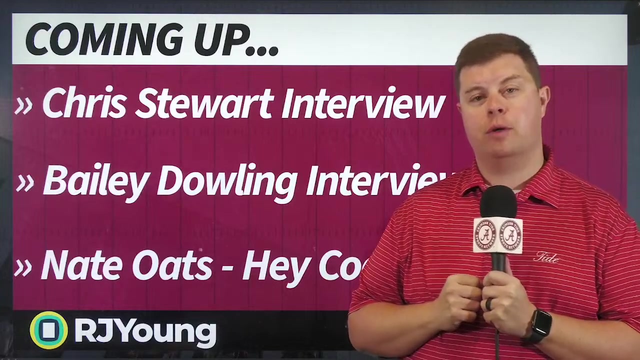 Thank you. Thank you. Get your tickets now at TalladegaSuperspeedwaycom Roll Tide and welcome to this Thursday edition of Crimson Drive driven by NASCAR. This is Roger Hoover with you from our Tuscaloosa studios as we get set for a very busy show. 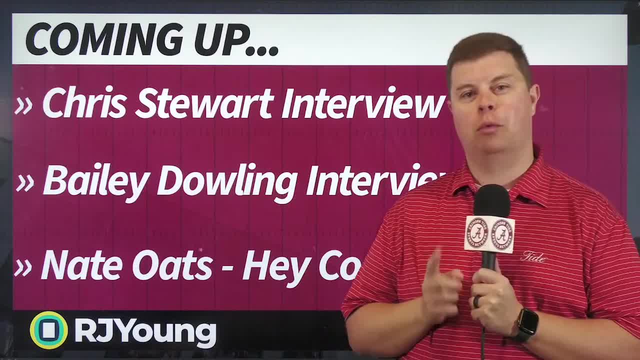 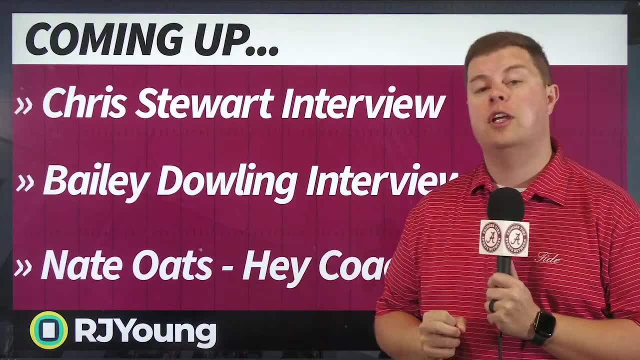 taking a look at Alabama men's basketball in the Final Four. We'll be talking about that in a conversation with Chris Stewart as we go through everything coming up on our show for today, thanks to our friends at RJ Young. RJ Young is the official technology solutions provider of Crimson Drive. 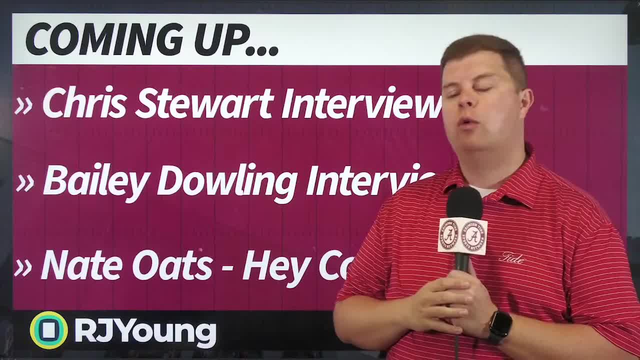 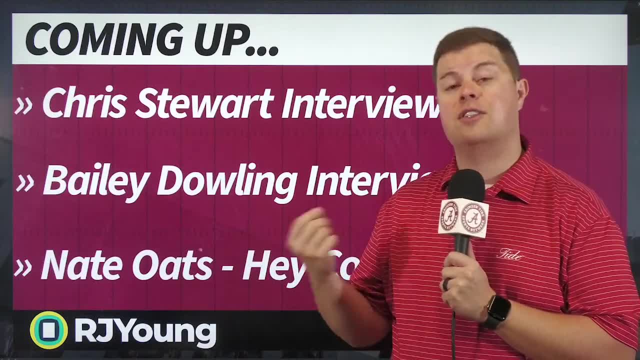 They've given us a smart board to go through everything in a real interactive way Throughout our headlines. But again, Chris Stewart will start the show as he got to make the call he has been dreaming of making for years and years and years: that Alabama men's basketball is headed to the Final Four. 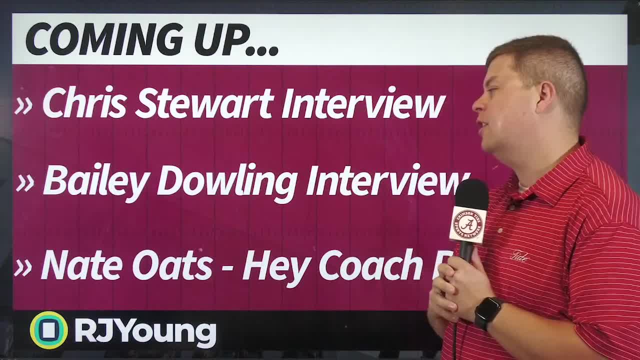 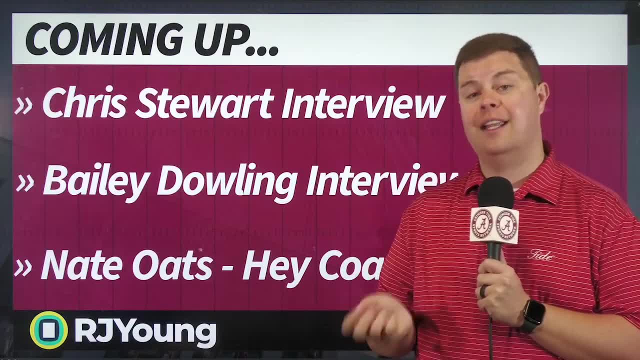 We'll talk about that with Chris to begin our show, and then we'll have a conversation with Bailey Dowling, third baseman for the Crimson Tide softball team, One of the first interviews we have recorded at the Advantage Center inside Bryant-Denny Stadium. 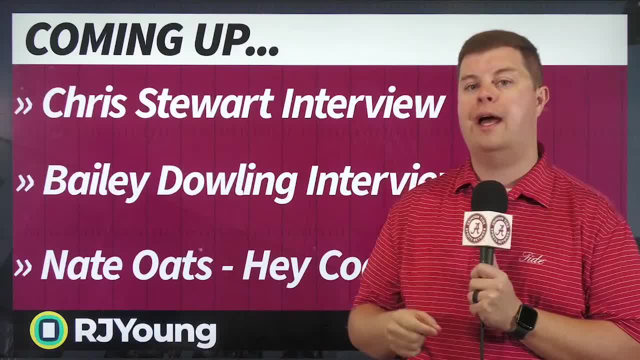 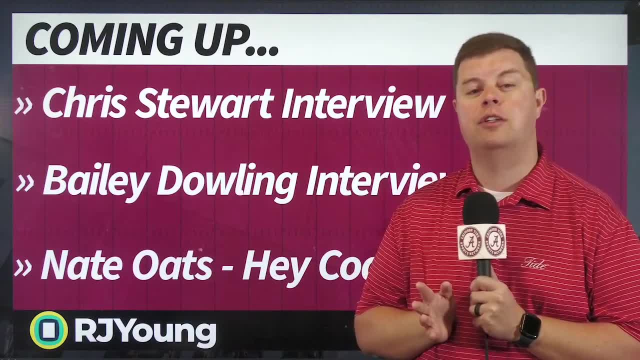 Fun conversation with Bailey Dowling about her journey from Illinois to Alabama and what's ahead for Team 28.. Then we'll take a look back to A great addition that we had on Monday night of Hey Coach, presented by Alpha Insurance at Baumhauer's here in Tuscaloosa. 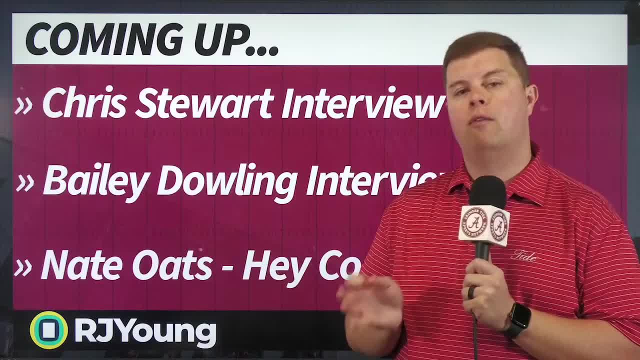 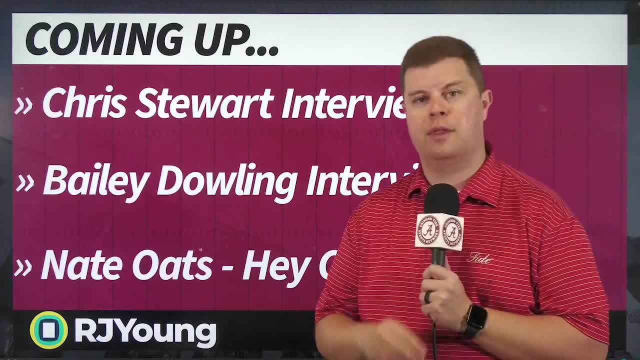 Not only did we have Nate Oates, but we had a full preview of what's coming up for this weekend. It is available to watch on demand on the CTS and YouTube page, as well as the Alabama Insider podcast. But, Nate Oates, we'll get some thoughts from the head coach of the Crimson Tide as we get set for Alabama men's basketball in the Final Four. 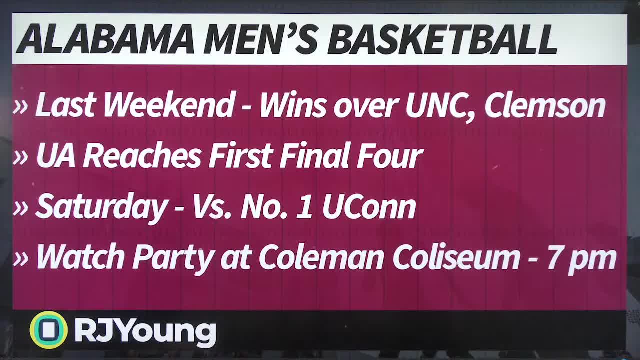 The Crimson Tide, of course, reaching the Final Four. First of all had that Sweet 16 win against North Carolina, And then Clemson took care of business, And the Elite Eight as the Crimson Tide make it to the first Final Four in program history. 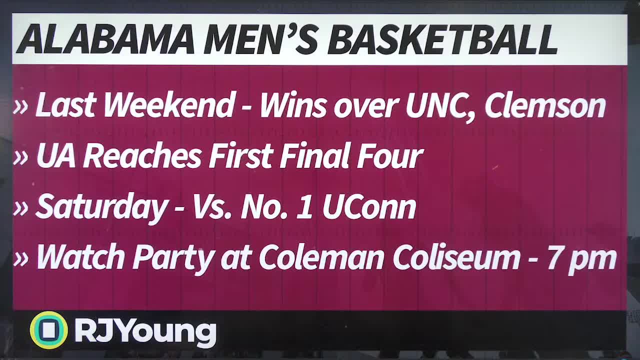 Great opponent on the other side, The defending national champion, UConn Huskies, a number one seed in their own right for this tournament. They will be a tough opponent coming up on Saturday. Our radio start time will be at 630. 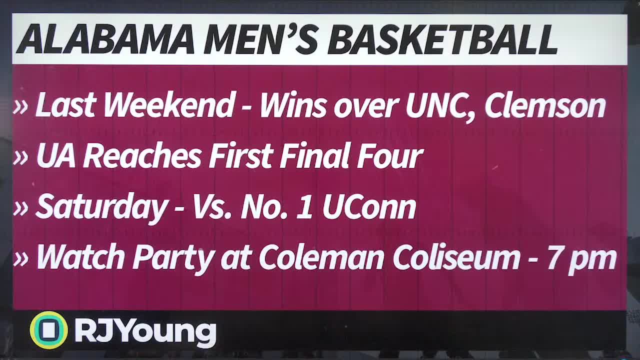 Don't forget as well. at 7 o'clock the doors will open at Coleman Coliseum for fans in Tuscaloosa. Make sure you go to the watch party, as CBS will have cameras there. Your reactions will be shown on the broadcast. 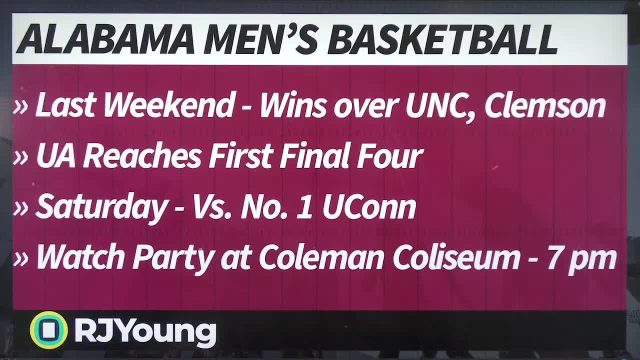 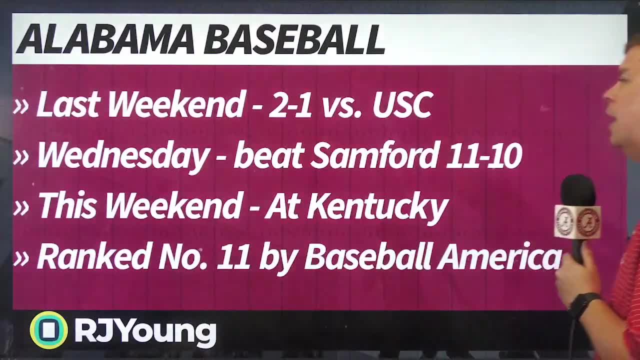 Should be a lot of fun that watch party coming up. I hope they'll do that as well coming up Monday. if Alabama is able to reach the national championship game, I imagine they would be. But Roll Tide to Alabama men's basketball in the Final Four. 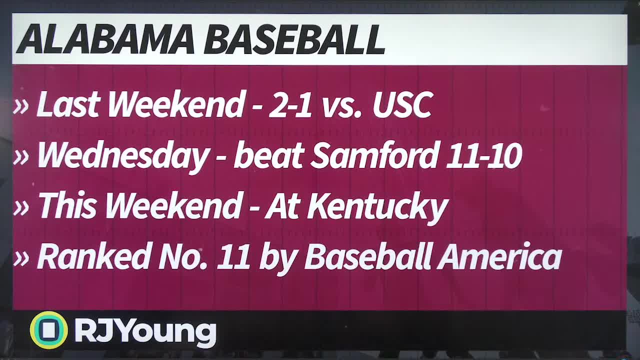 Taking a look at Crimson Tide baseball. Alabama last weekend won the first two games against South Carolina before dropping the finale by only a run. So a really good performance against a top ten South Carolina team. as Alabama once again won a home series Now on Wednesday, the Crimson Tide yesterday actually had a trip to Sanford in Birmingham. 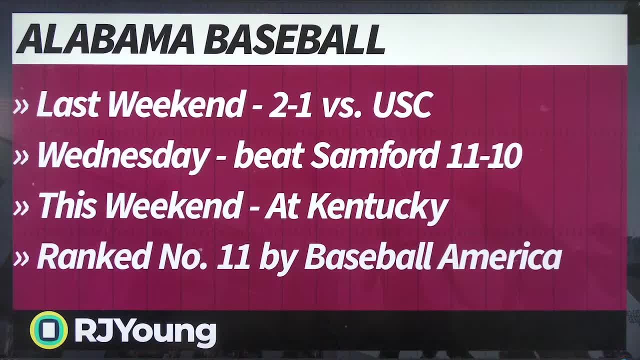 and picked up an 11-10 victory. A game that featured two games, Two home runs by Gage Miller, TJ McCants, Ian Petratz, also homering for the Crimson Tide as Alabama held on in the end to get that 11-10 win over the Sanford Bulldogs. 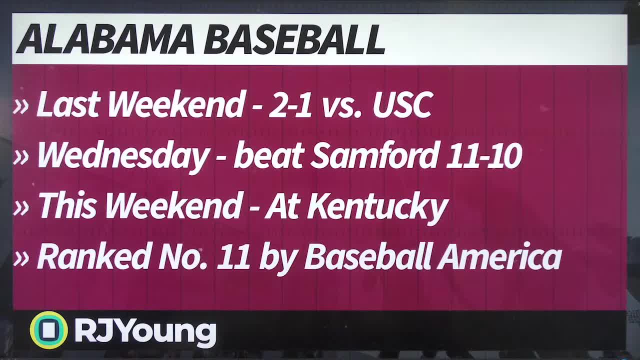 Now this weekend the Crimson Tide taking on the Kentucky Wildcats, a team that may be ranked behind Alabama, but Kentucky is off to an 8-1 start in SEC play, The Crimson Tide 4-5, but Kentucky and Arkansas are really the two outliers in SEC baseball so far. 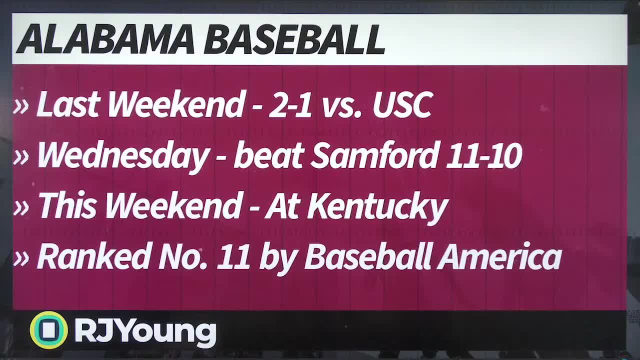 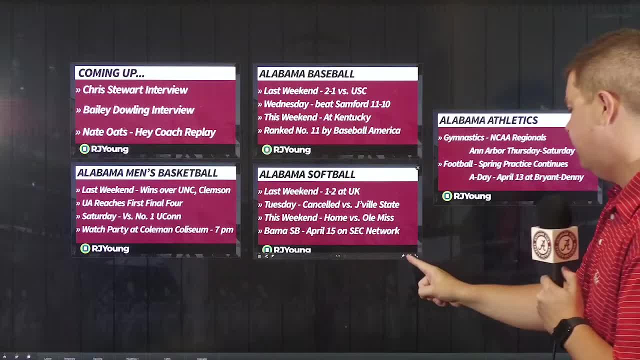 with 8-1 marks through the first nine games of SEC play. Crimson Tide, on the strength of that series, win South Carolina now ranked 11th in the country by Baseball America, The Crimson Tide softball team. last weekend they were also in Lexington against Kentucky. 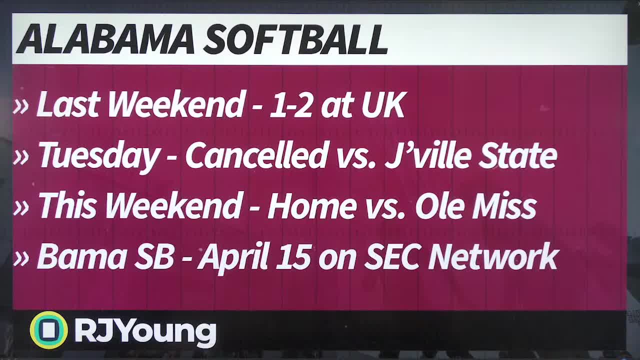 and ended up going 1-2 against the Kentucky Wildcats. Earlier this week they were scheduled to play Jacksonville State, but that game was postponed due to, or really just canceled due to all the inclement weather we had around the state Now this weekend and the next weekend, as you'll hear Bailey Dowling talk about in a moment- 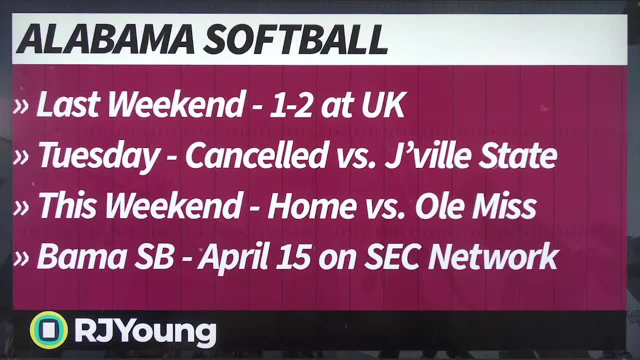 home softball coming up at Rhodes Stadium First of all. this week it will be Alabama against Ole Miss. And don't forget, there's going to be a great documentary done by SEC Story on the SEC Network coming up on April 15th. 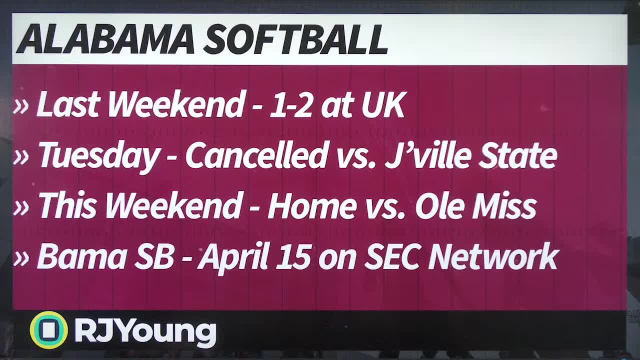 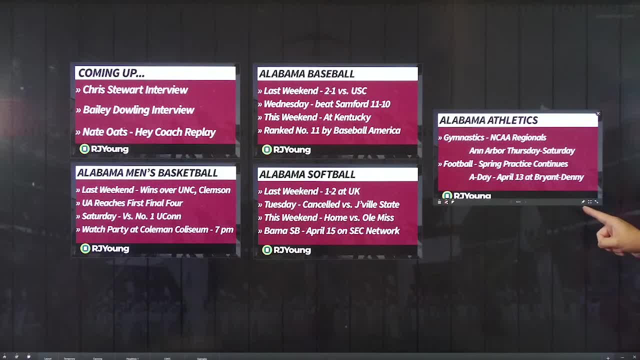 It'll be Bama softball- the story of the 2012 National Championship team for the Crimson Tide, So we look forward to watching that. Patrick Murphy's been tweeting about it and we're certainly excited to see that on the SEC Network on April 15th. 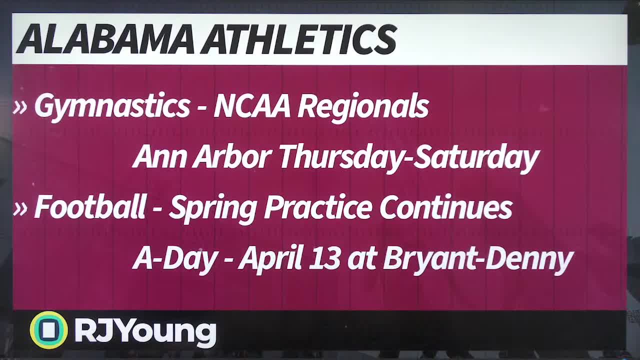 A few other notes: gymnastics starting today in the Ann Arbor Regional in the NCAA. So really hope the Crimson Tide can continue this season to the NCAA Championships. Best of luck to Ashley Johnston and the Crimson Tide. Football, spring practice continues and we'll be talking more football, of course. 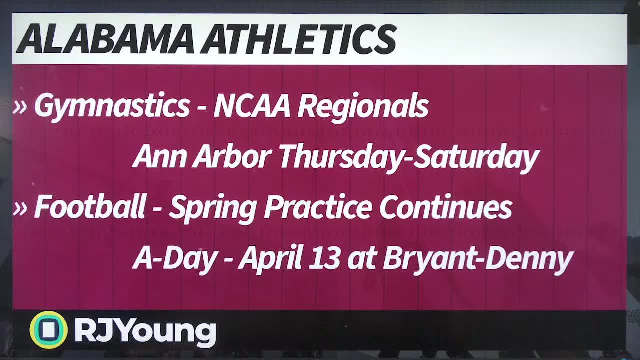 next week, with A-Day right around the corner, April 13th at Bryant-Denny Stadium at 3 o'clock. Our radio coverage will start at 2.30 pm. We can't wait to be back inside Bryant-Denny Stadium for the Golden Flake A-Day game coming up on April 13th. 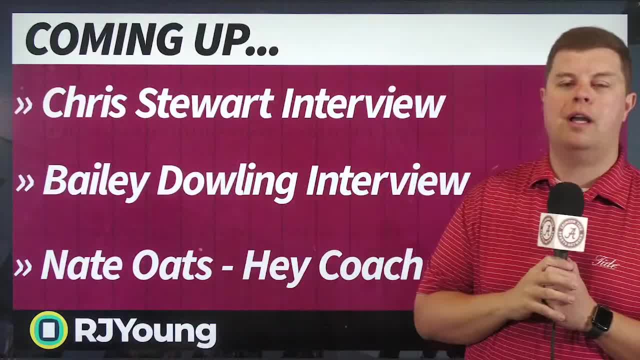 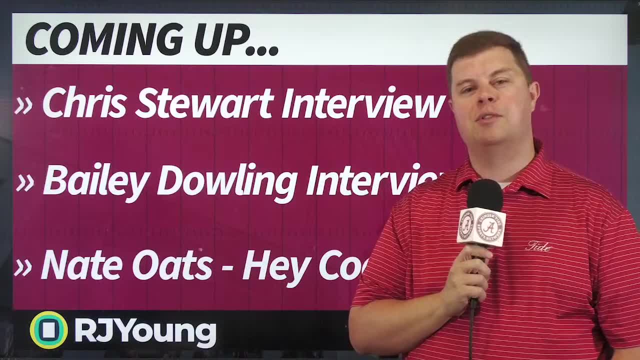 Chris Stewart will be calling that for us here on the Crimson Tide Sports Network on Play by Play. He'll also be calling Alabama basketball in the Final Four. Over 20 years for Chris as the voice of Alabama men's basketball. finally, this moment is here. 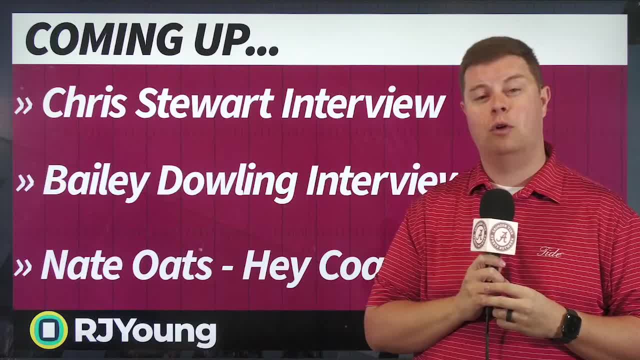 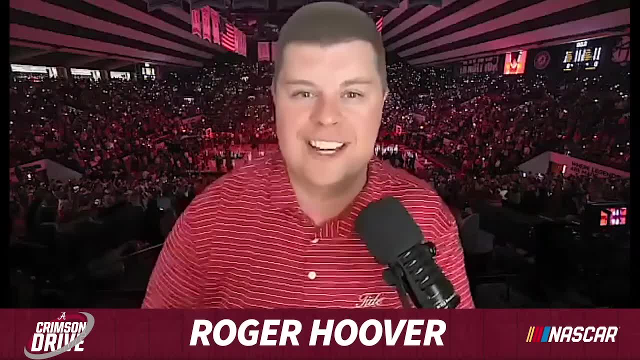 We caught up with him in Phoenix to get a preview of Alabama in the Final Four. Roger Hoover, great to be with you from Alabama, but we keep talking with somebody on the West Coast and we'll count Arizona as part of that for this week's show. 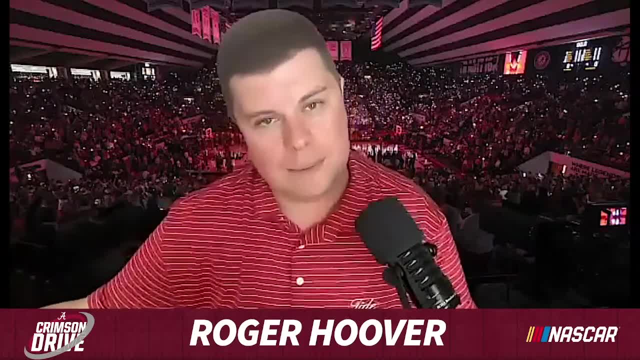 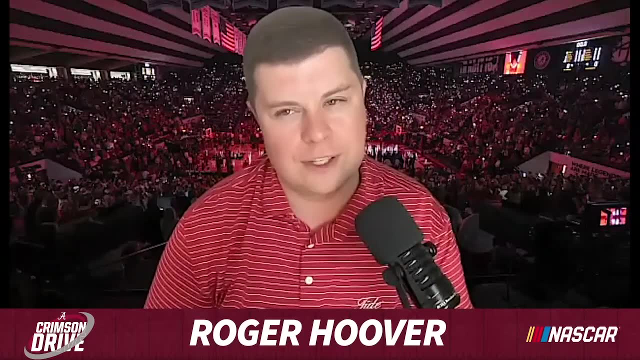 Chris Stewart, who's been from Spokane to Los Angeles, back to Alabama for a bit now in Phoenix, Arizona. And Chris, you're there because the Tide keep rolling all the way to the Final Four- Roll Tide. it's fun to talk about basketball here in April. 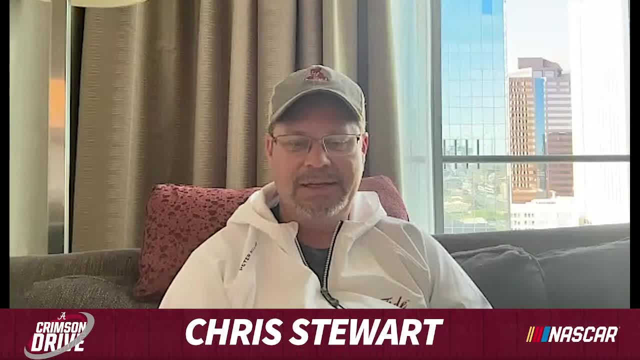 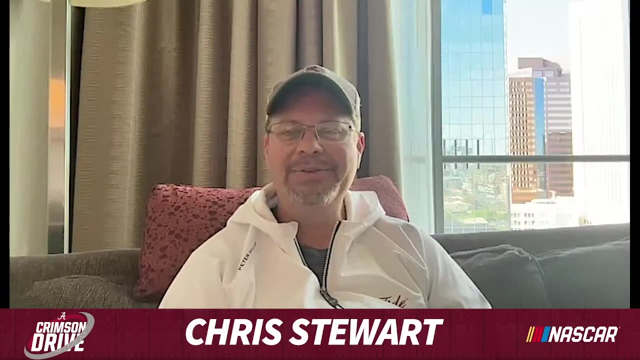 Boy it is. and a special time, Unbelievably special experience. And, yeah, 12 straight days: Tuscaloosa to Spokane, to LA, back to Tuscaloosa And a day and a half at home and then right back out to the West again. 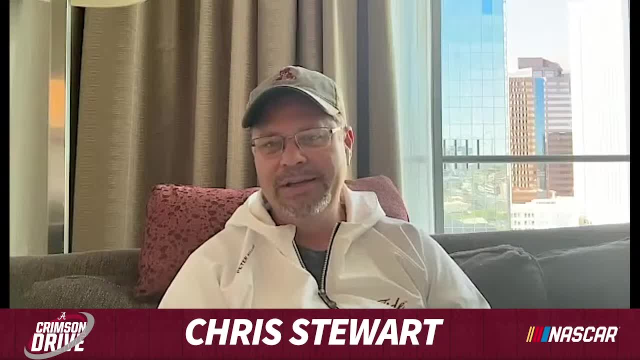 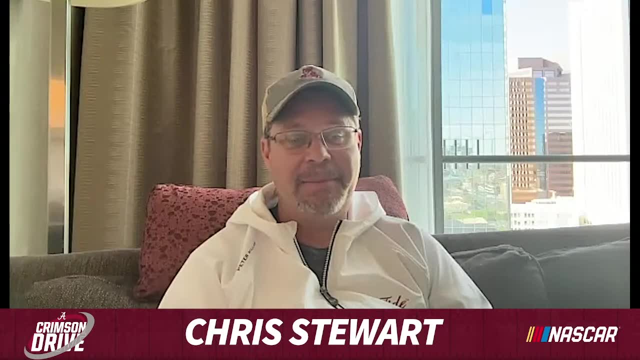 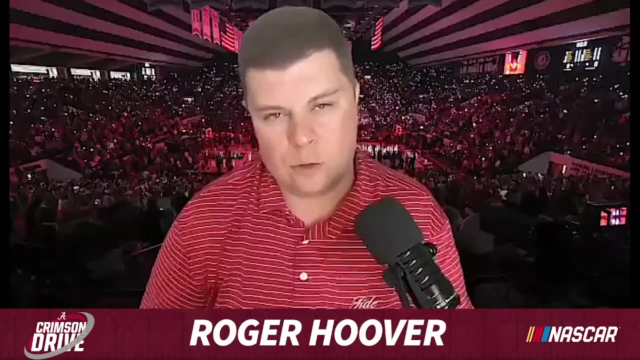 Really really cool environment, cool setting, wonderful greeting for the team yesterday when we got here And it's got a. It's got a big-time event vibe, and that's because that's exactly what it is. Same thing could have been said about last week's trip to Los Angeles. 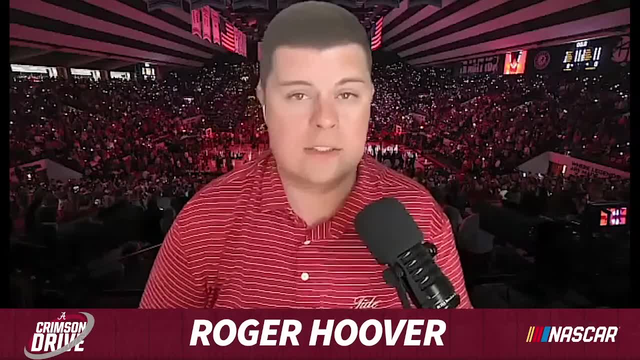 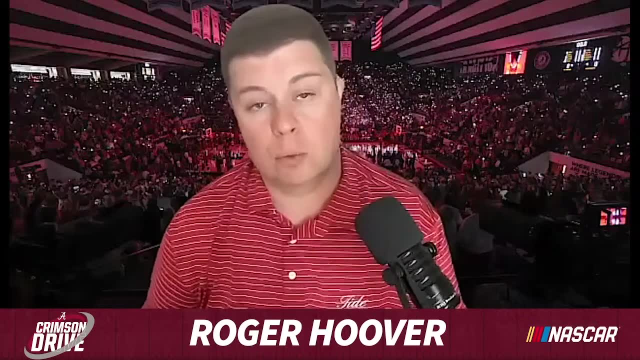 for the Sweet 16 and the Elite Eight, Crimson Tide getting two wins against North Carolina and then Clemson to reach the Final Four. Take us back to that North Carolina game. Obviously the Tar Heels the number one seed in that region. 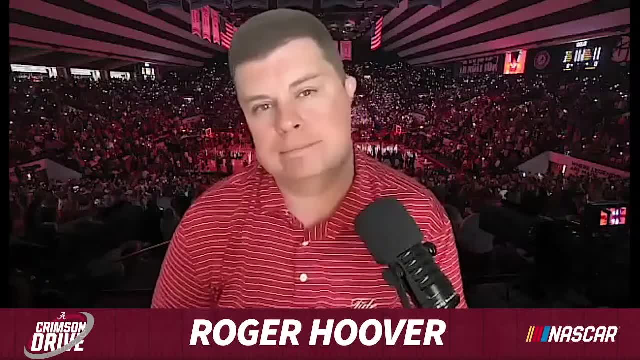 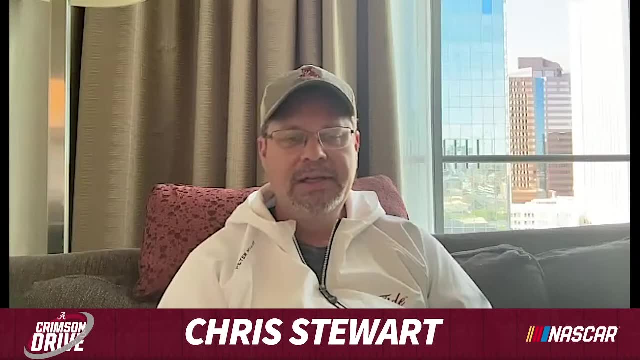 What had to go well for Alabama to have success. first of all, in that game Could not allow the Tar Heels to get a lot of second and third, Could not allow the Tar Heels to get a lot of second and third. They had a lot of second-chance opportunities, defended at a high level. 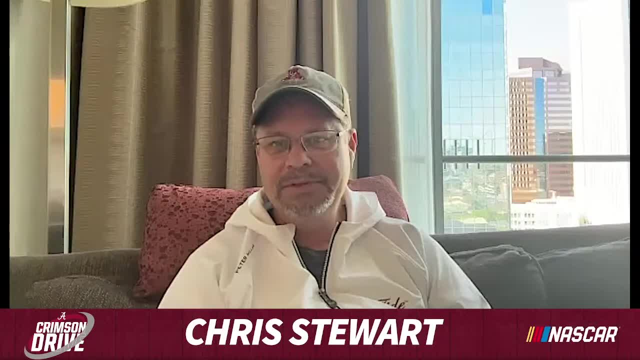 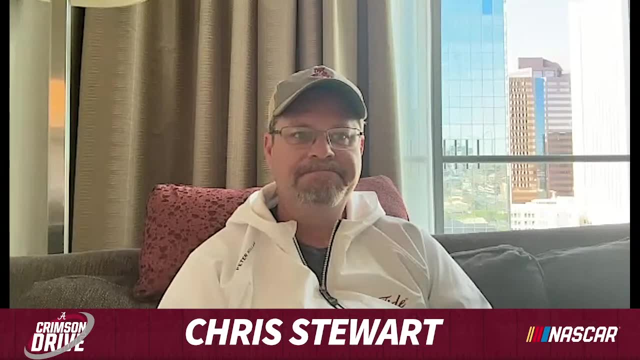 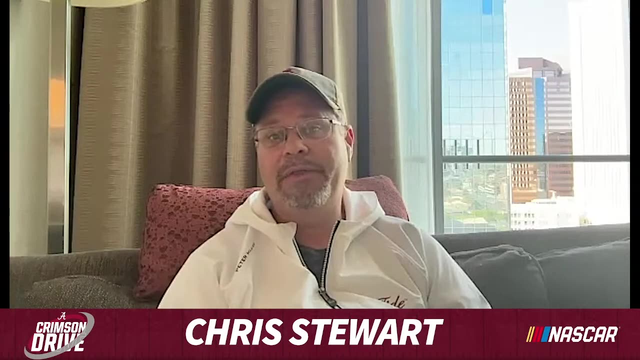 made sure that they did not give up a ton of second-chance looks for the Heels shot it well and continued to guard at a level that exceeds what they had done throughout a good bit of the regular season. So you know, I think that's amazing. 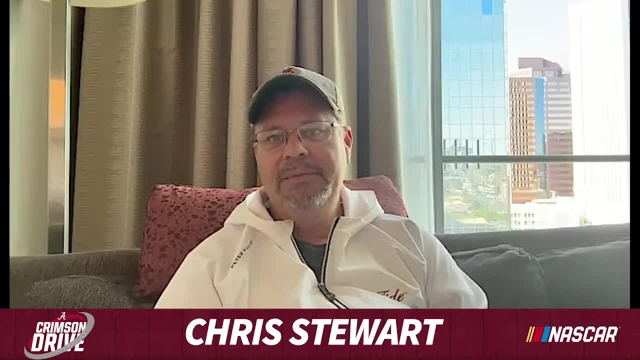 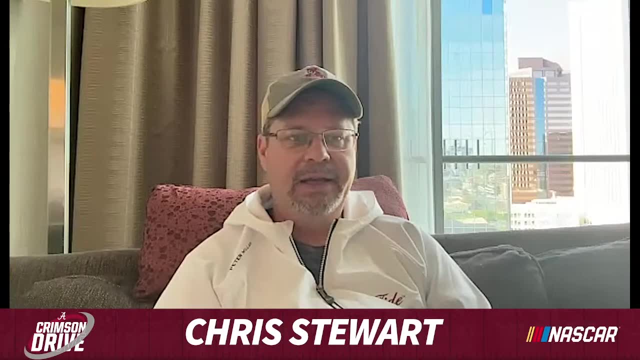 And I think that's a major thing. They continue to be who they are. offensively, Roger, they finally got some things locked in on a consistent basis on the defensive end, And that's what allowed them to get it done against the Heels. 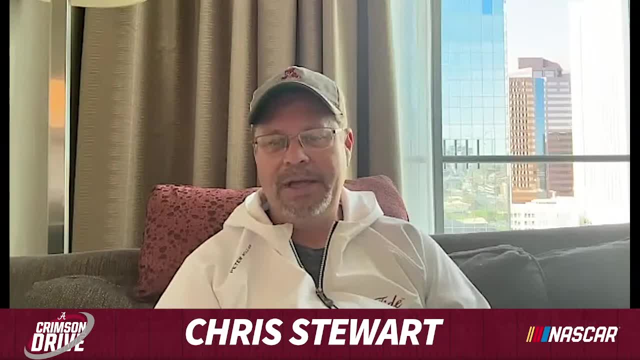 It was really fun to see all of that come together And you know, you knew North Carolina was going to make a push and Bama just continued to answer whenever that occurred and thankfully held them off and got the win. Certainly was great to see Grant Nelson. Great performance in that game. And then Alabama wins to move on to the Elite Eight for only the second time in school history, taking on a Clemson team that Alabama had faced earlier in the season. But, as it turned out, it was a much different result. 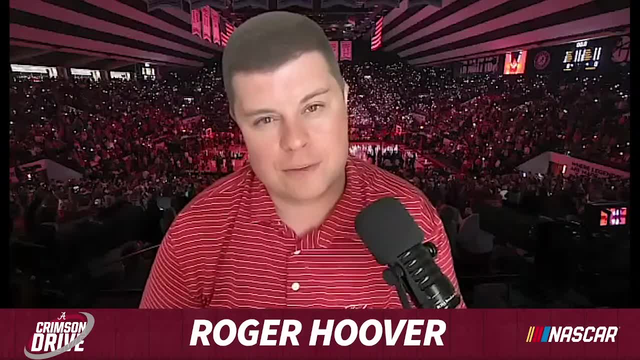 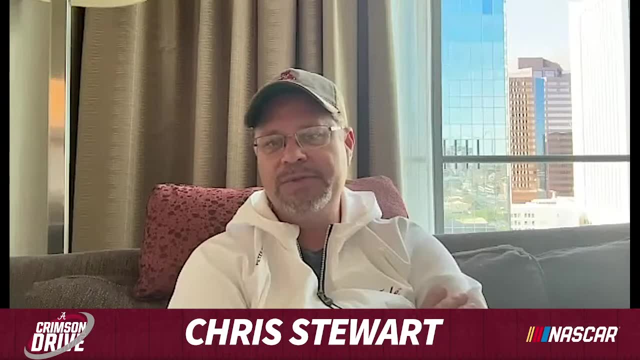 than what we saw in Coleman Coliseum, thankfully, as Alabama reached the Final Four. Yeah, you know, it's kind of odd because even though they lost that game, I think they had a ton of confidence because of the matchup. They knew who they truly were in relation. 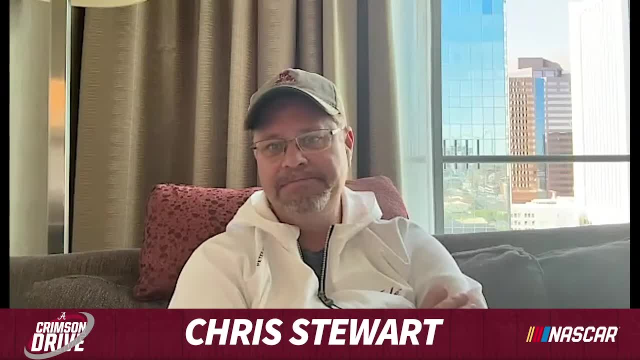 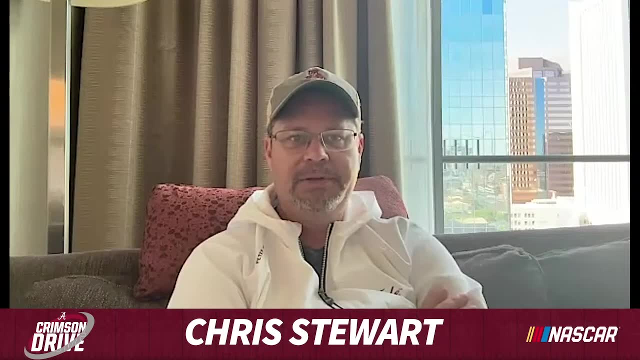 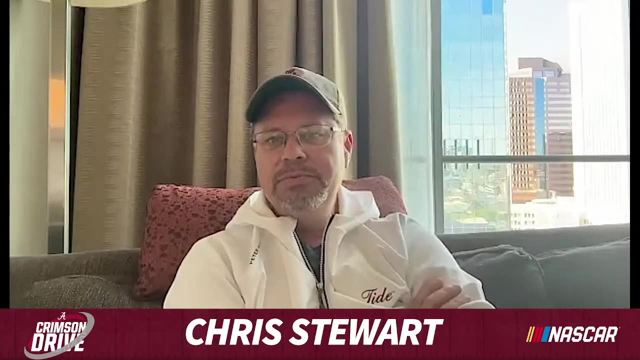 To Clemson. They knew they'd played really bad, frankly, in the game against the Tigers- And that's not taking anything away from their win against Alabama in Tuscaloosa. But at the same time Alabama knew that if they played more to their true identity, 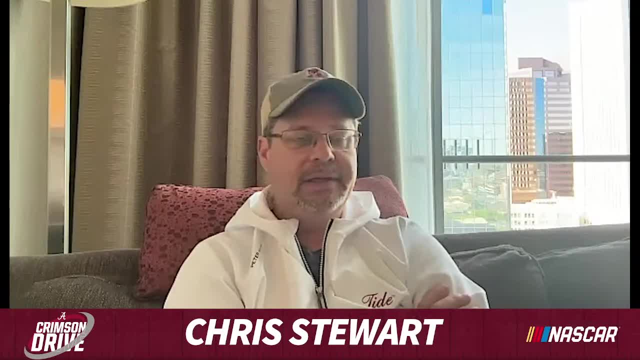 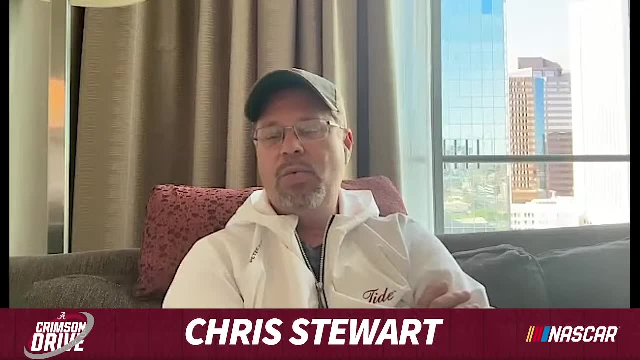 that that would be a different outcome And that's what we got. And it was another one. that was a fight to the end, But so glad to see Alabama play so well down The stretch. defend, continue to make shots- One would make a run. 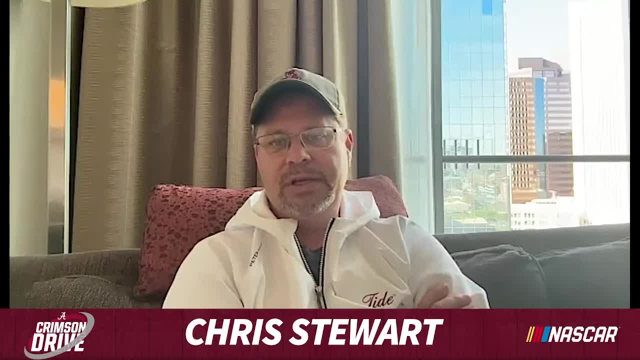 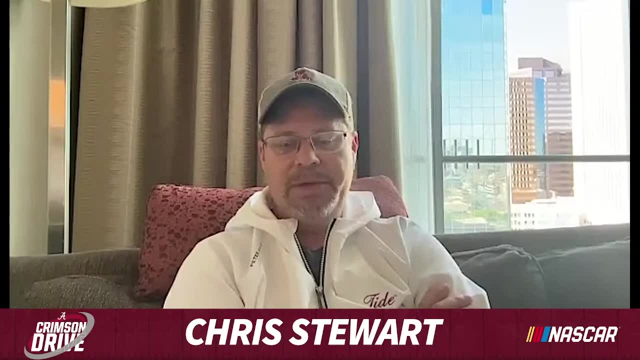 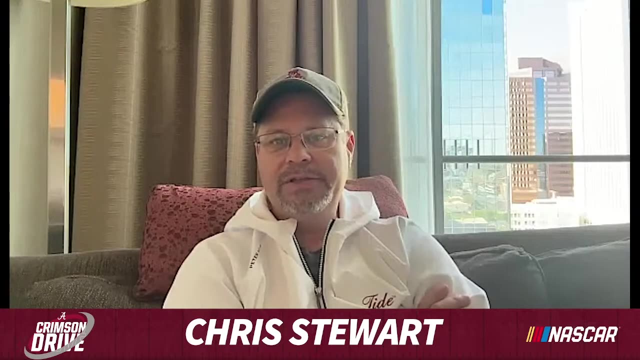 The other would answer back and just continue to keep them at arm's length, Thankfully, and got that special finish. Clemson's a tough team. Very good, PJ Hall. fouling out was obviously big, But the damage had been done, I think, to them before that. 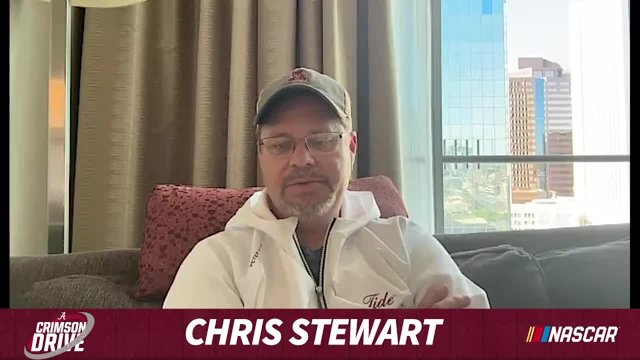 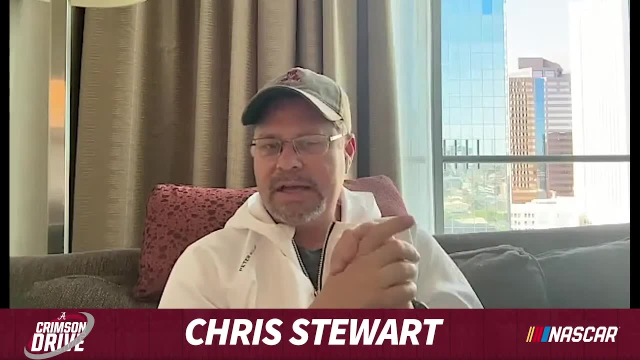 And you know talking with a couple of people tied to the Clemson program at halftime, when they had it at 30. And they were 13 with 758, I think the time left- Whatever the under-eight media timeout was- 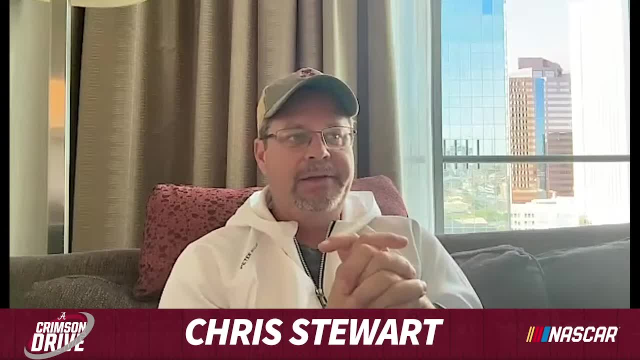 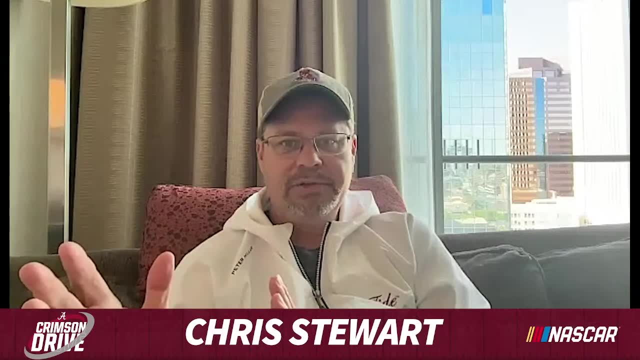 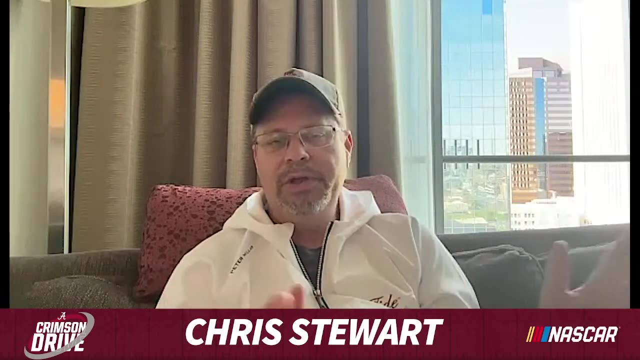 Clemson's got that as a 13-point lead And that's a game where if you let it go five points the wrong direction. that looks so different going into halftime. If you only shave five. okay, it's a very manageable game. 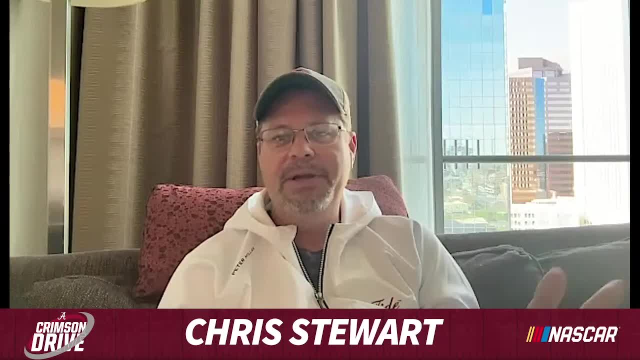 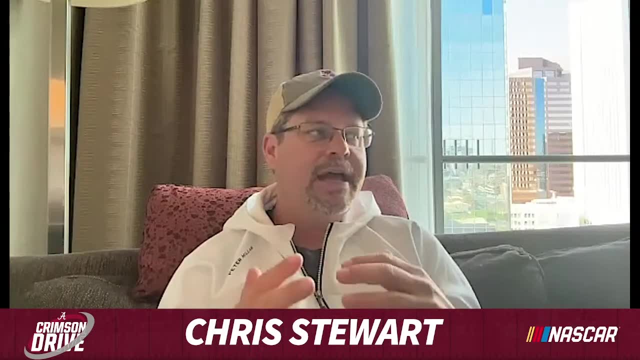 Two Going in, Going into the locker room, down only eight. But instead of it being that, Bama completely flipped it and was up three at halftime And you just had the feeling that, even though we're a long way from the finish line. 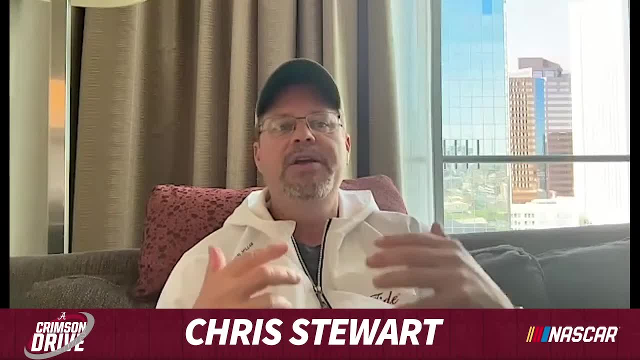 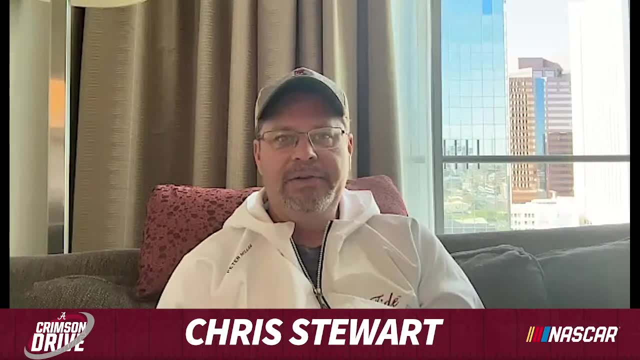 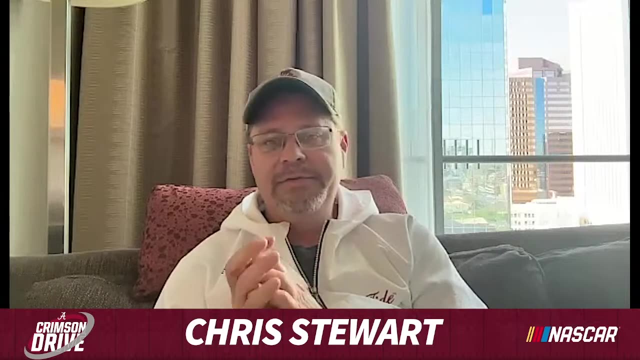 and I think at one point Clemson did take the lead in the second half, you felt like you had taken their best shot, And when you were able to overcome that and just play the game from that point forward, then Bama was going to have. 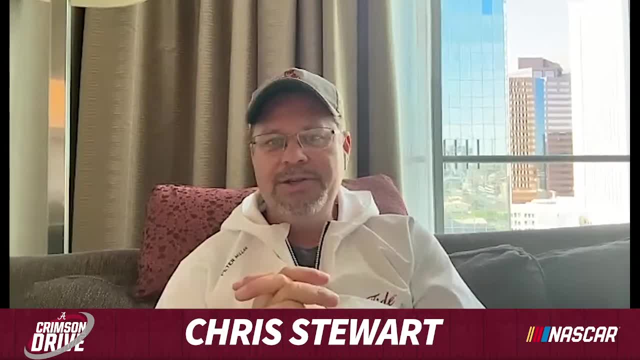 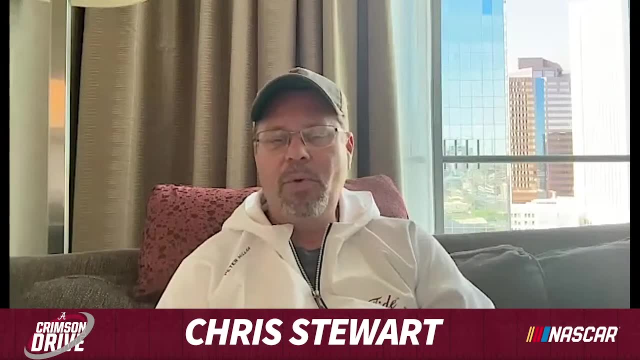 The opportunity to do what they did, And that is not just survive, but advance and move on in this fantastic tournament to a place that they've never been before, which is the Final Four. What did it mean to you to get to say that on the radio? 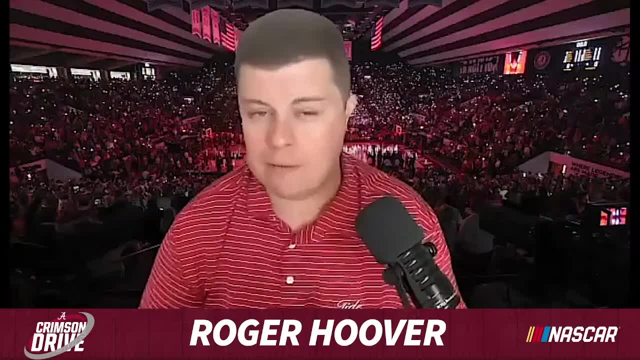 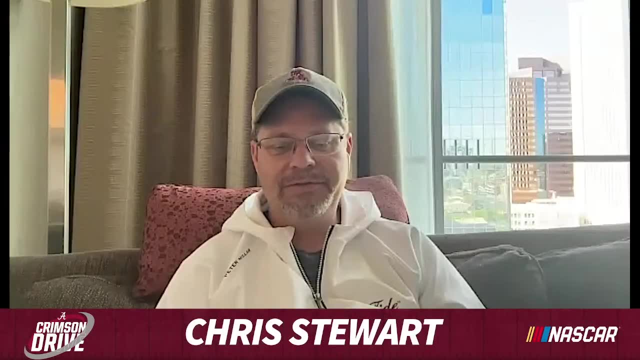 Alabama's going to the Final Four. You've had some great final calls in football, obviously men's basketball through the 20-plus years as well, But this one certainly is different. Yeah, it's very different. I've done a college basketball Final Four. 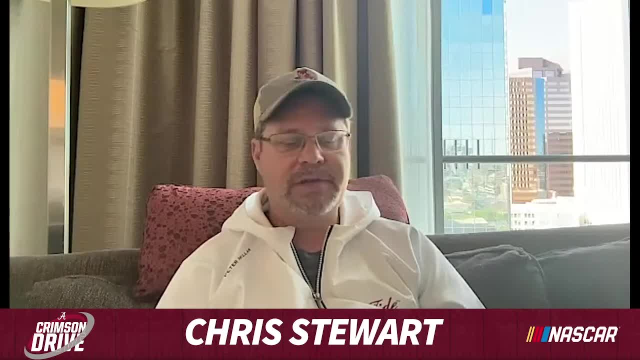 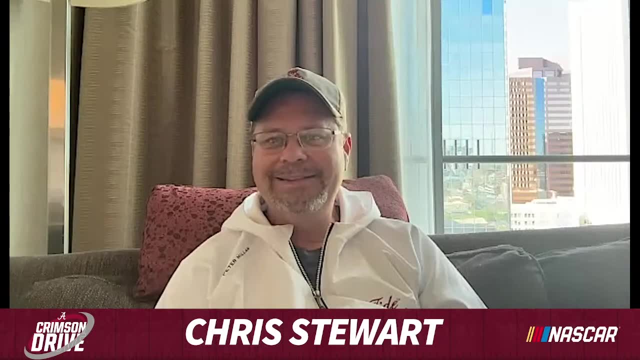 And even a national championship win. before You know I've talked about this, probably before you were born or a toddler. I did Birmingham Southern back in 1995 when they won the NAIA National Championship. Different stage, different level, But if you don't think, an NAIA title means something. 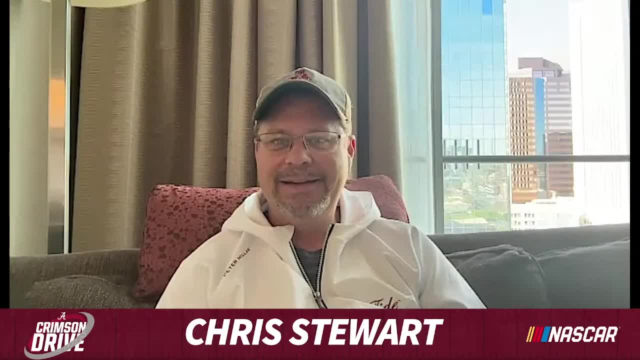 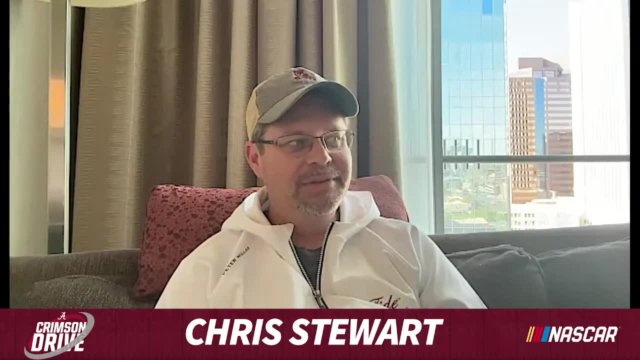 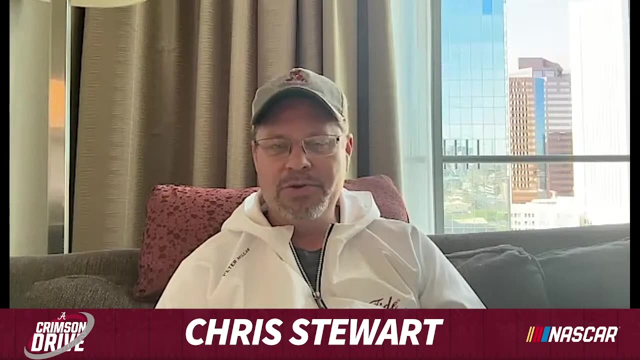 go on over to the football building and ask Kalen DeBoer if it does, because he's got three. He's got three NAIA championship rings himself, And you know that's an accomplishment, That's a big accomplishment. But the setting, the venue, the environment, the exposure for it, it's just so different. 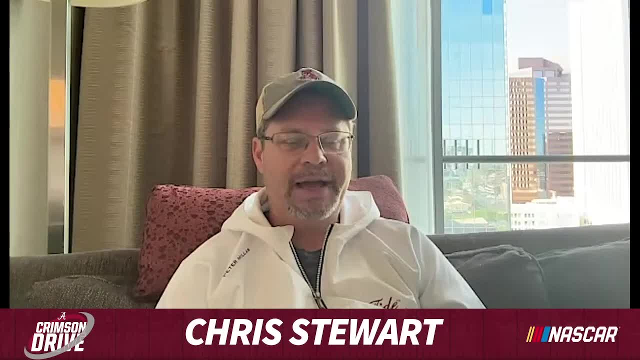 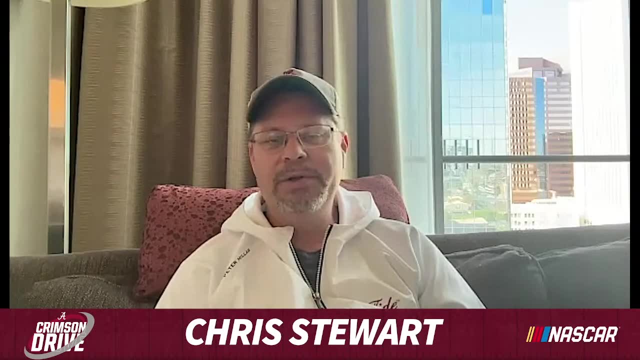 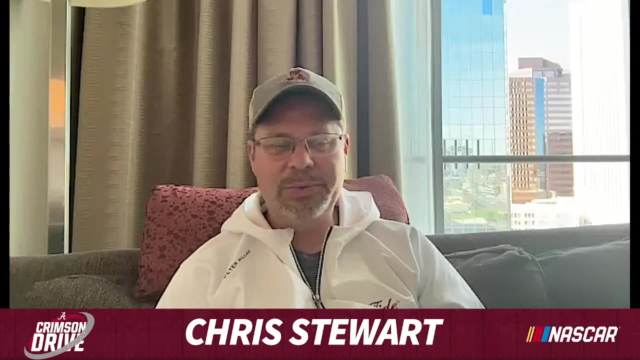 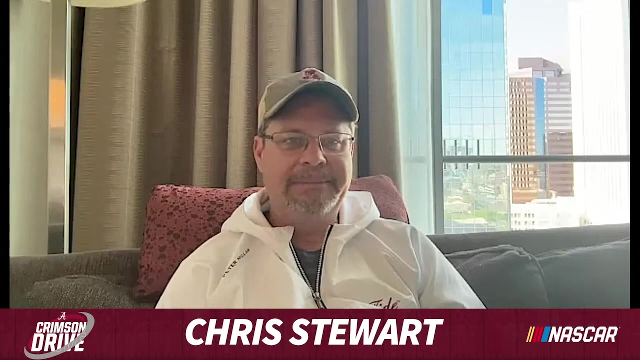 So to have the privilege of broadcasting this for Alabama Also, that was very early in my career, Even though it's different when you are a part of a championship and it happens in your first or second year of doing play-by-play. you appreciate it, but you don't at the level that you do now. 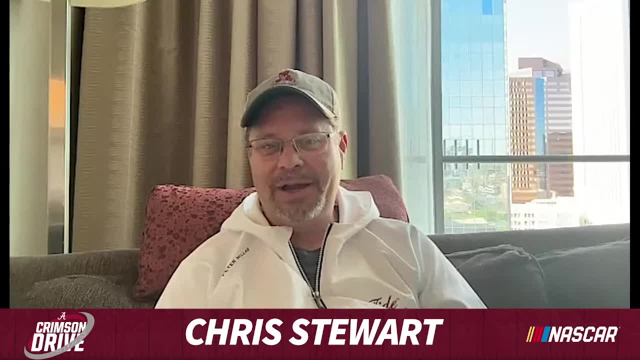 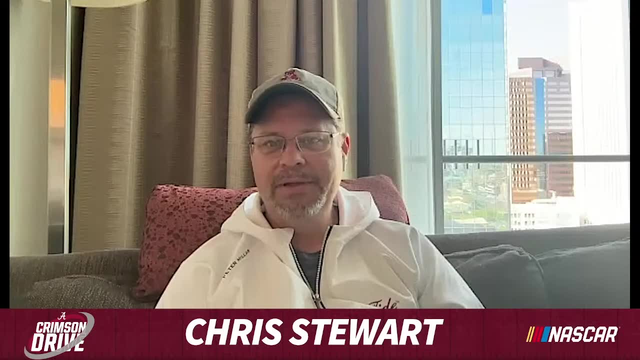 certainly 22 years into being the basketball announcer, like I am in Tuscaloosa, and 24, 25 years, whatever it is, of being a part of Alabama broadcast. But then on top of that, as you and I have talked about too, Roger, 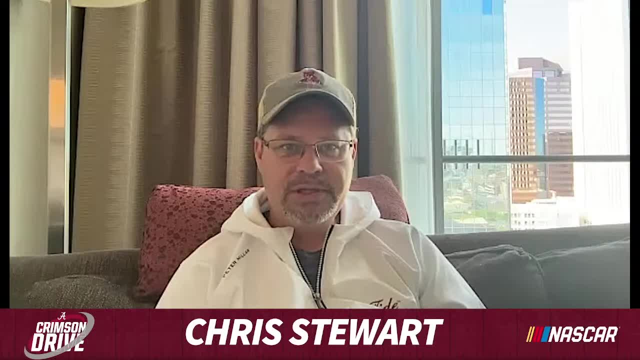 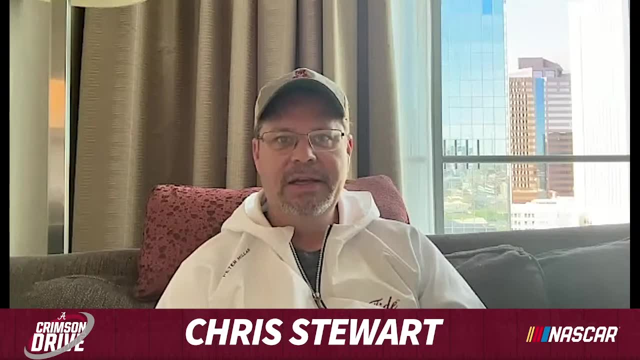 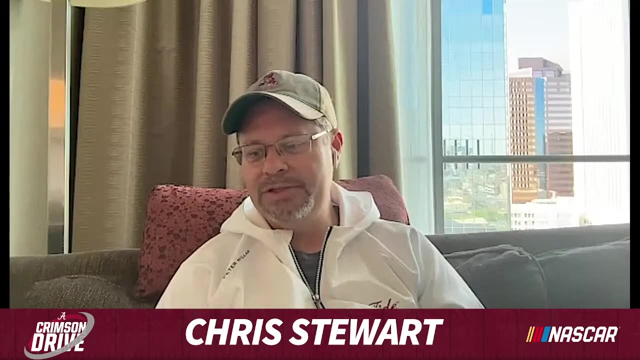 I've been a fan since I was a kid, And so to see this Happened to have. you know, I was a kid in the stands at the BJCC when Derek McKee, Mark Godfrey, Terry Conner and Jim Farmer 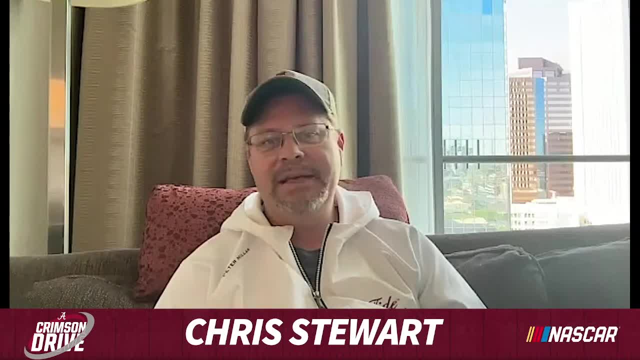 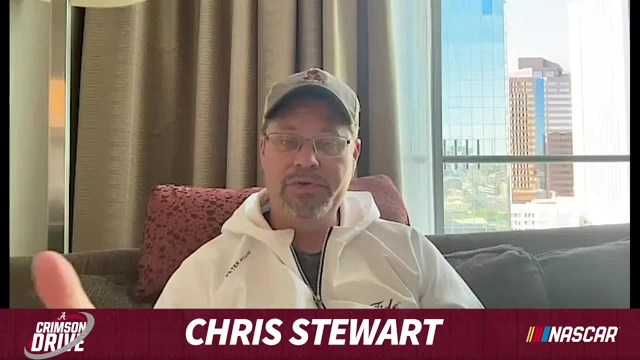 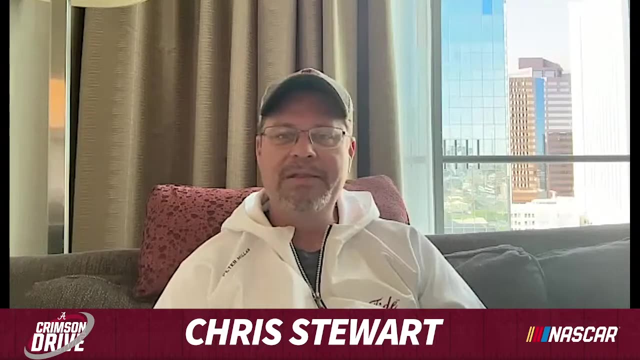 and I'm leaving out some really good players. But I mean when that team in 87 played in Birmingham in the first two rounds in advance to go to Louisville for the Sweet 16 and lost to that Providence squad with three- Tino was the head coach and Billy the Kid Donovan. 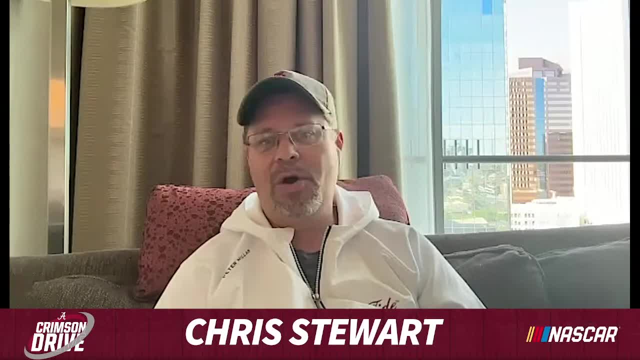 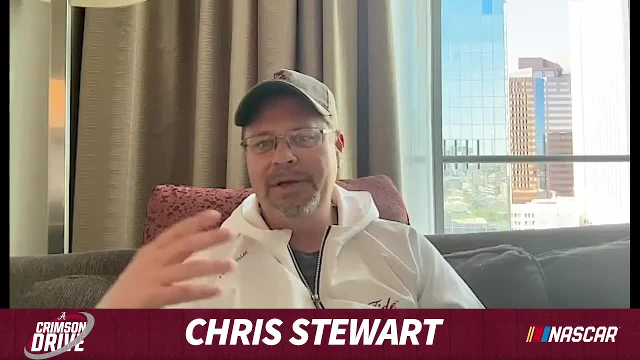 as the sharpshooter with Delray Brooks. That was a heartbreaker. Bamble was a two seed and thought that was going to be the team that was going to get over the hump and go to be the first in the Elite Eight and maybe win the whole thing. 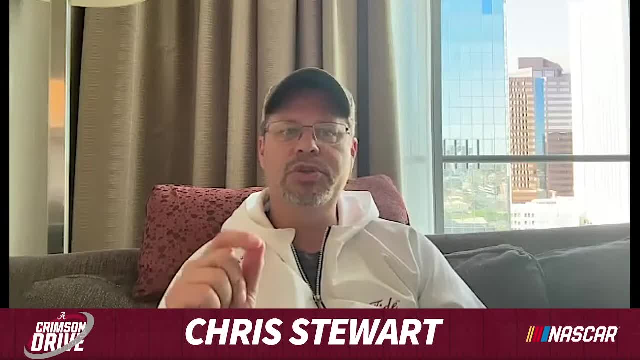 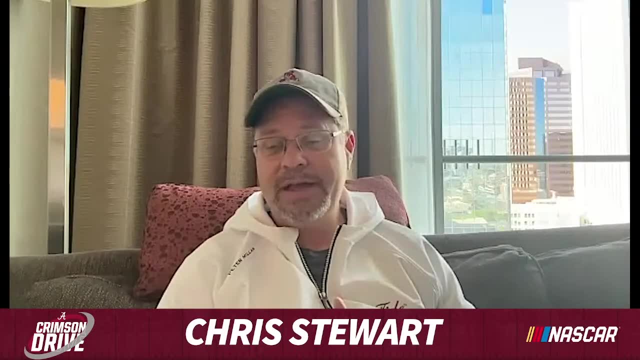 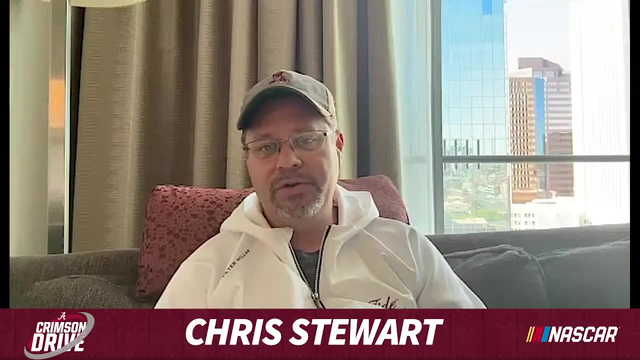 And it was one of several teams. frankly, Roger, that was good enough to win it all if they could have gotten past a hurdle, And the most recent being last year, if that team beat San Diego State, then that team obviously is one that I think very easily could have won. 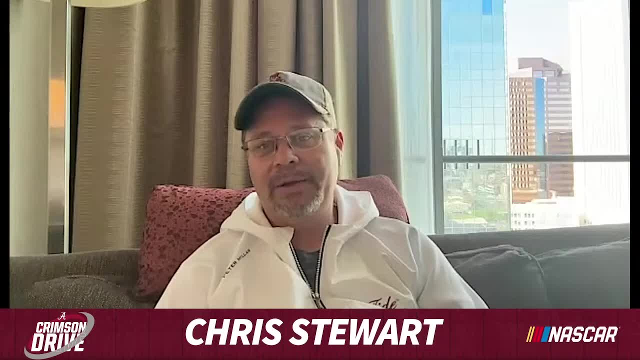 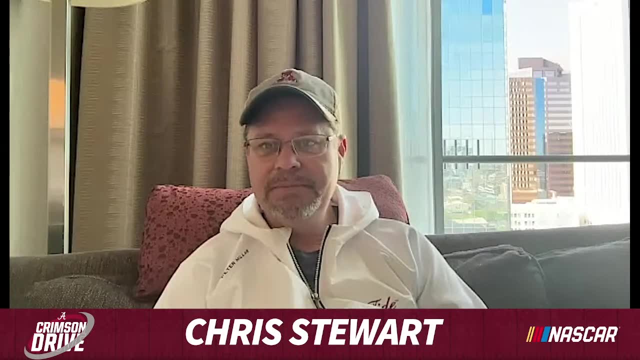 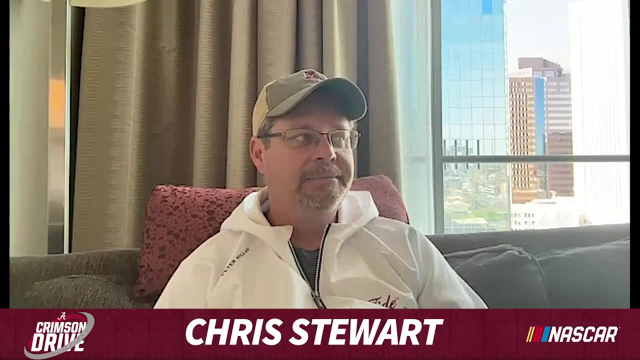 the whole shebang and nobody would have been shot by it. They were the number one national seed going into the tournament. This one has come out of the blue to some, but not to me. I felt all along that this would be a better team now than at any point. 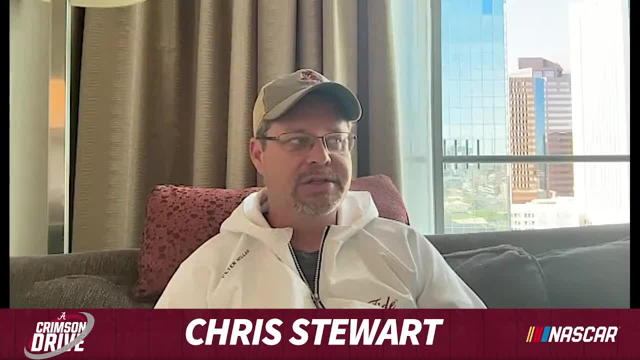 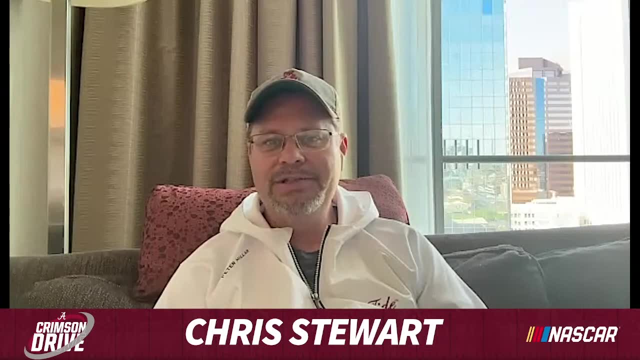 And that has played out that way And just excited to see. I think they'll have the chance to be in the position they're in And hopefully they're not done. Hopefully it's got two more wins And we will have one heck of an A day next weekend with a new coach. 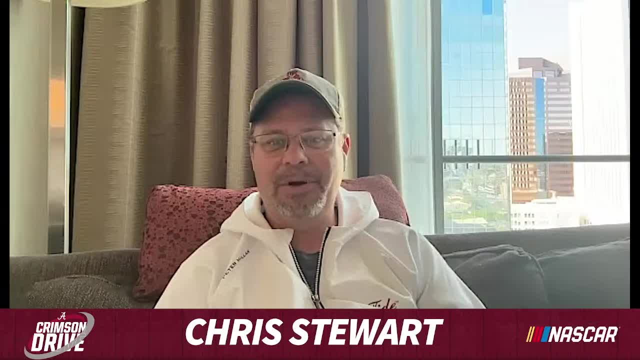 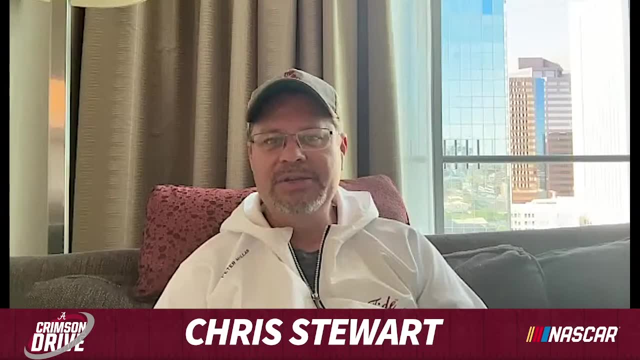 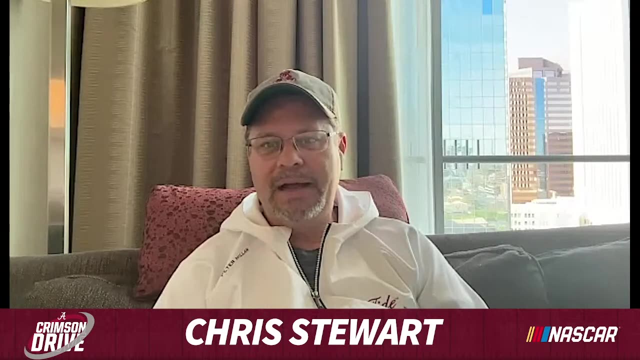 a new basketball trophy in town and a lot of things to celebrate, But it's a really cool time And it's an important time. The ceiling has been broken And now Alabama, Alabama, basketball, I think- well, I don't think this is the only- 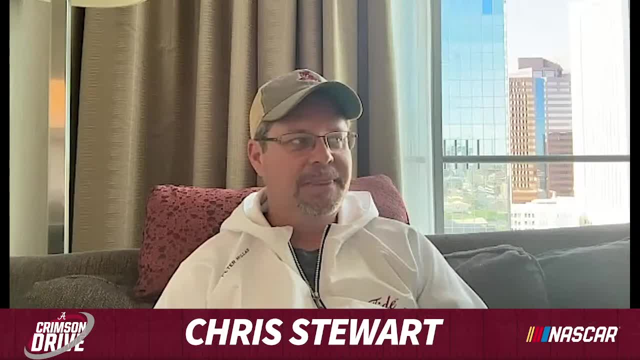 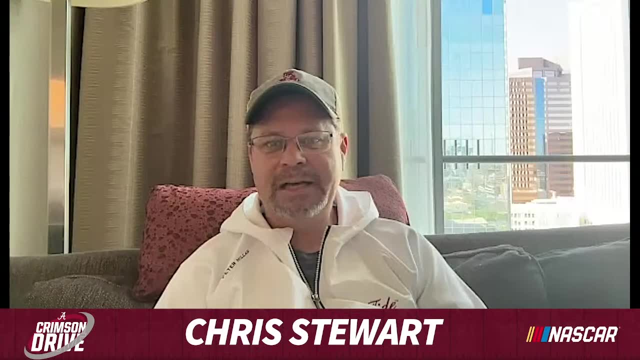 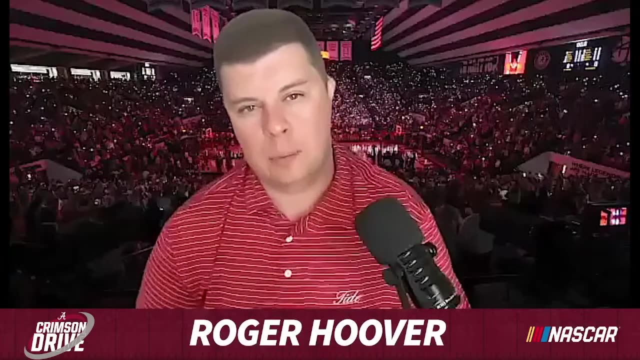 I think this is the first of multiple Final Fours that will occur with Nate Oates as the head basketball coach. I don't think he plans to take the foot off the gas anytime soon. Certainly hope not. So again, a great moment for you getting to say you know. 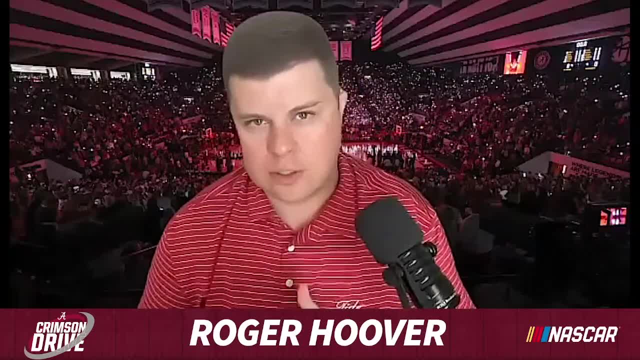 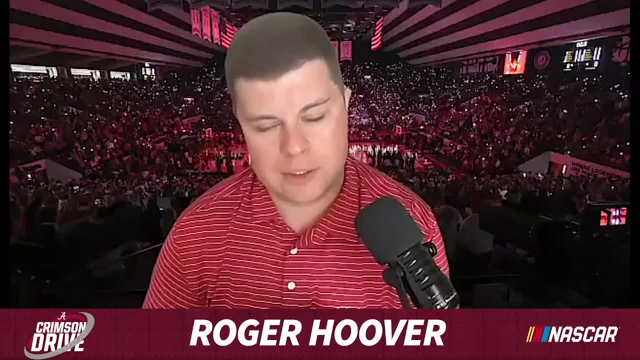 Alabama is rolling to the Final Four And I know you don't want to talk about yourself too much, but this is the Crimson Tide SportsCenter. I've got to ask this because we all know your story well. here We've got to document the health struggles you went through a few years ago. 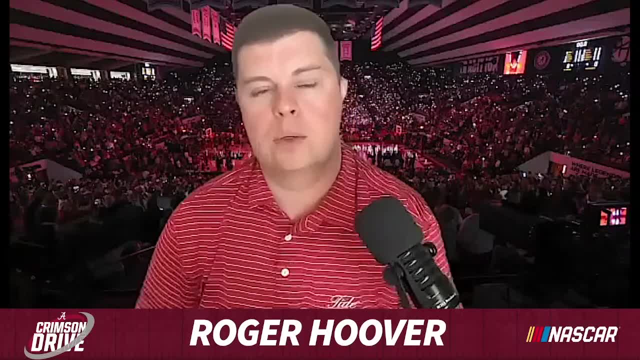 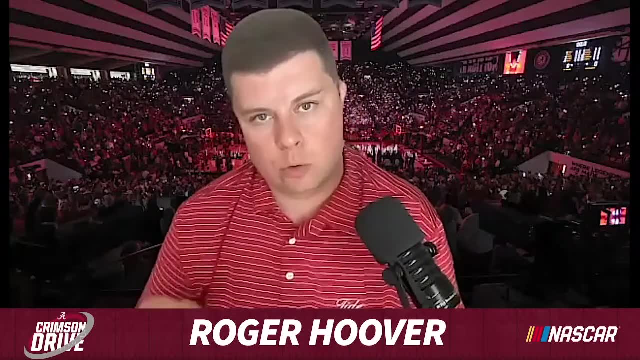 The national stage was introduced to that over the weekend with an excellent feature by the Turner Sports pregame show getting ready for Alabama's Elite Eight game. Just what did it mean to you to have your story kind of told again to a national audience and then the feedback you've received since then. 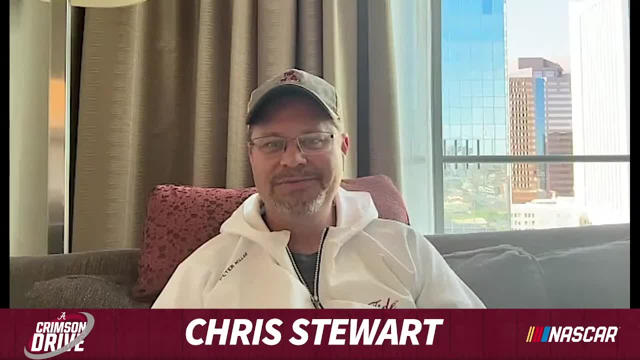 It was among the many other things, Roger, that have been about this. It was surreal because I'm literally standing in my hotel room getting ready and I'm watching national TV and there's a feature being produced about me And then, when it's over, there's Ernie and Charles and 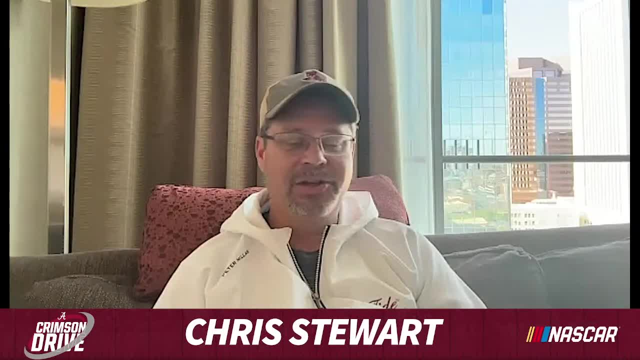 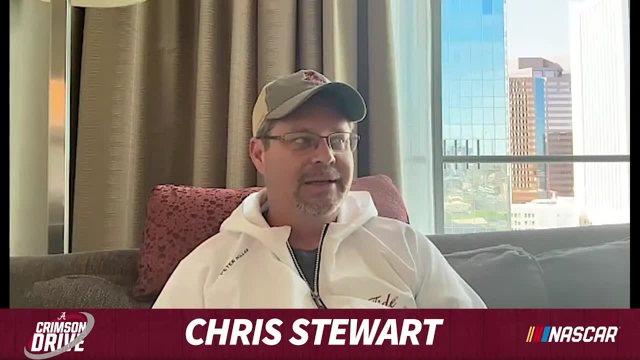 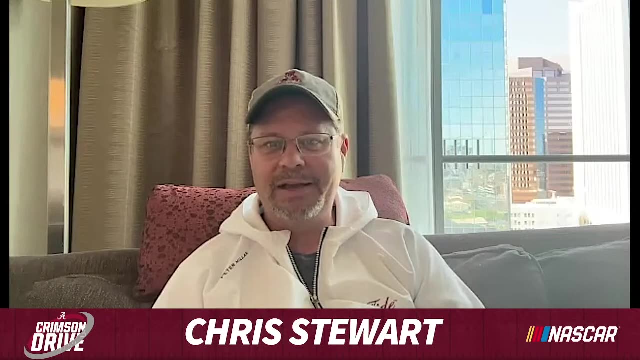 and and Kenny and Clark all talking about me. It was kind of weird, to be quite honest, but it was extremely kind. And then I, you know, was sent the clip later on. I was on the phone with the guys at the end of the show. 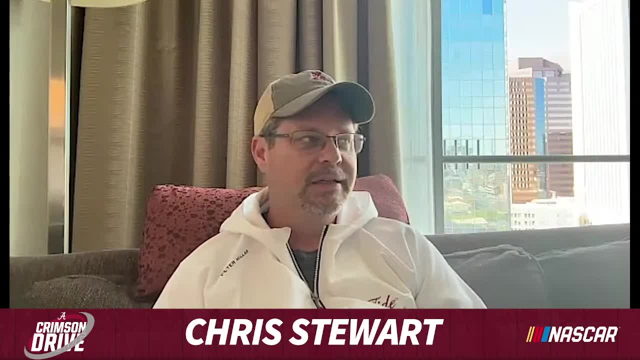 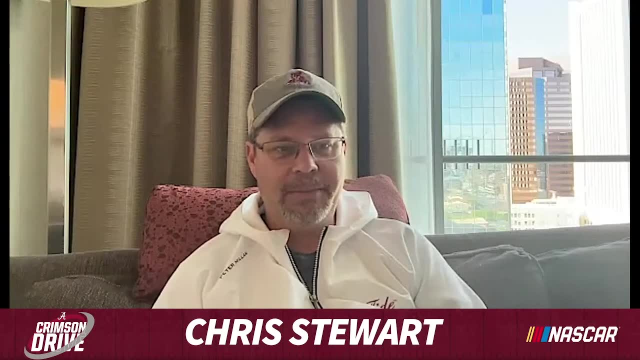 I was on the phone with the guys at the end of what they did at the end of their broadcast night of playing the call at the end And I'm grateful The story's able to be told because I understand that I'm the face for the. 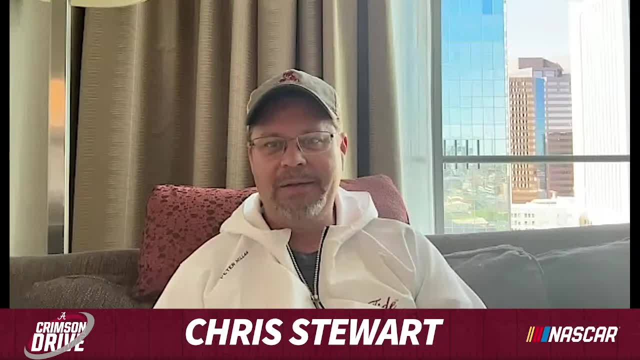 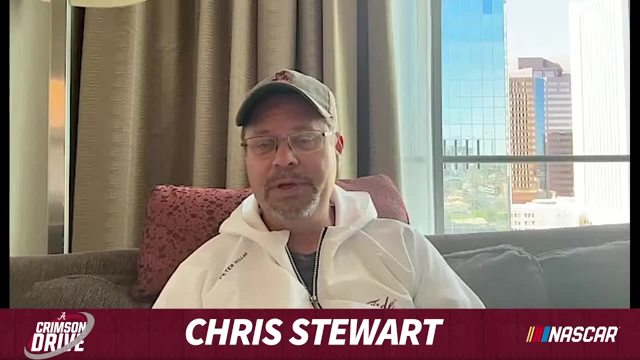 story. but the story is not about me. The story is about medical people that saved my life, that helped me get back to where I can do this. Friends, like I said, I'm grateful, Like yourself, who who helped me tremendously when I needed the help. you. 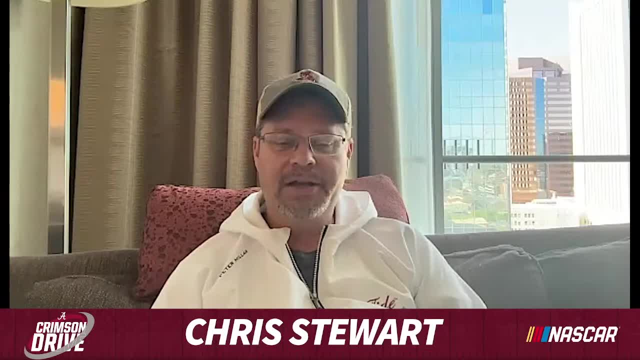 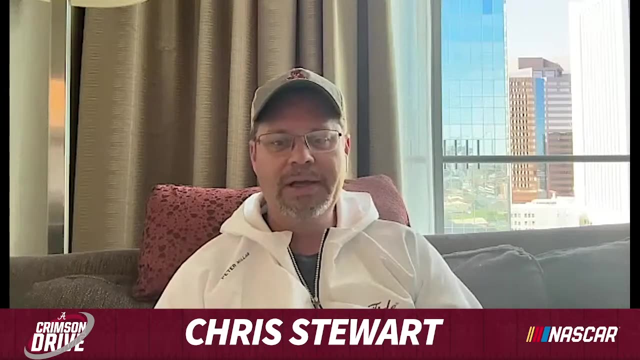 pitched in in a massive way, and not just the bridge leading up to me doing, coming back and doing games, but you literally were there to help and assist as I was getting stronger and able to to take on more of my regular responsibility for it. 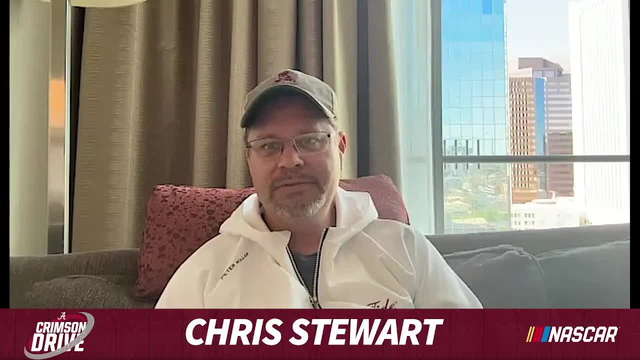 I've said it most, you know many times, but most of all, just my personal belief that it's a miracle that God did in my life and it's not none of it happens without his blessing and his favor. It's not something I deserve. 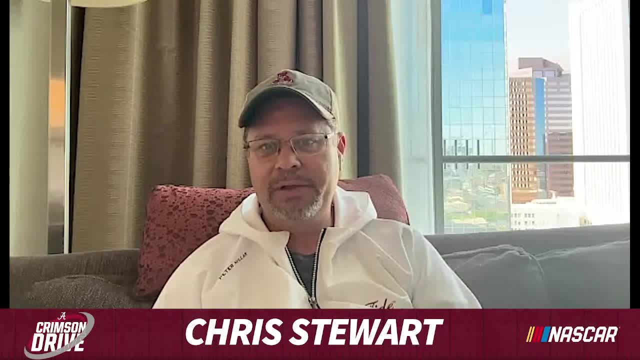 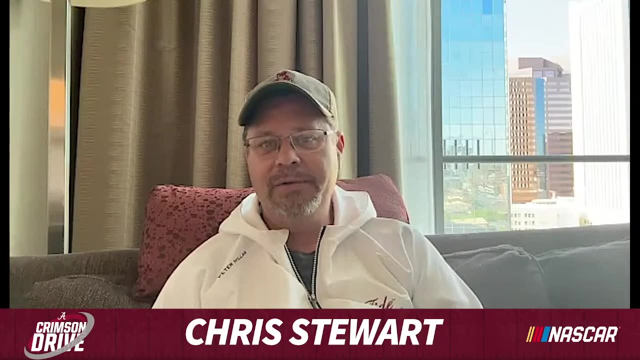 It's not something I've earned, but it's something that he blessed me with and I will forever be grateful for it. And I've. you know I don't try to beat anybody up with it, wear anybody out, but I have a responsibility to share where I think it came from. 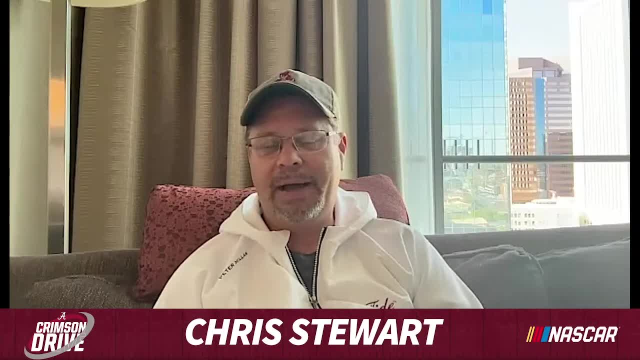 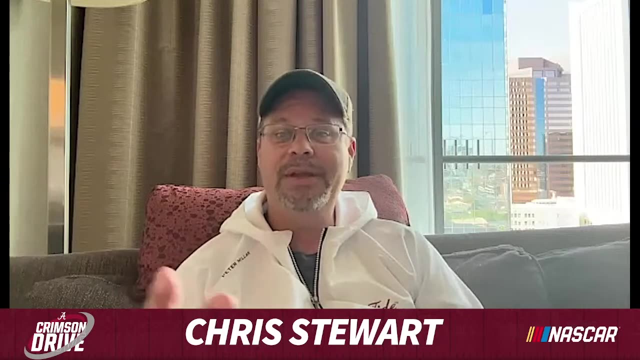 And why I'm able to do what I'm doing now, And I am appreciative that that Ernie, and actually an Alabama alum who produced it, Khalil Cage, who you won't hear her name, You won't see her, but was actually a member of Crimson Cabaret. 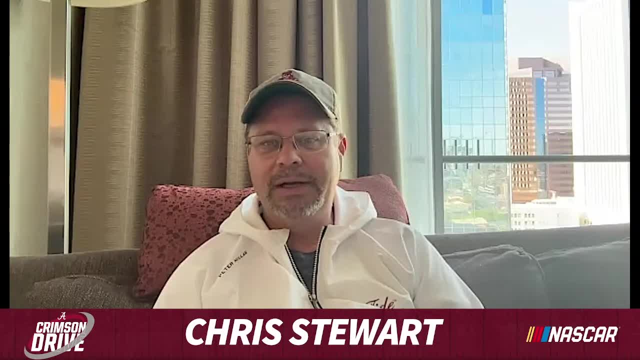 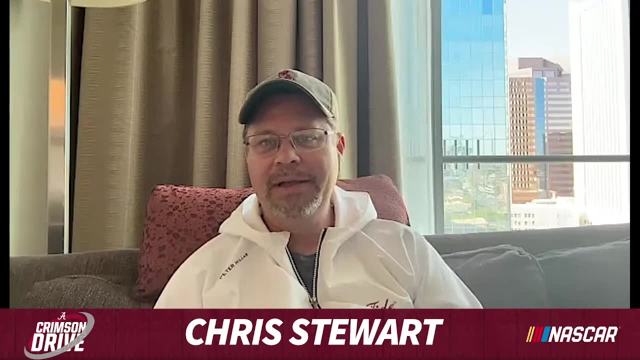 probably 15, 20 years ago, when that- that's where I'm better. She's married to Greg Cage. She played basketball in Alabama and she- she came up to me when we were at USC at shoot around one day and she goes. I want to tell your story in a feature. 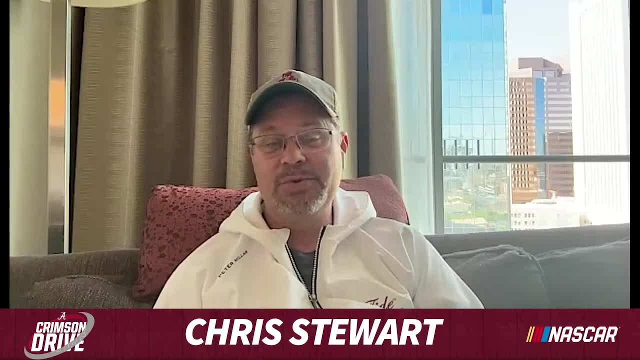 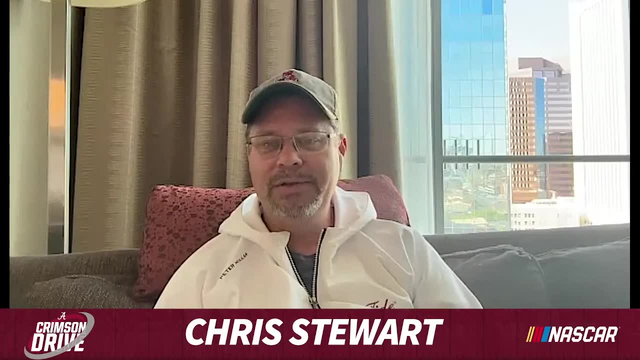 I don't know if it'll ever air because this was before the North Carolina game. She goes. we want to do this And in case Alabama wins and we can, we can run it before the elite eight game, but I want to produce it and have it ready just in case. 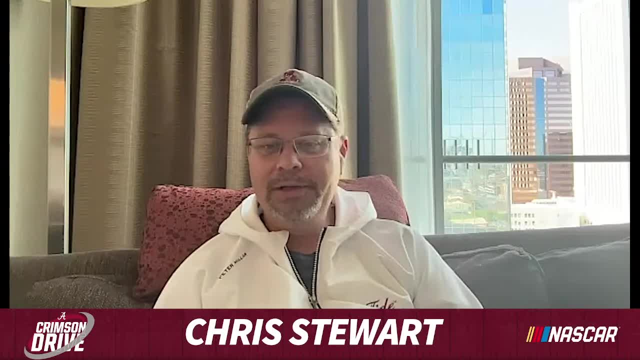 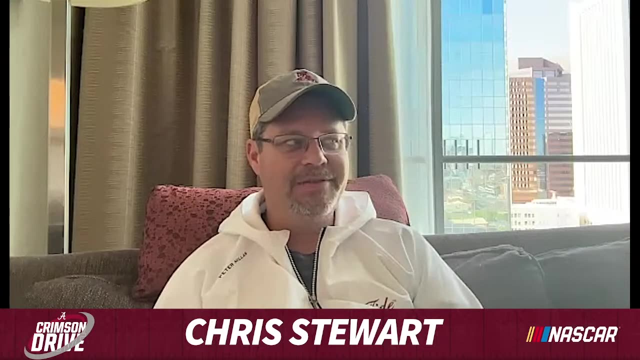 So I was grateful that the tide won, that it went up on the cutting room floor and the players were who weren't around and didn't know the story, were incredibly gracious. One of the most slap me in the face moments about how incredible our team is. 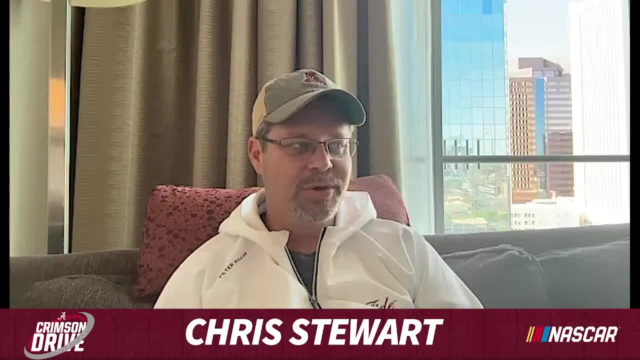 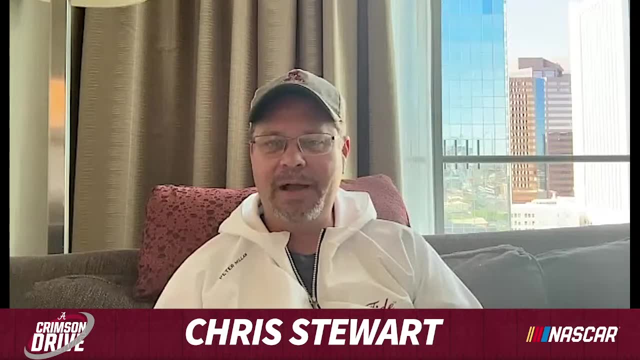 and our kids are, was when Riley Griffin comes over to do the post game interview after the elite eight win And I'm there asking him about going to the final four And he said: well, we all saw on social media the feature before it ran on television and we sent it around in the team. 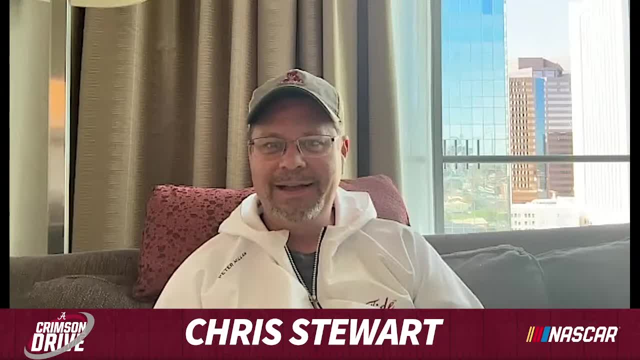 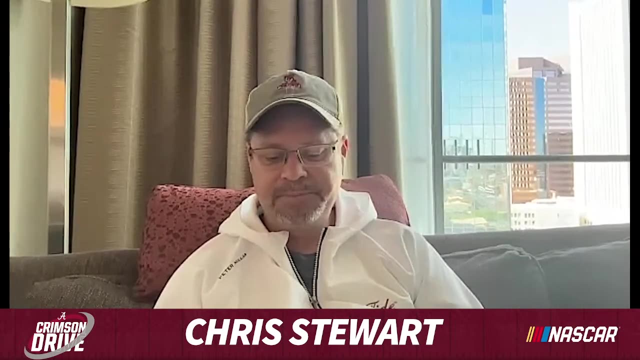 chat and said we got to win this for Chris And that was. that was very humbling And I'm so grateful that everybody has been as kind as they are. I just hope that people understand. it's nothing really that I've done. 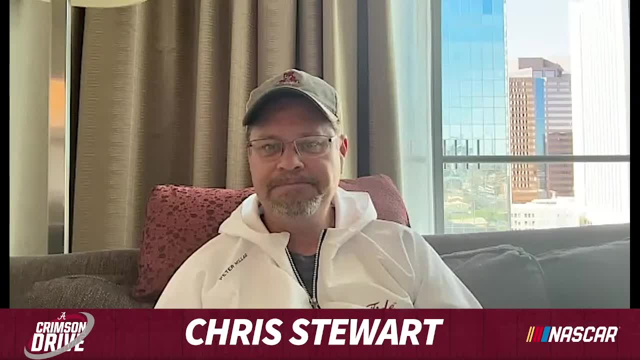 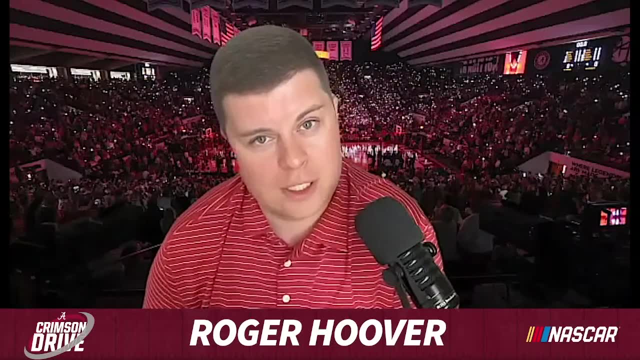 I've done, I've done. I just know how fortunate and how blessed I am. We're extremely grateful for that as well. Moving forward, And again you're in Phoenix getting ready for these games coming up this weekend. It's got to start with another tough challenge with the Yukon Huskies. 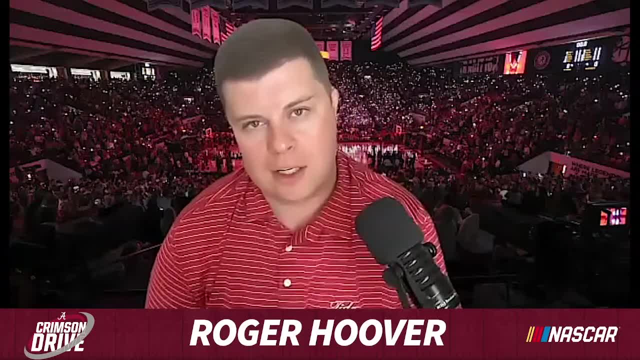 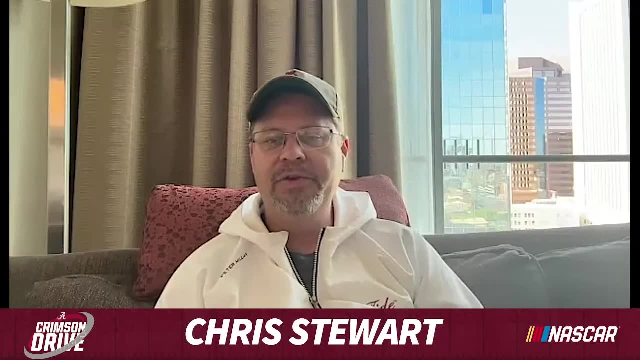 Just what's going to be most important for this Alabama team: getting off to the right kind of start against Yukon on Saturday. Roger, I don't think Alabama has to be anything other than what they've been this year, when they've been at their best. 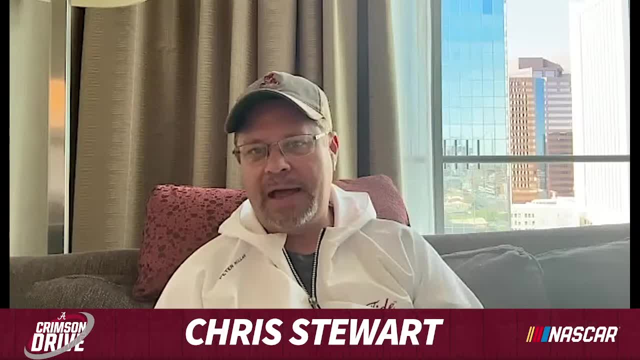 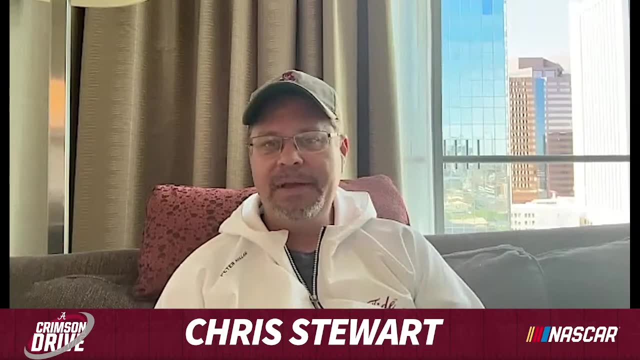 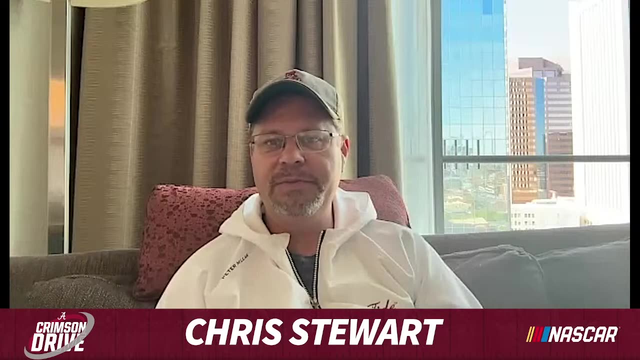 Uh, I don't think they have to play the game of their lives, Um, I just think they have to continue to be who they've been, but they can't be average or below and expect to get to Monday night. They've. they've got to be the best version of themselves, and what? 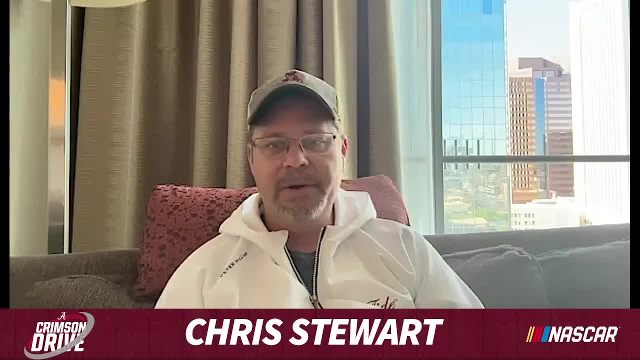 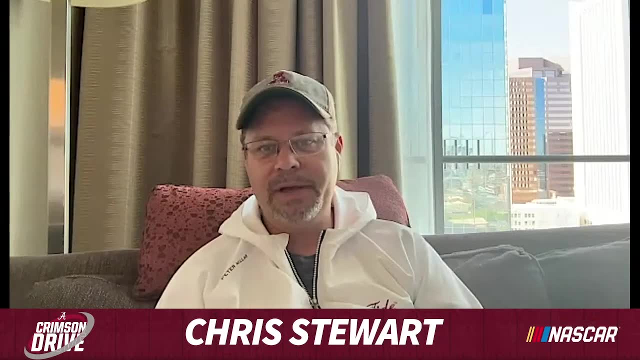 we've already seen from them. It's not going to take a miracle. It's going to take 40 minutes, Um, but if you slack off any, it's, it's not 20. Minutes is Illinois found out because they played really well for about 20. 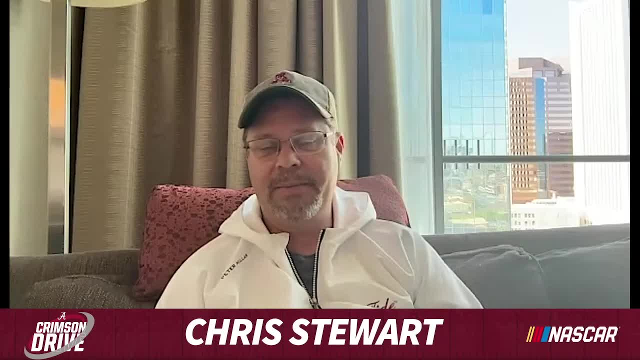 minutes. It was a five point game And the next thing they know they come out of the locker room and they were just hammered a 30, 30 run. We'll get you beat if you're on the wrong side of it. 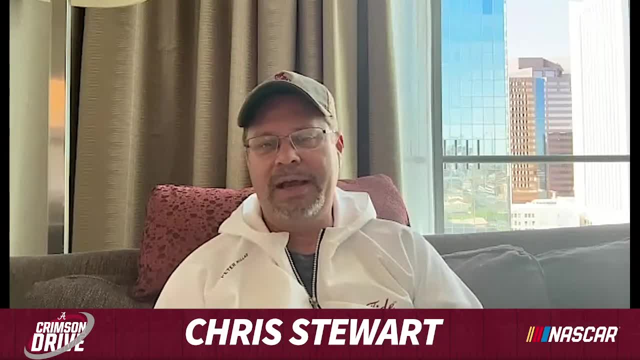 And that's exactly what happened. And you know you can't have any lapses. You've got to find a way. You've got to find a way to make sure that you are still in that game at the under four media timeout. 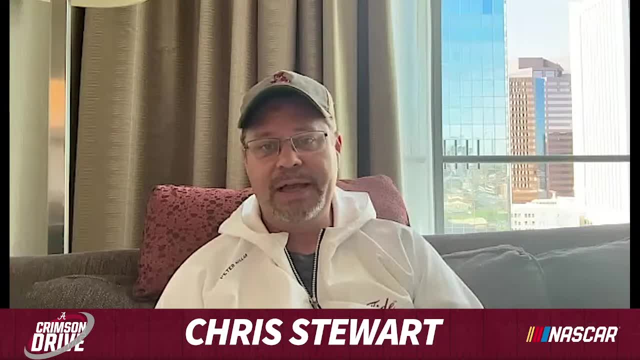 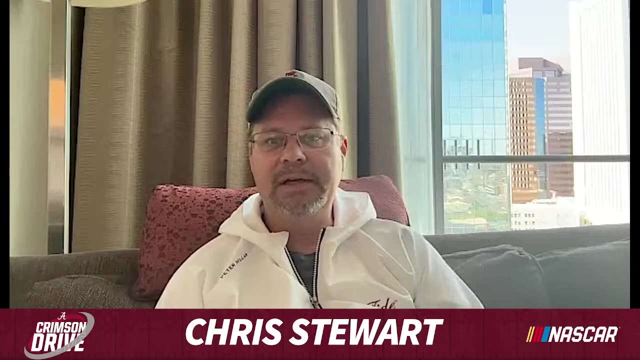 And, uh, they have lost this year. They've lost three games, Uh, and they are beatable and Alabama, at its best, can beat anybody. They have said that and believed it all year. We have seen that, Uh, but it will take in order to cut down the nets on Monday. 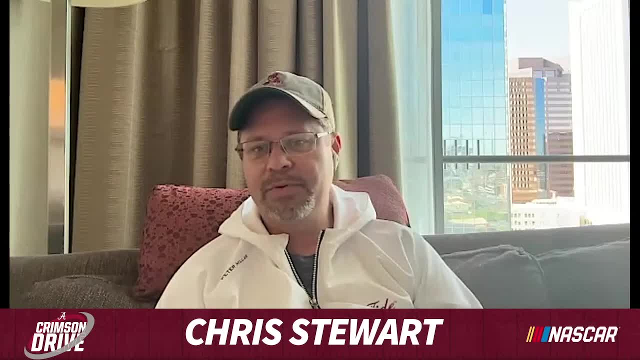 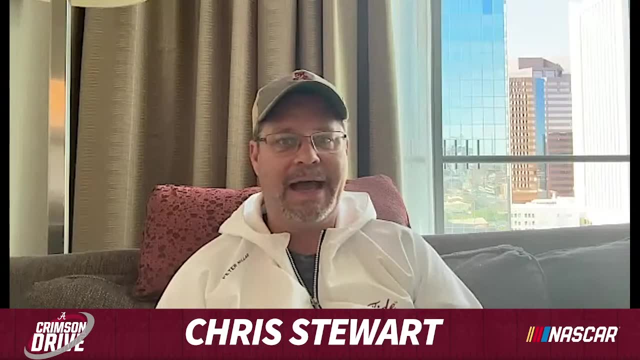 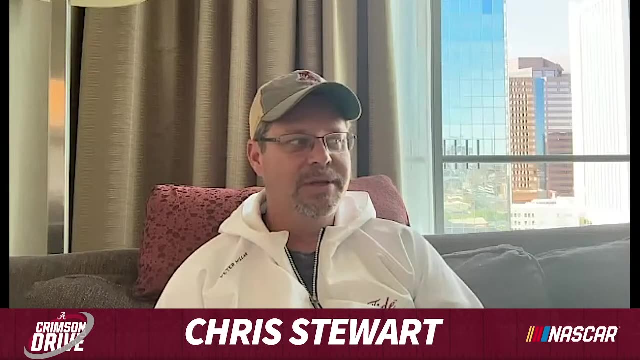 it will take two fantastic performances um against two tremendous teams. whether it's you can on Saturday and either NC state who's been a great story themselves, or or Purdue. you know this, this could be the retribution tour for Alabama. 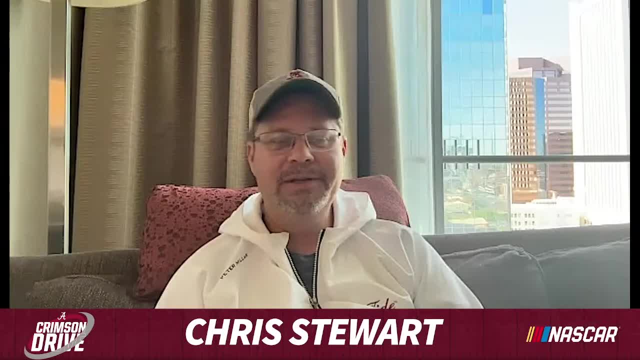 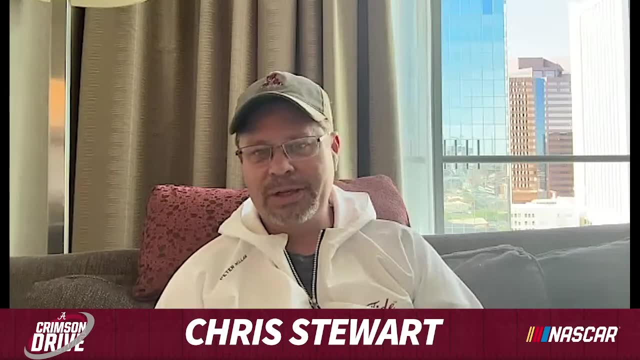 Uh, you know you, you beat Clemson, Who's already beaten you. You beat UConn, that beat you 20 years ago, And then you, uh, would potentially play a Purdue team that beat you earlier in this year. I will say: Purdue has not beaten Alabama in the United States of America. 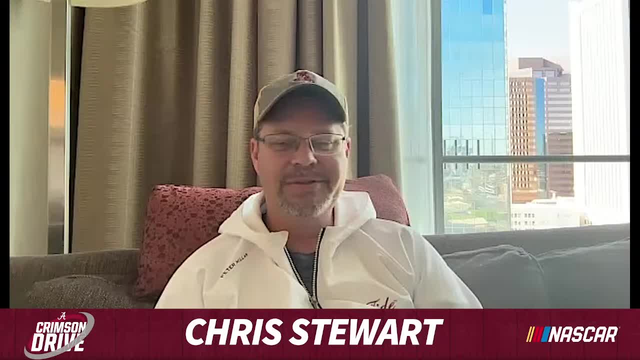 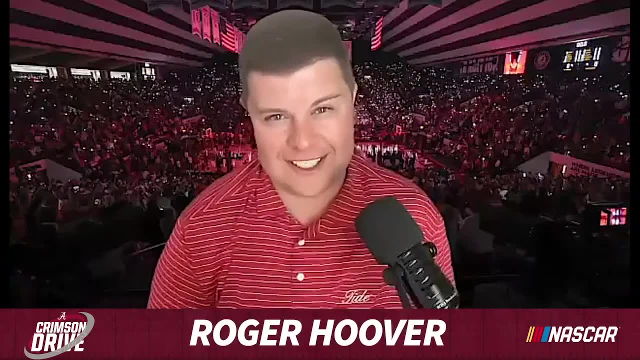 though by golly we're undefeated. Uh, we're undefeated on this side of the border, So hopefully we'll get another shot out of it and get it taken care of. Yeah, I'm hoping you get the chance to see Zach Eady in person coming up on Monday. 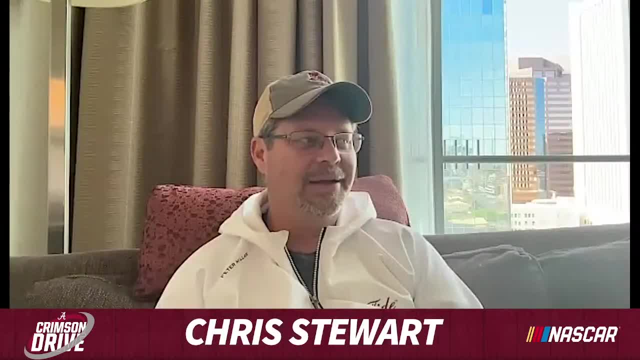 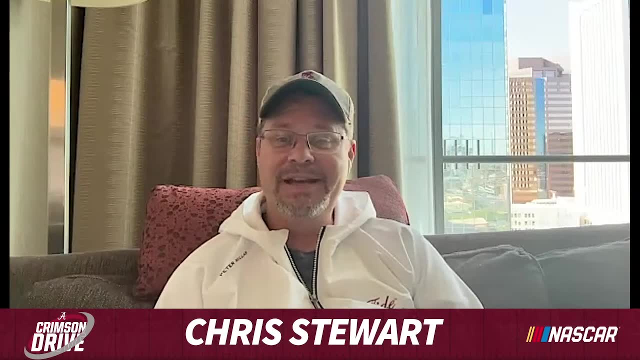 If it shakes out that way, I would- uh, look, I'm not going to lie to you. as long as Bama's playing, it doesn't matter tremendously, but I hope it's that big fellow for NC state instead of that big fellow for. 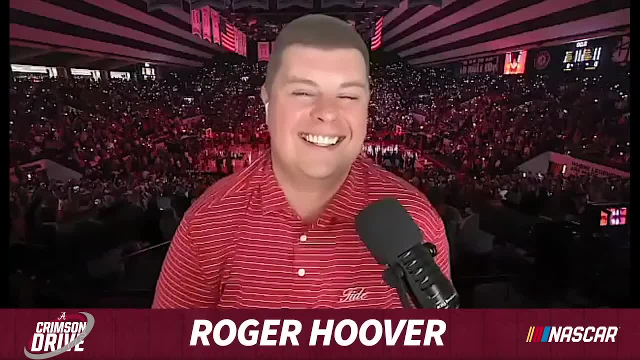 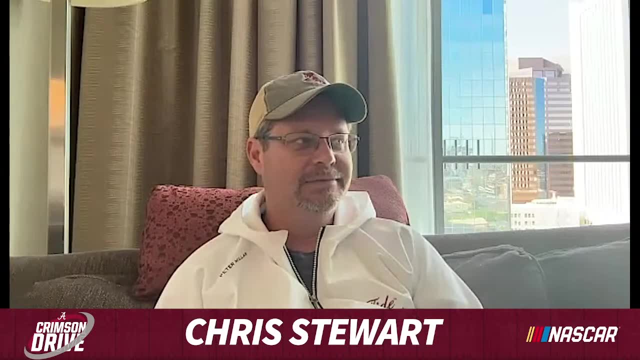 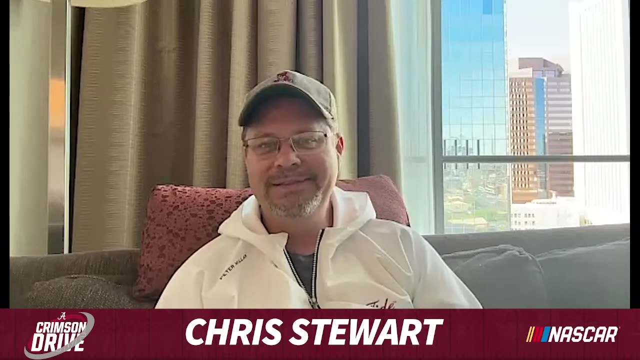 Purdue. I may come to regret that if it happens, but no, they um anybody that's here. this point can win it clearly And it's special, I think there are two underdogs. There's clearly um two teams that everybody's expecting to see play on Monday night. 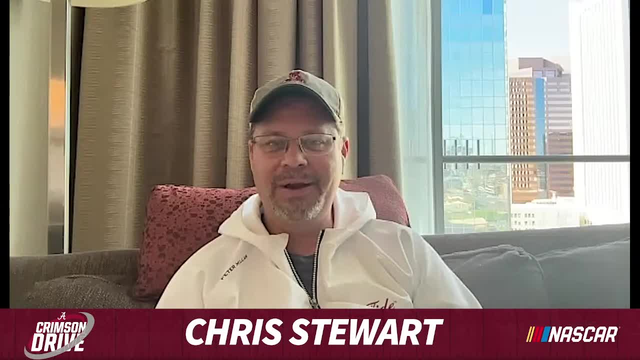 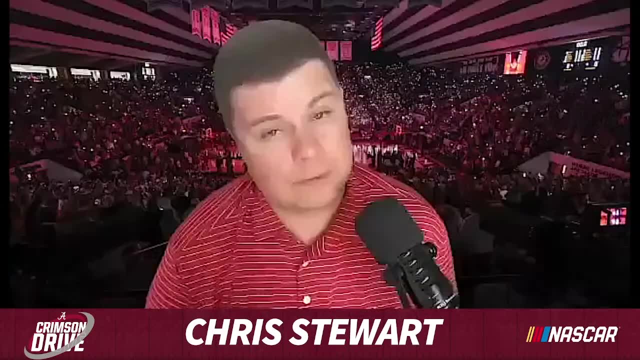 but I've got a feeling that NC state and Alabama don't really care about how the script has been written by by many. They're here to kind of write their own. We look forward to it. Well, Chris, you, Brian and Tom have a blast coming up in Phoenix. 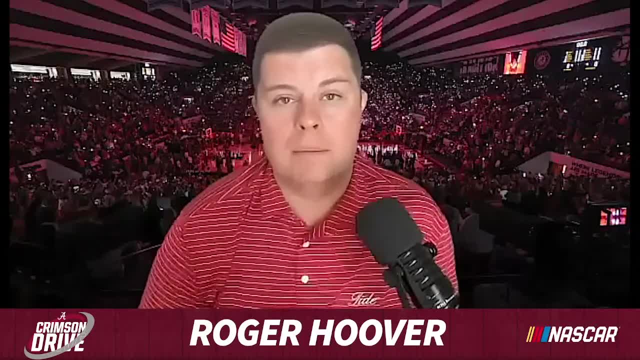 We can't wait for the broadcast coming up On Saturday and then hopefully on Monday night And, like you said, uh, right after that, uh, we'll be talking football, getting ready for a day coming up on April 13th. 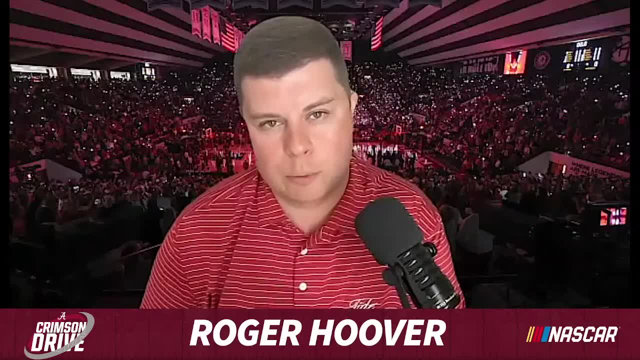 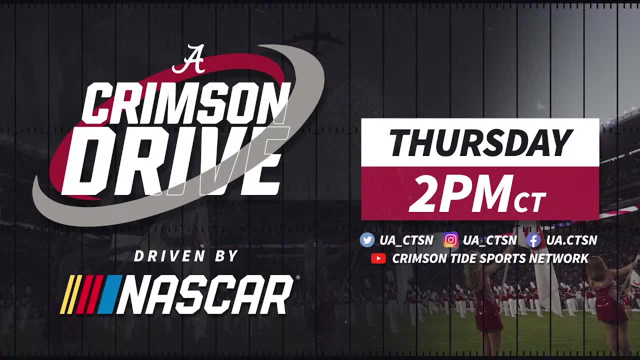 but just all the best that's coming up for you and the Crimson Tide sports network moving forward. Thank you for your time with us today. Roll tide, Roll time buddy. Thanks so much. There is nothing like sweet home, Talladega. 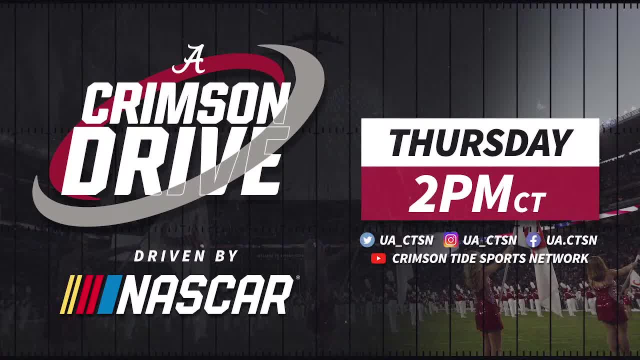 Don't miss out on the opportunity to witness the thrill of four wide racing on one of NASCAR's most iconic tracks. from the blistering speed on the track to the unparalleled fan access at the Talladega garage experience, There's something. there's something for everyone to enjoy. 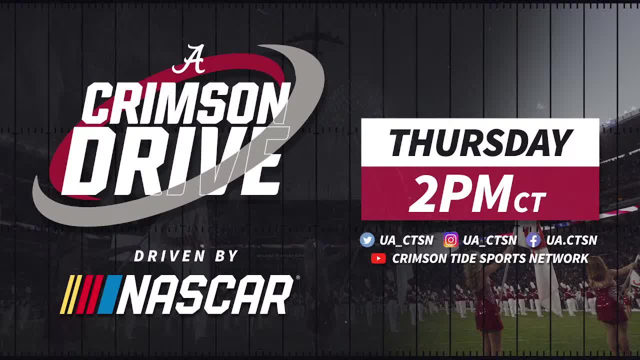 Don't miss out on NASCAR, as much anticipated return to Talladega super speedway for the Geico 500 on April 21st. Purchase your tickets today at Talladega super speedwaycom. Fun conversation with Chris Stewart. Best of luck to Alabama in the final four. 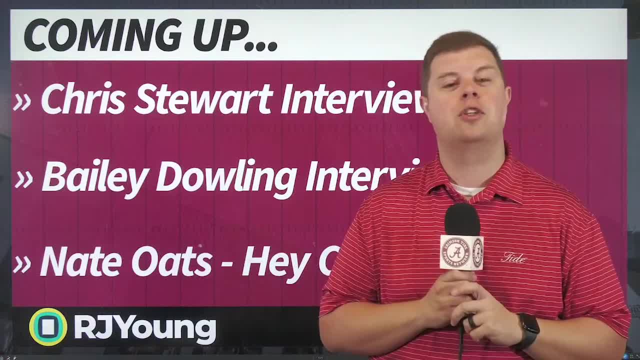 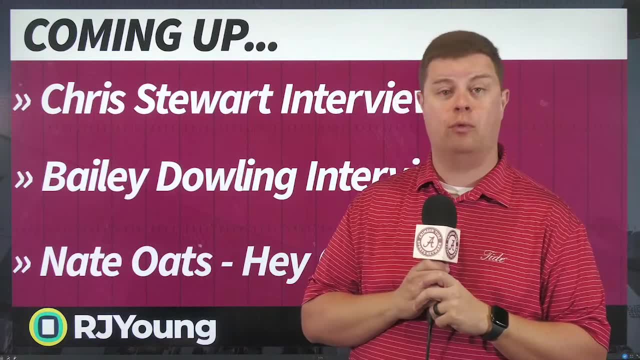 Hopefully we're talking about a national championship coming up next Thursday on Crimson drive driven by NASCAR. We switched gears to Alabama softball and we had a fun conversation as well with Bailey Dowling, third baseman for the Crimson Tide softball team, And she is the first to be on the show. 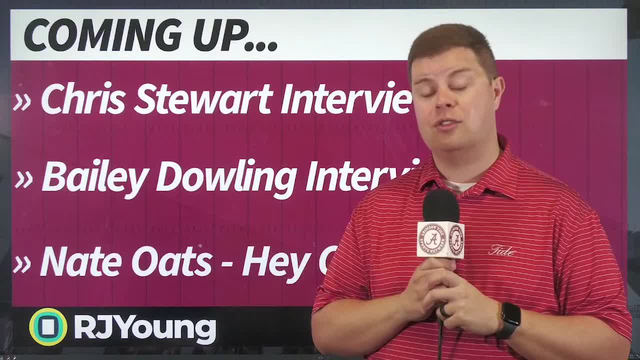 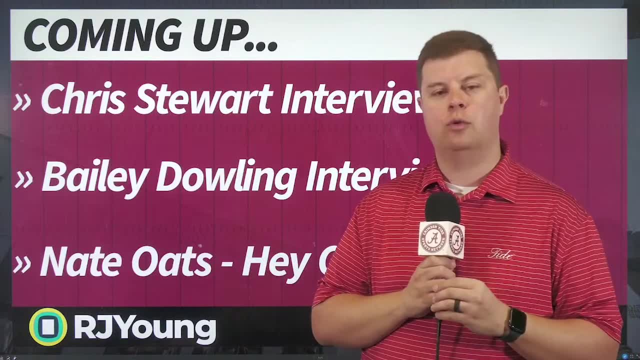 Bailey Dowling is the first student athlete we recorded an interview with in our new podcast studio at the advantage center inside Bryant Denny stadium. Of course the advantage center was unveiled in September- Learfield doing a lot of great work to get that up and running to help connect student athletes with NIL. 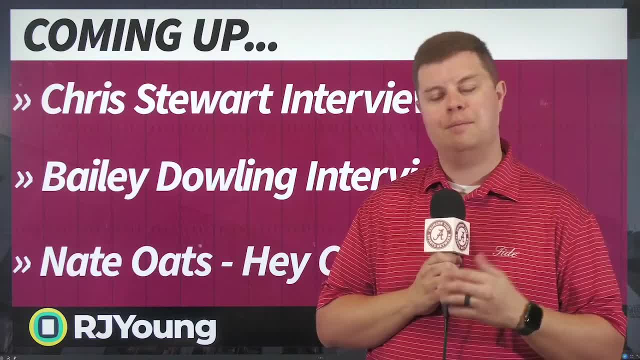 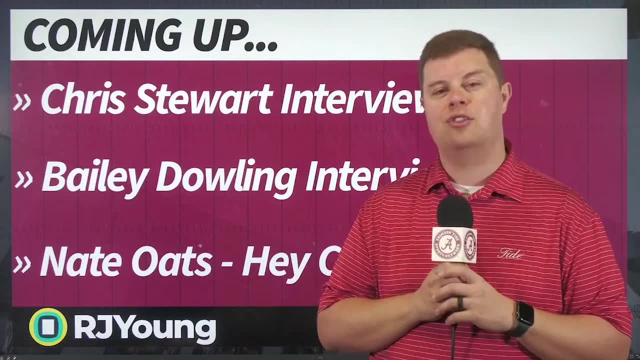 opportunities again through the advantage center at Bryant Denny stadium. So part of that, the podcast studio is going to become the new home for a lot of our student athlete interviews And Bailey Dowling was our first guest. Great conversation about her journey to Tuscaloosa, as you'll hear about. 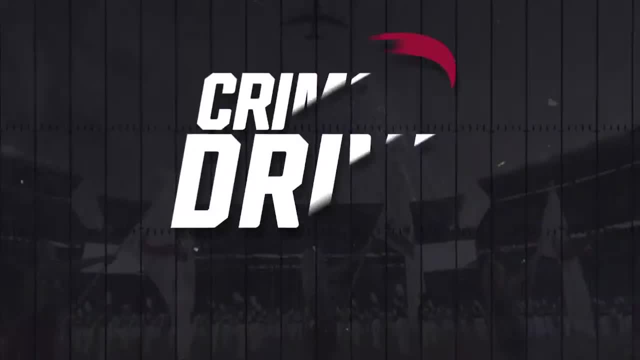 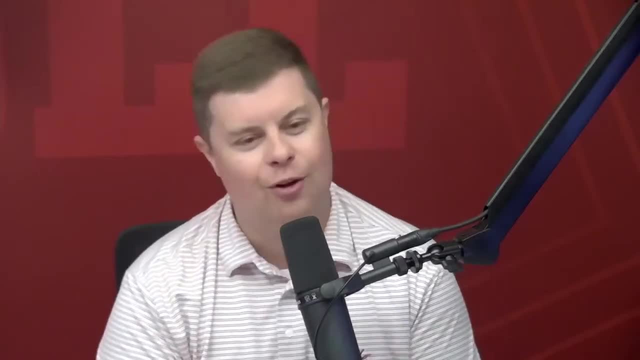 This was a childhood dream for her: to play for the Crimson. Welcome back to Crimson, drive driven by NASCAR. This is Roger Hoover. Now please be joined by Alabama softball third baseman, Bailey Dowling, our first in studio guest here at the advantage center at Bryant Denny stadium. 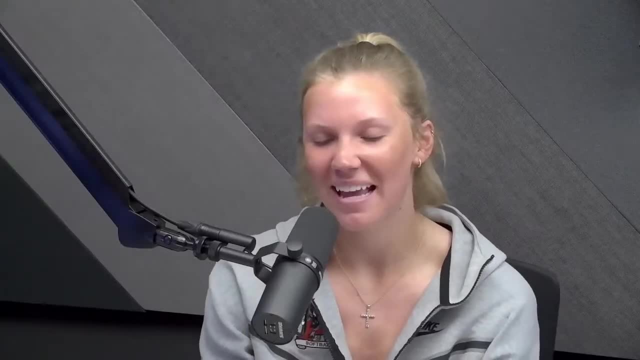 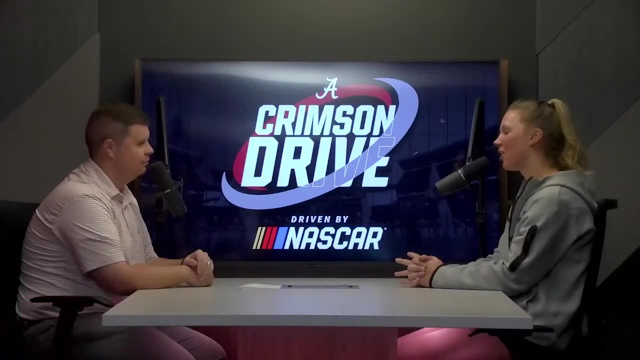 and Bailey roll tide. How's the senior season going for you? Thanks for having me. It's been really fun this year. We have a great team, great team chemistry and it's just been really fun having all our transfers and all the. 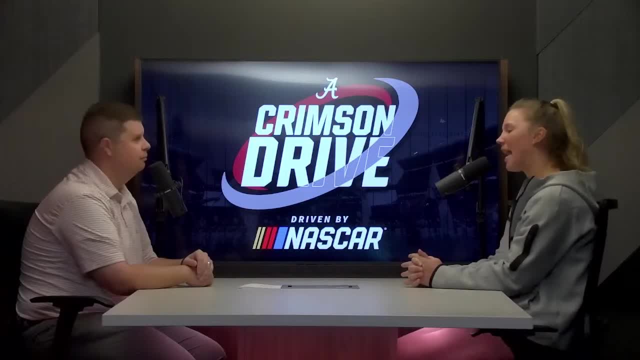 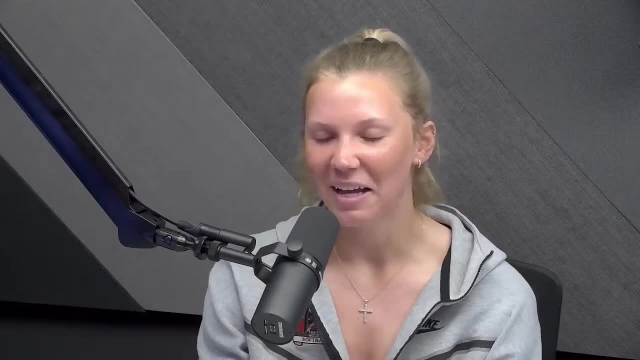 underclassmen, come in and having our new coaches- bro And Adam is our hitting coach. It's just been really fun overall. Has it hit you? This is your senior season? Not yet. It comes and goes- my senior day- It did. 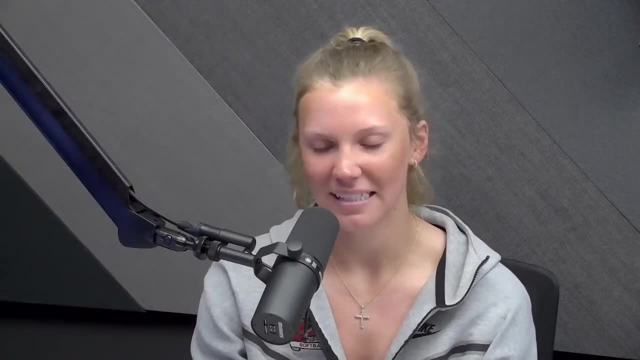 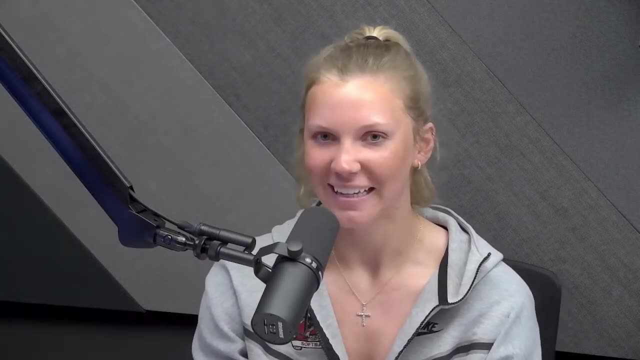 And having all the girls in my class have their senior days. I got really emotional about that, but whenever we just get out there on the field it doesn't really hit me much. So hopefully, hopefully, not till till we're winning more emotional. 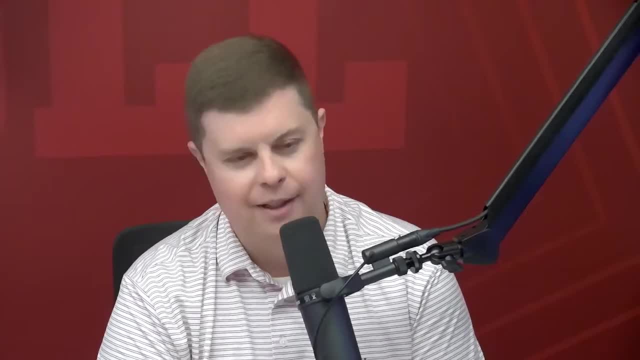 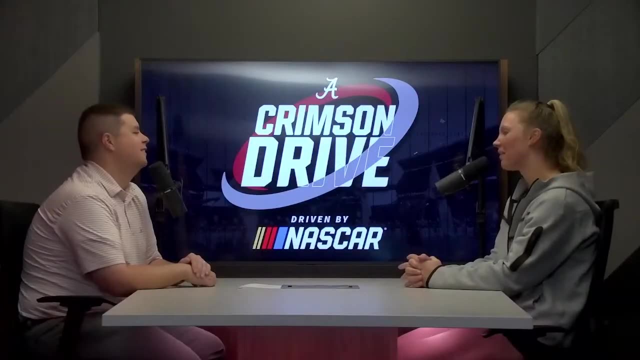 going through your own senior day or seeing your teammates kind of have their family in town getting that. you know the videos are really remarkable, how they get everybody so emotional on senior day. I think honestly everybody else's videos, just because mine. 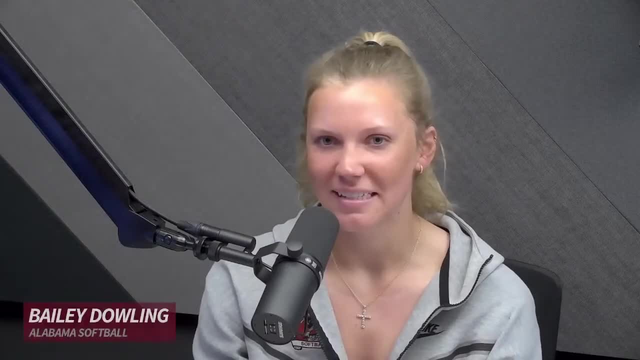 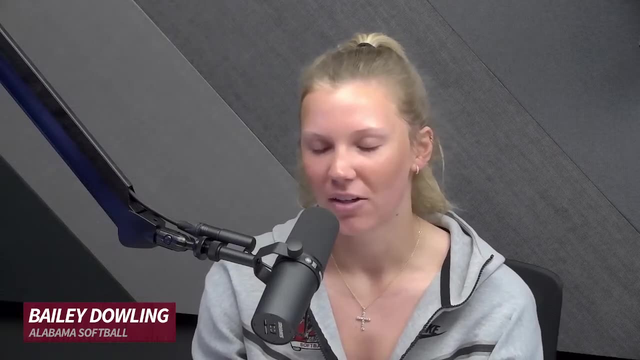 like I made it So I knew what I was going to say. but everybody else is like just seeing them and having them for four years, or like having Jenna here for five years. It's just watching. theirs was really emotional and having their families out. 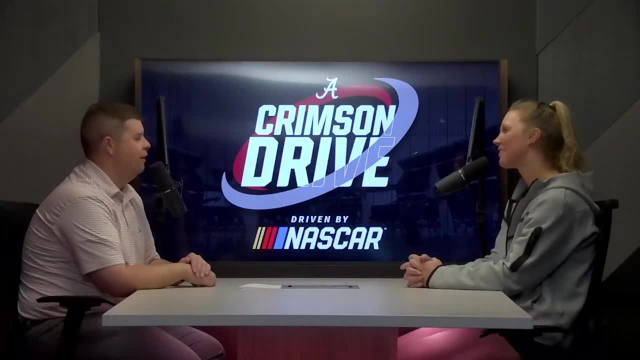 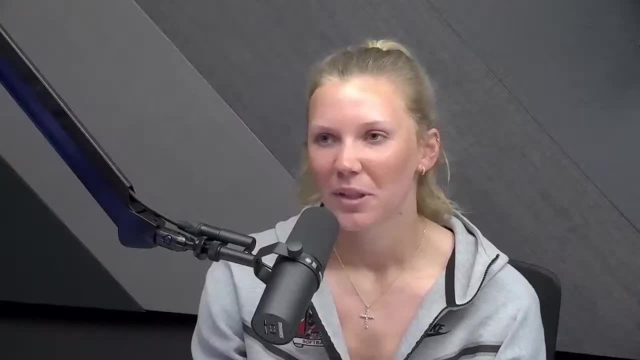 there And, yeah, I would say, watching everybody else's. and for you, the main message was: be fearless. You even gave out wristbands, right? That said, be fearless. Why was it important to spread that message to your team? So when I got hurt, 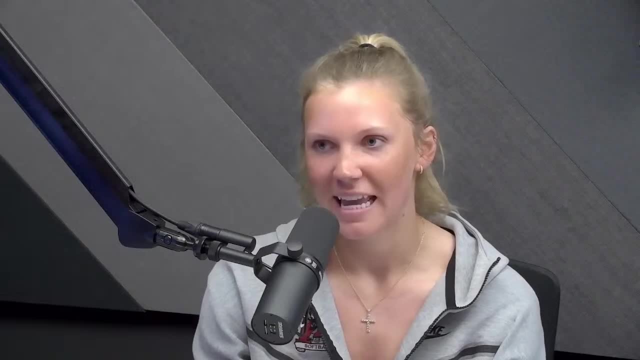 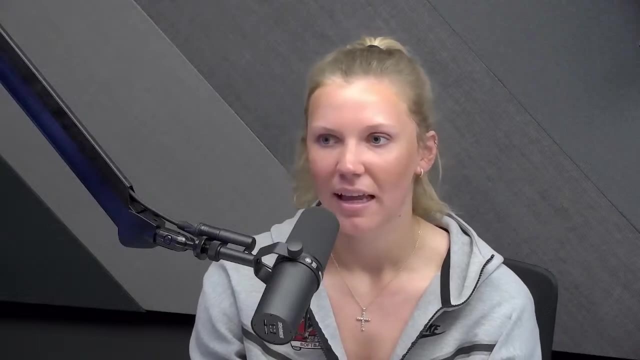 my freshman year I blew out my whole left knee and I didn't really have anything to lean on when that had happened. And my family? I grew up in Illinois so I never had family here. you know, being nine hours away is just the team. 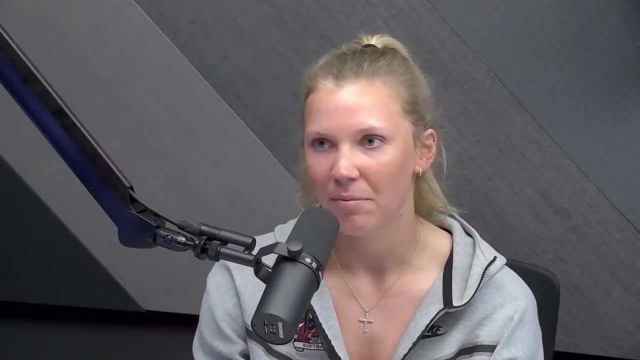 And so being hurt and having to go through that journey and rehab and everything. my mom had always given me bracelets growing up in high school and they always had sayings on them And one of them was be fearless. So that always kind of stuck with me a little bit. 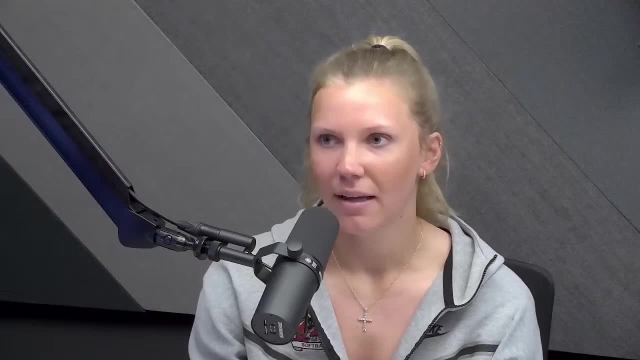 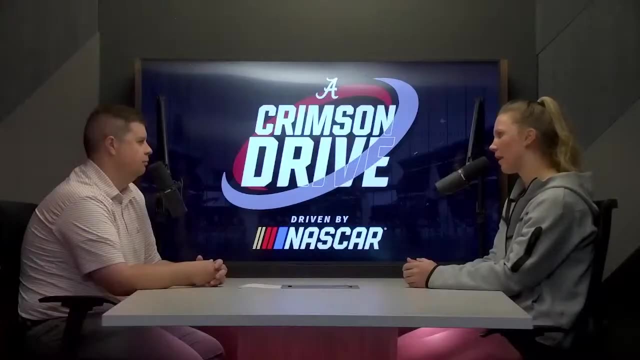 And then we started talking about it and I'd found that bracelet again And that saying just stuck with me. And when you go through a serious injury like that, it's not only hard physically to come back from it, but mentally that's harder. 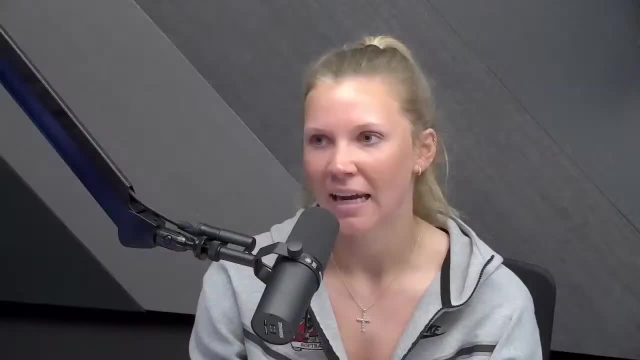 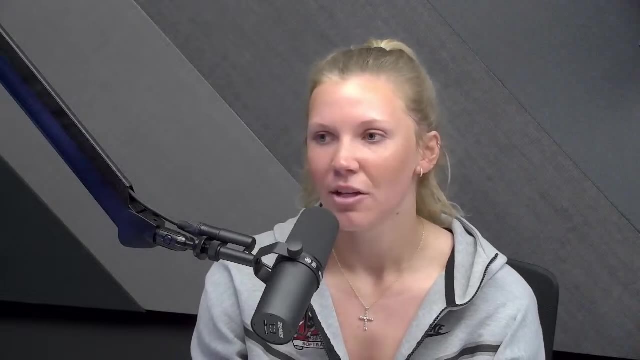 harder to do. And so having that saying it just really stuck with me And I started telling myself like I just need to be fearless through the journey because God always has a plan for me. And just having that saying I really leaned on it and it really helped me get through that. 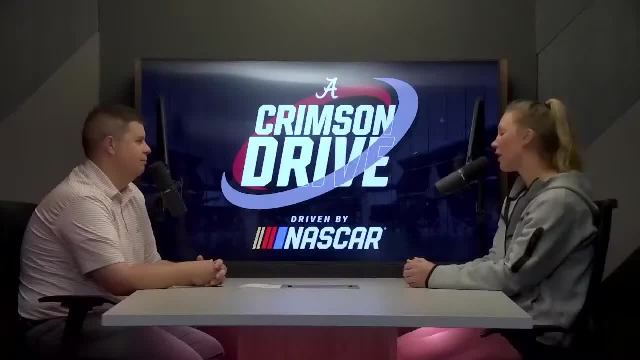 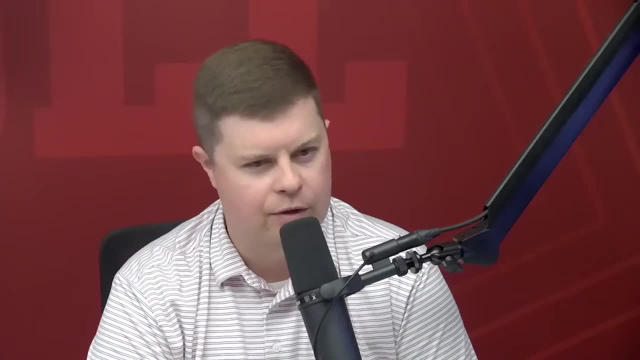 And um, it's really stuck with me since then, And um, so I gave bracelets out to everybody for that, And just so it's a little part of me that I gave to them. What does it mean to you now, when you could see that with your teammates now? 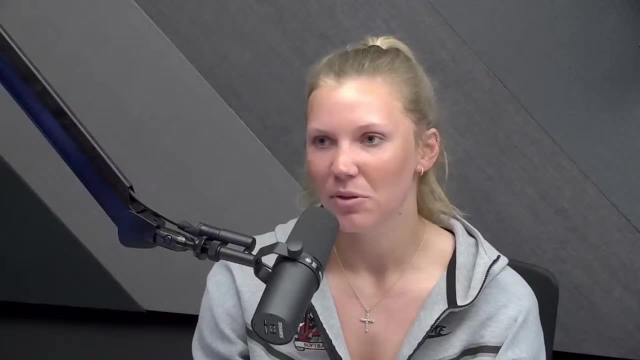 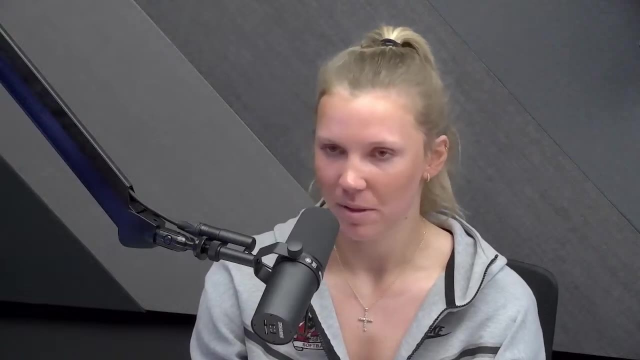 they're adopting that as kind of their mantra for the rest of the year. I think it's awesome, because when you step on the field you can't have any fear going out there. and this game- you can't be perfect. It's impossible to be perfect. 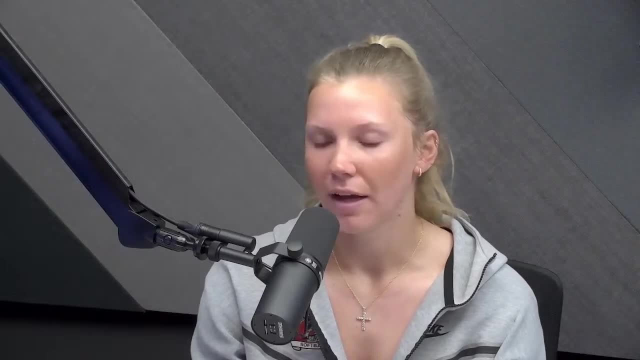 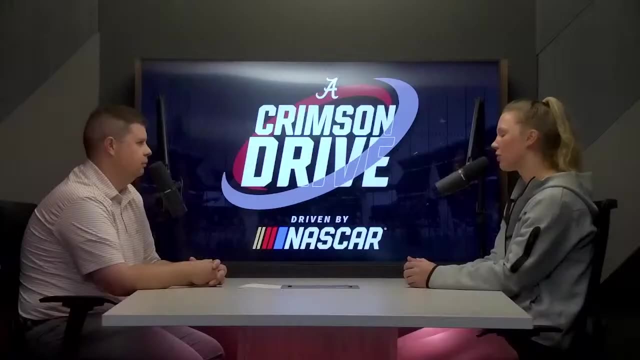 So not being scared of failing or, you know, not getting the job done when the team needs you to come through Like you got to give yourself some grace, And so being fearless when you step out there, that's just. that's just part of the game that you have to have. 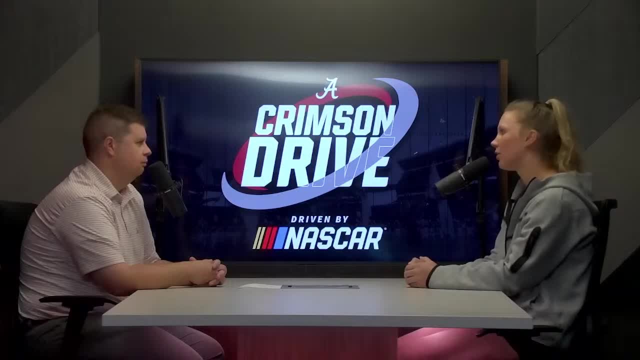 And that's how you become good, And so I think it's cool to see that my teammates adapted that, because that's been a part of my journey for a really long time, And that's you know, you're not always going to be perfect. 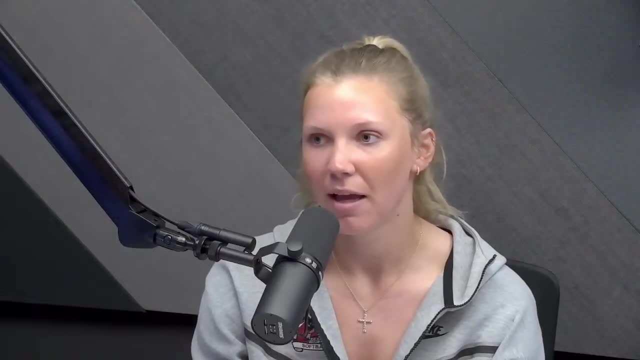 I'm not always going to be fearless when I get out there, because you know there's always going to be moments, But having that, having that with me in my back pocket, is always good, And seeing my teammates have that, it's really cool. 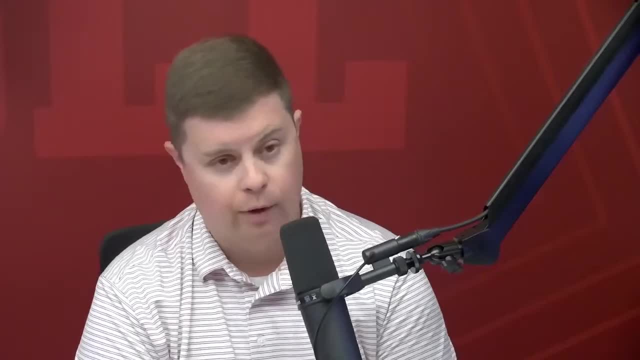 So you did that on your senior day. then we'll get to uh what this team is capable of The rest of the way coming up. but I want to go back. It's the beginning of your journey. I just tell us where you're from and what got you interested in softball. 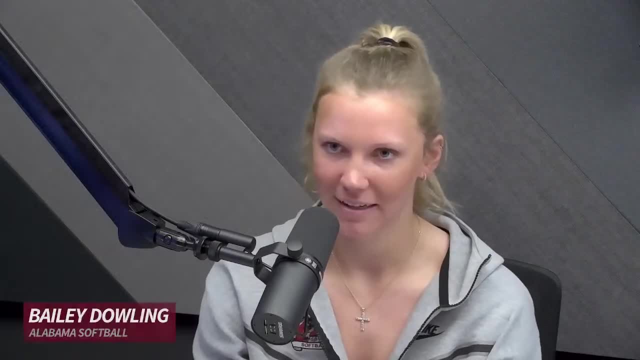 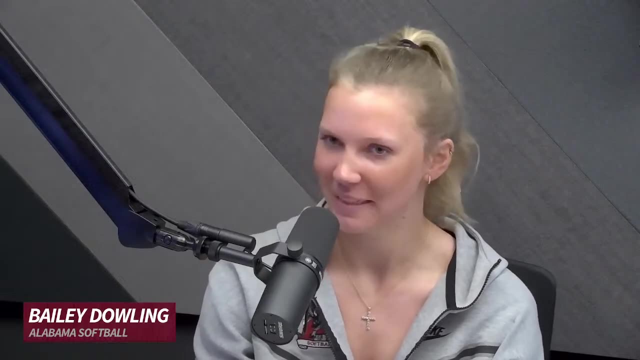 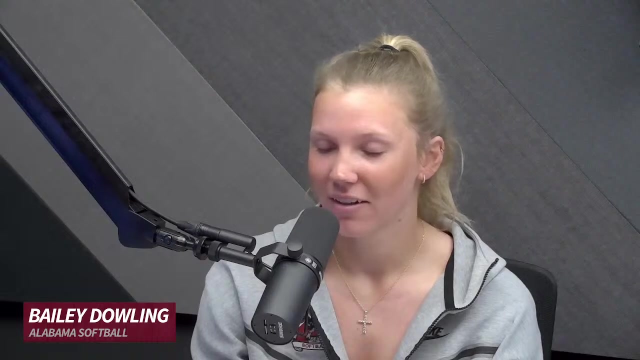 I'm from St Joseph, Illinois, a small town next to Champaign. Um, it's actually really cool, cause Lance coached at um Illinois, So we kind of had that little bond when he came in here. Um, I grew up playing soccer and I actually love soccer and I was very shy because I have two half sisters and they never lived with us. 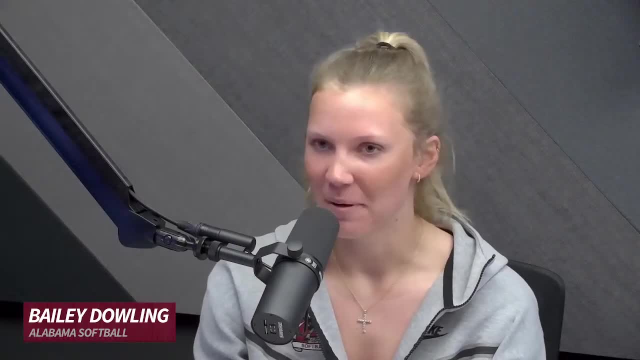 And so I'm the only child Really, And I just didn't talk much, just really shy. And my mom forced me to play T-ball, like I did. I did not want to at all, And once we got out there to the first practice, 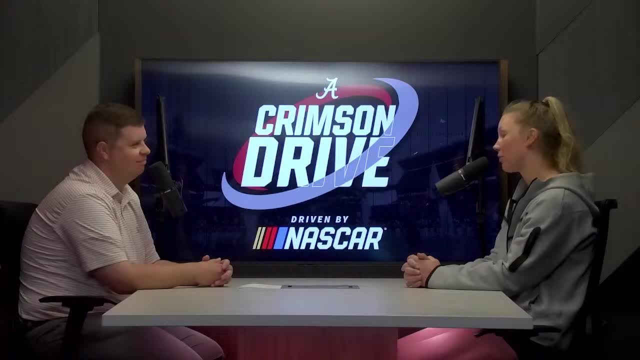 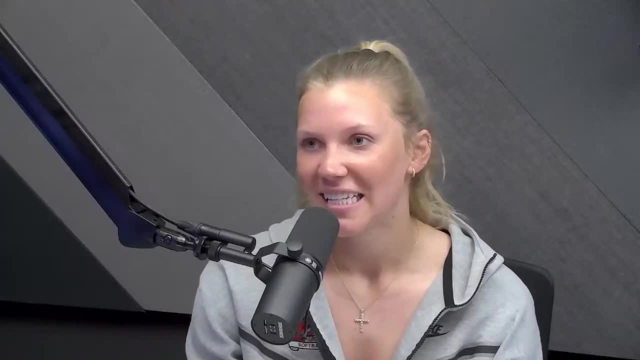 I remember I dove in mud because we weren't even on a field, because we were so small, and I loved it ever since I dove and just got dirty And so I've been playing it ever since then And, um, my dream was always to come to Alabama or play here. 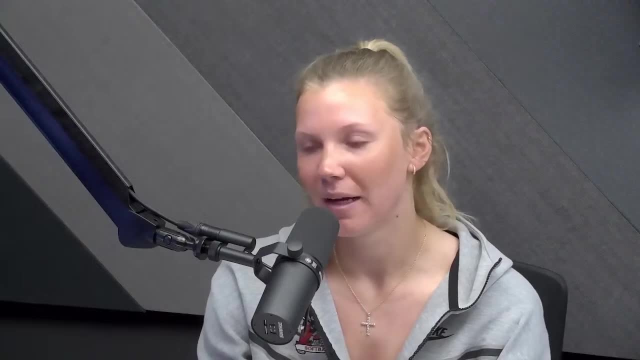 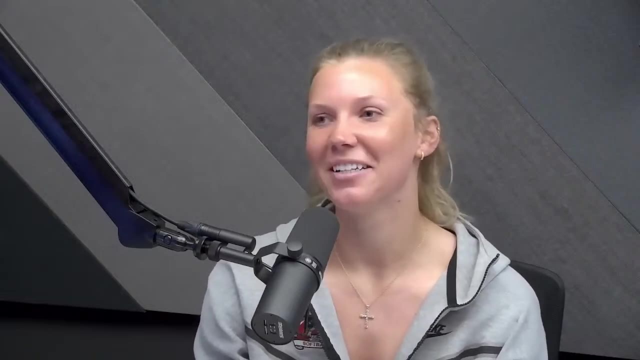 And there's a lot of other schools that were on the list, but Alabama was always the number one, And I don't know why, because when you're young it's always like the name or the colors of the school, or like just their jerseys and everything like that. 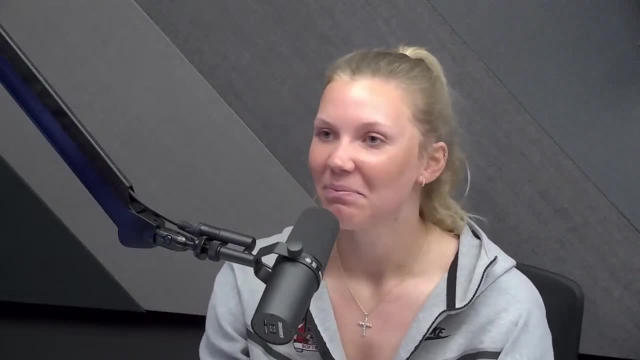 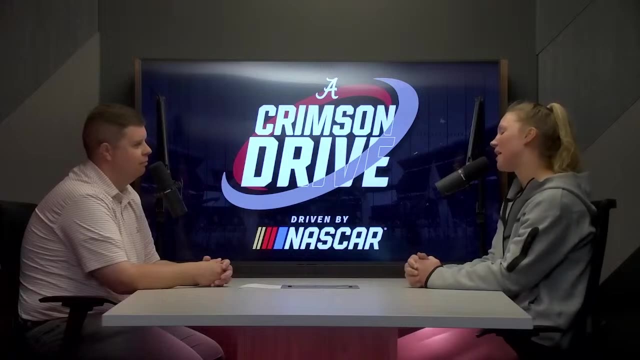 And I guess I just really liked crimson and white. Um, but yeah, Alabama was always number one and, being so close to Illinois, we always- my parents- got to take me and watch all their games. And Illinois actually played Alabama a couple of different times. 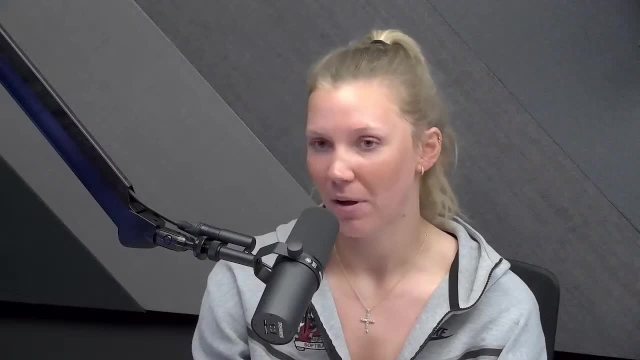 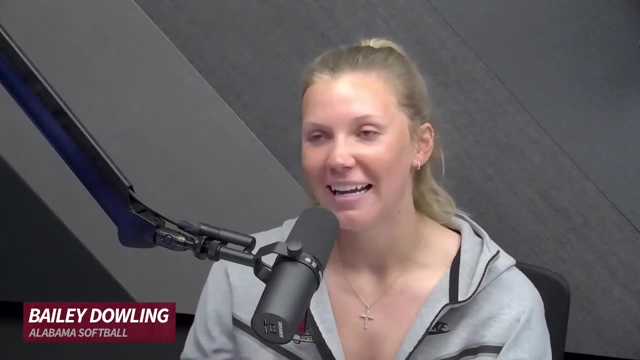 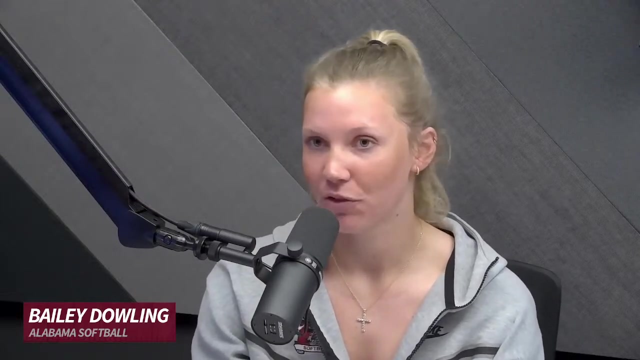 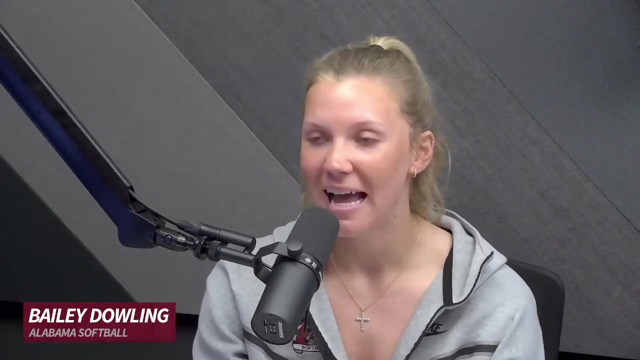 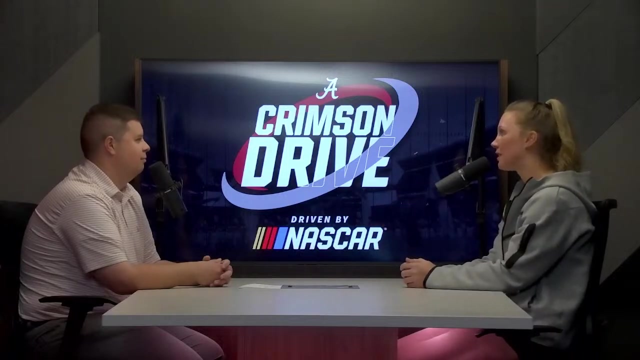 And one of them. my parents had drove me to Northern Iowa And the dome and they had played because it was so cold and they couldn't play outside and Illinois had played Alabama and it was when Jackie Traynor was on the team still and in between games she had made peanut butter and jelly sandwiches for everybody on the team, like without being told to or asked to. she just started hanging them out and making them and me and my dad had stood on the ledge over looking the dugout where she was making them and it was just the coolest thing because my dad was showing me like 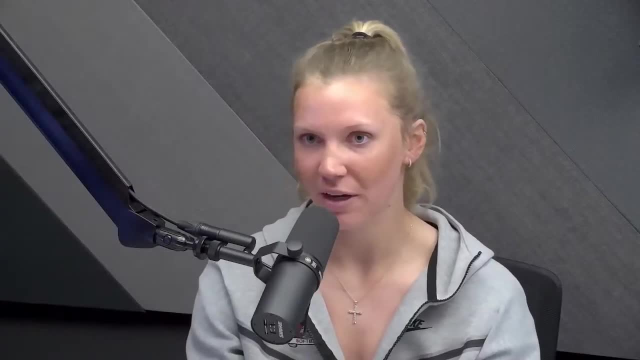 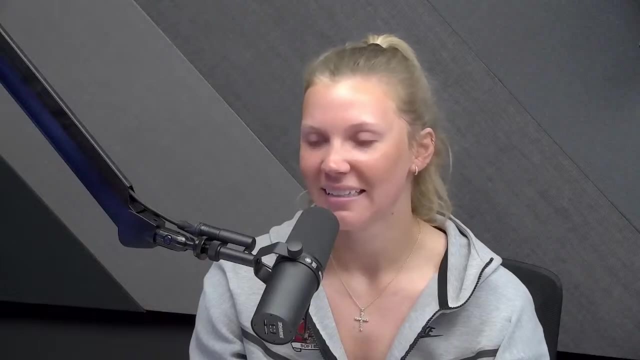 Hey, that's how you become a good teammate. Like she's doing it without being told, but like seeing that it was just really cool And um, since then, that moment that was very clear that I just wanted, wanted to play here. 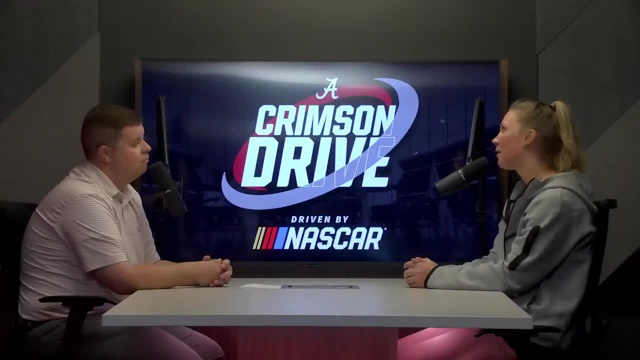 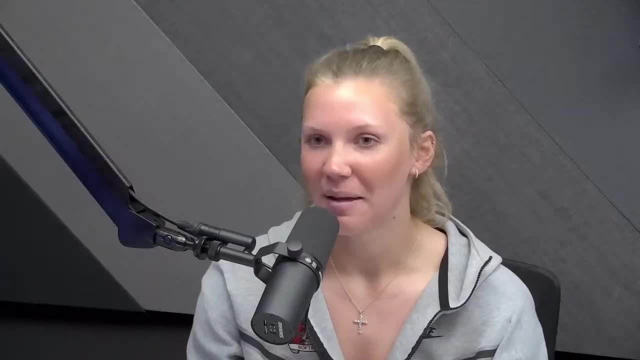 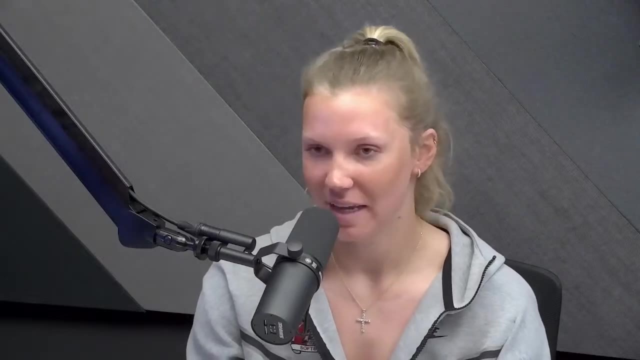 And I actually wrote a letter to an um elementary school- I think it was the third grade. Our teacher had asked us to write like our dream or what we wanted to do when we got older, And I had wrote that. I wanted to hear the crowd say my name at the Alabama Field whenever I'm stepping in the box. 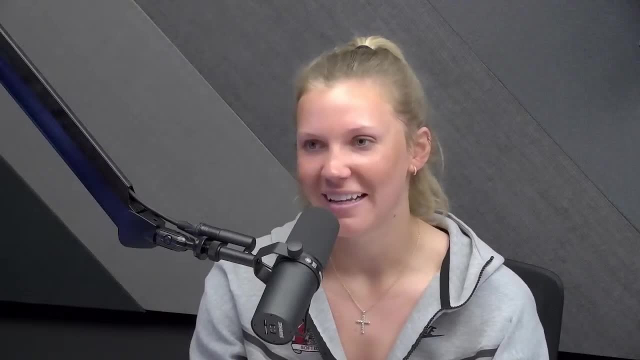 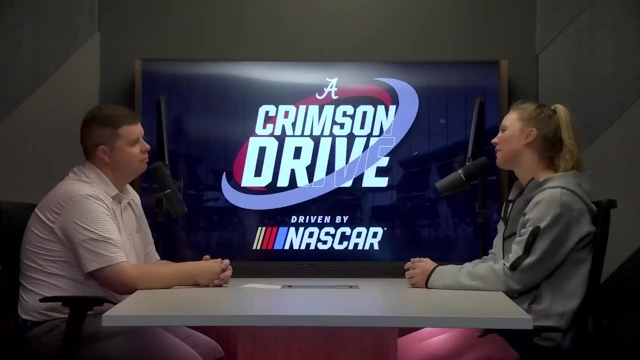 So whenever I had committed here, my mom had brought the letter and like showed the coaches and there's just a really cool like Pivotal moment and It was super cool to see the reaction to that because this really was John Cole deze ring from the beginning. 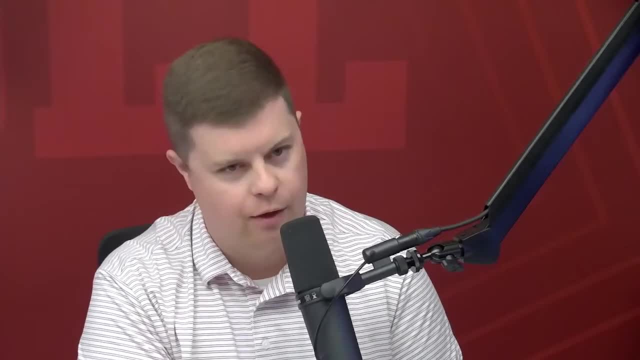 So you have the dream at a really young age. What's the work like the making sure you are on the right track to play for the University of Alabama? What's the dream like in the beginning? What's the work like, though, making sure you are on the right track to play for the University of Alabama? 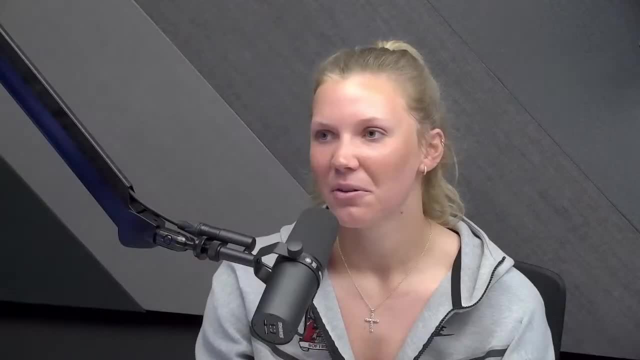 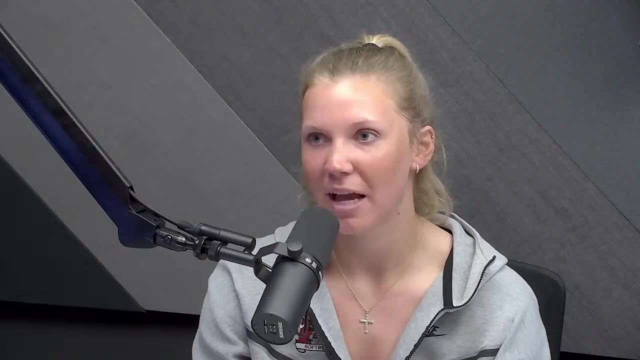 What's the work like, though, making sure you are on the right track to play for the University of Alabama? you do in middle school and high school to become a great all-around player. so, thankfully, growing up so close to the U of I, my parents always got to take me to their games and we actually became 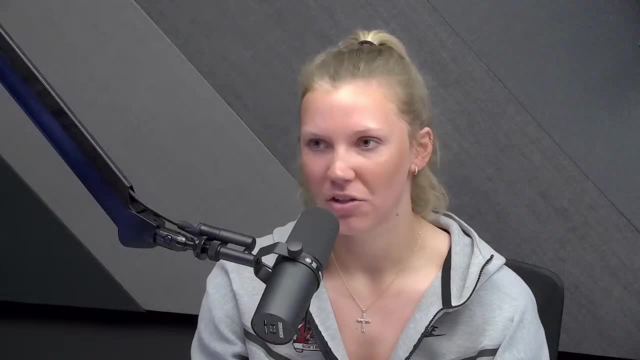 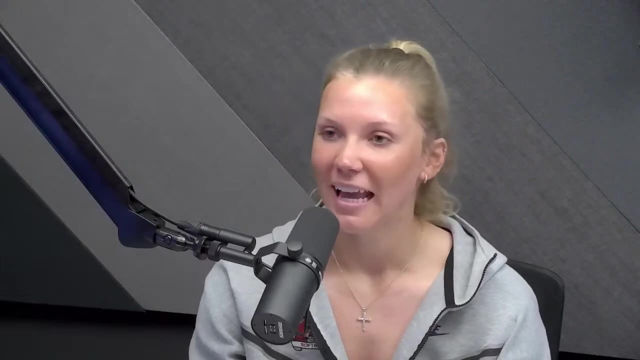 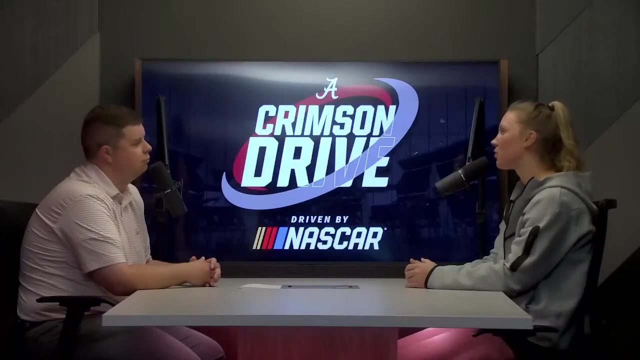 really close with a lot of the players, and one of them- Kelly Cervantes- now she was Kelly Waddell- had married one of the Illinois baseball players and they became my coaches at a very young age, like 10 or something, and so I grew up having them just teach me softball and give me lessons. 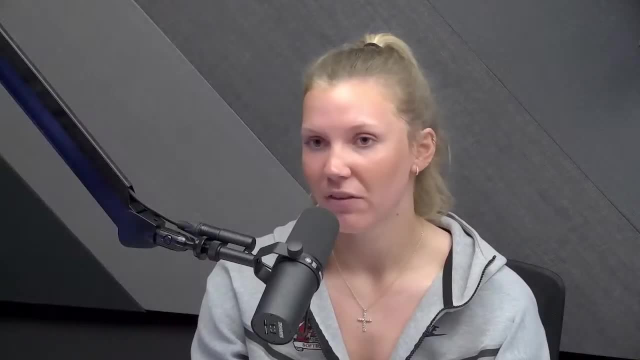 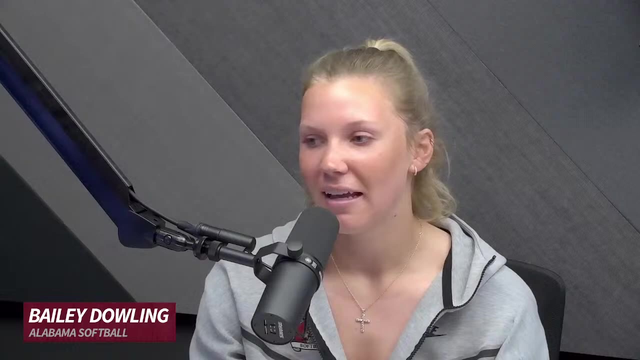 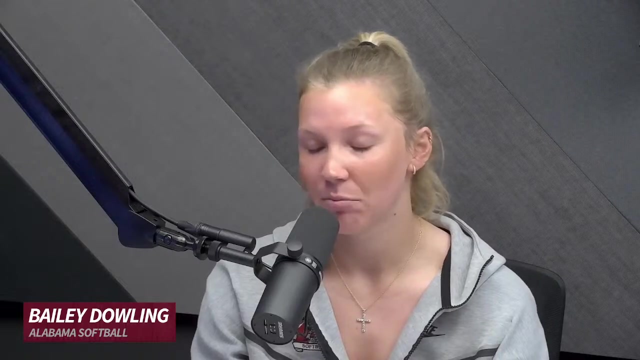 and they were my travel ball coach for a while and I still, whenever I go home, that's who I work out with, so they're- they're who got me here today, for sure, but yeah, I, we would have practices all the time and I'd always be having like a two-hour lesson before after practice. it was insane to look. 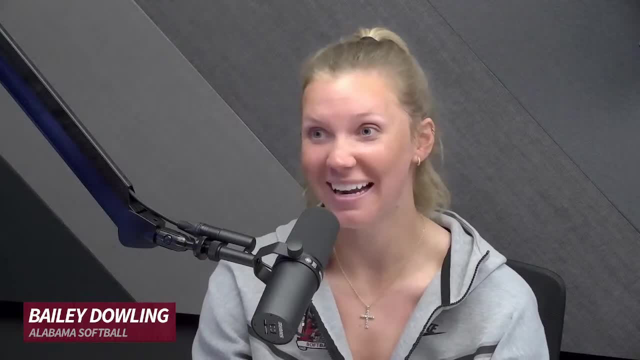 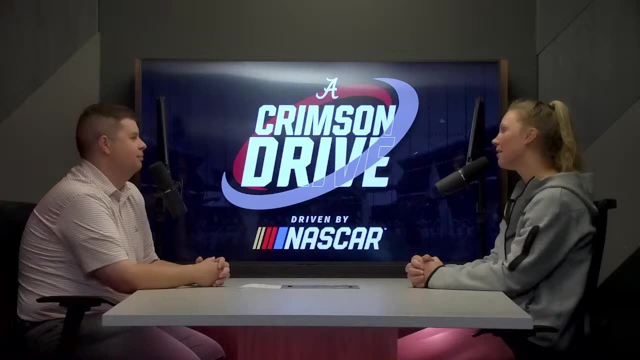 at now, you, you. I'm just thankful that my parents gave me that opportunity and that we were so close to Illinois that we got to become close with Kelly and Matt and that I had that chance to get to work with them, because I wouldn't be here without them. and of course, everybody grinds it out in the batting. 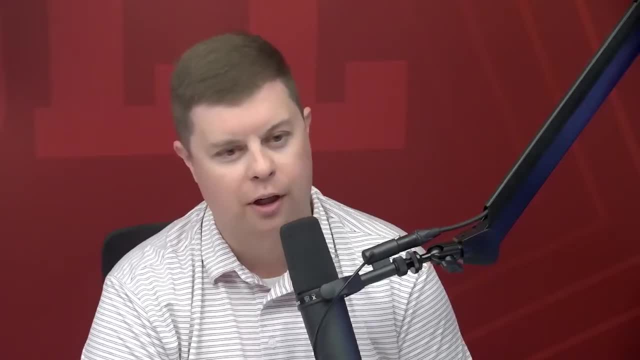 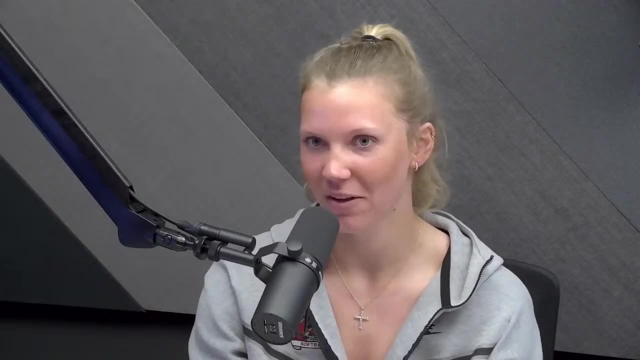 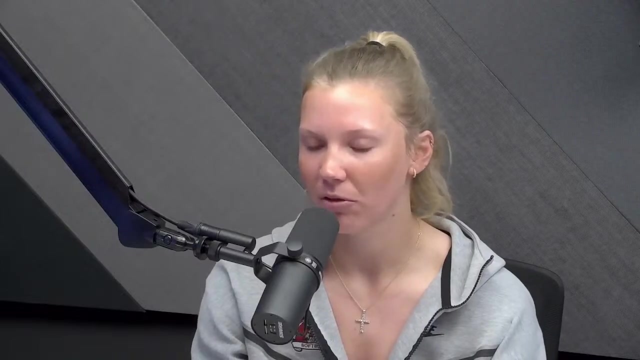 cages, but for you, I mean, the batting cages are only a few steps away. tell us about the barn. yeah, I call it the shed, but I guess people don't call it a shed because sheds are small. so, yeah, the barn. um, whenever I got old enough and softball really was like I always wanted to play. 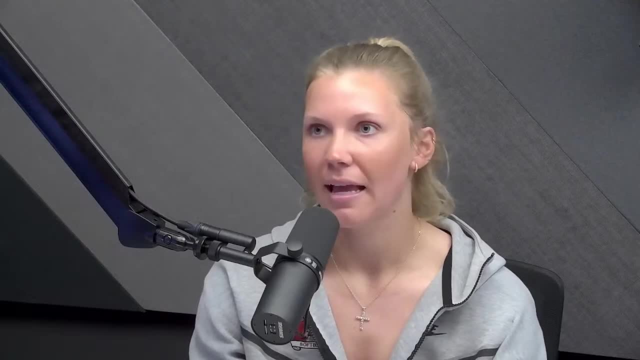 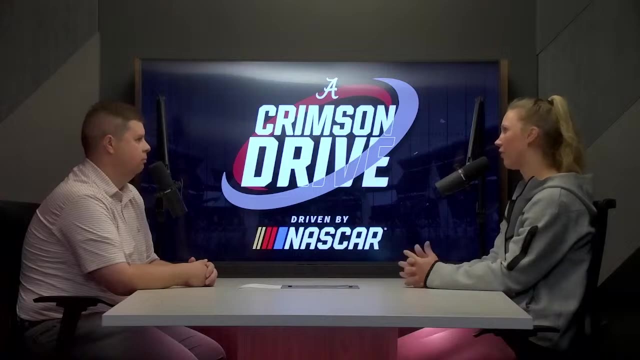 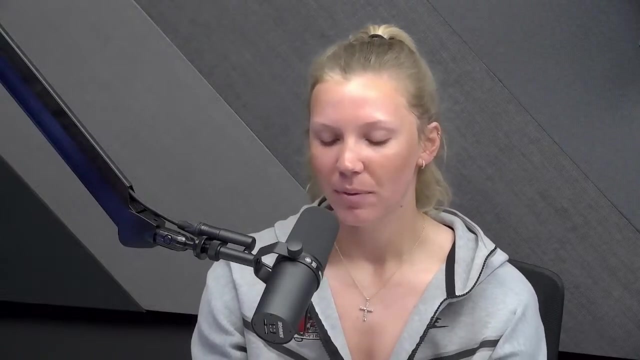 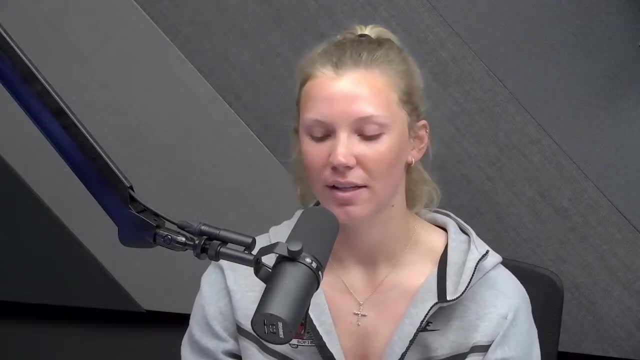 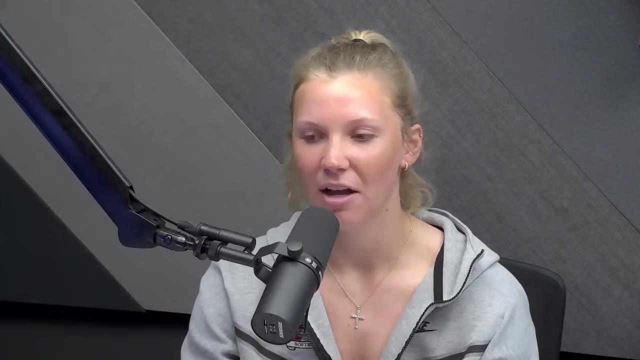 is for all of his construction stuff, and then two-thirds is all turf with a basketball hoop and then a batting cage, and so that's where I got to do all my lessons and everything growing up, and it's just really cool to have that in my backyard, because then when I did get into high school, I 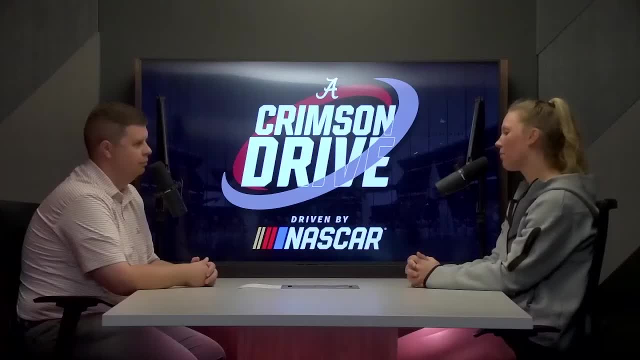 could you know, give my own lessons to other girls growing up in our town, and so it's been really cool just to see that I got to grow up there getting lessons from Matt and Kelly and now I'm giving lessons out of it, so I'm very thankful for it. 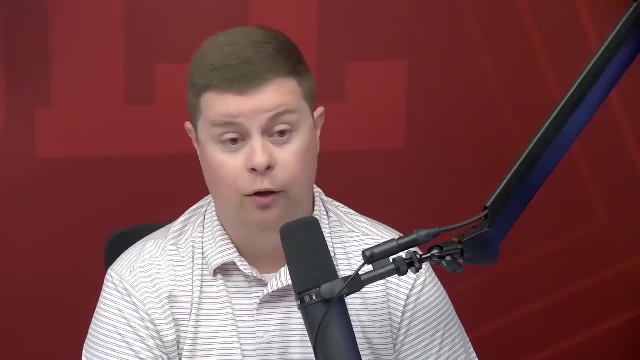 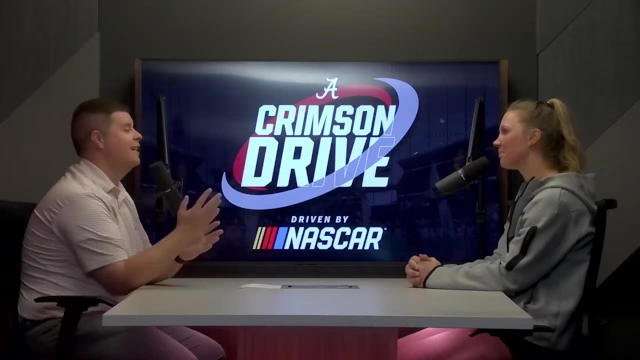 that really is cool. again, a lot of home runs for you as you cook Illinois softball by storm. you have the career home run record in Illinois and then you're getting ready for that senior season, getting close to the national record. then the COVID-19 pandemic. just how tough was it to see. 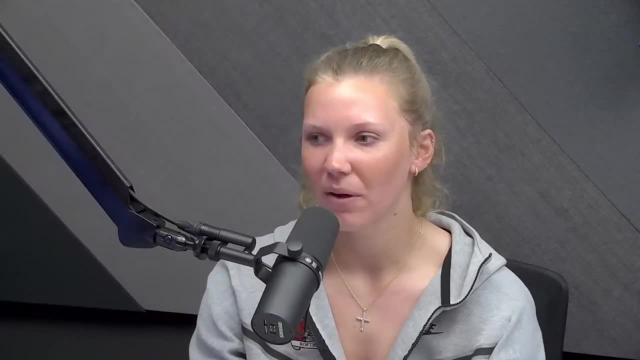 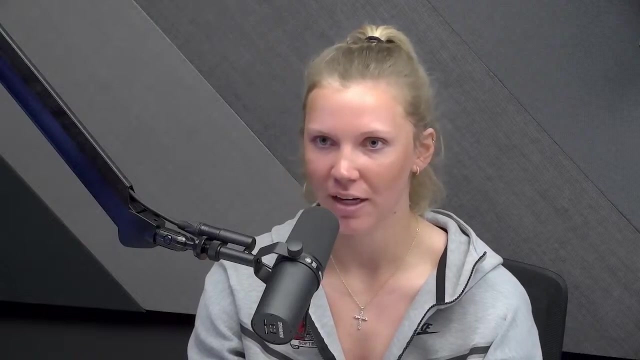 your senior season cut short. I think it was more hard just knowing that. take away all the records and everything, just that. that's a huge moment for anybody that is moving on with their life. like being a senior in high school, I didn't get a walk for graduation like I had nobody- nobody there our high school, thankfully. 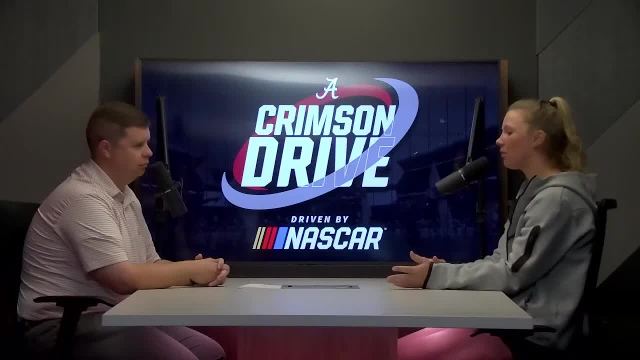 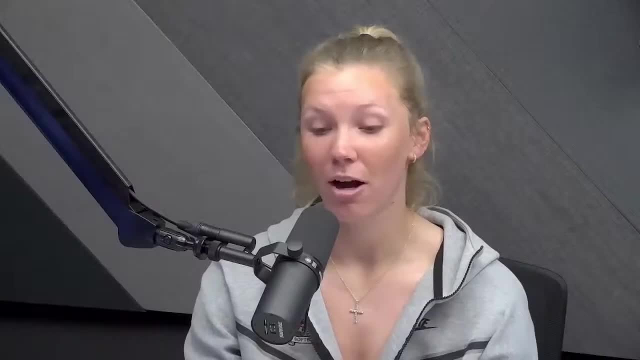 let us walk individually. so you picked a time and you could go in on your own and you got to choose four people to be there and you walked. there was nobody in the gym, it was just you, and they made a video out of it, which was really cool, but you know you don't have that true high school. 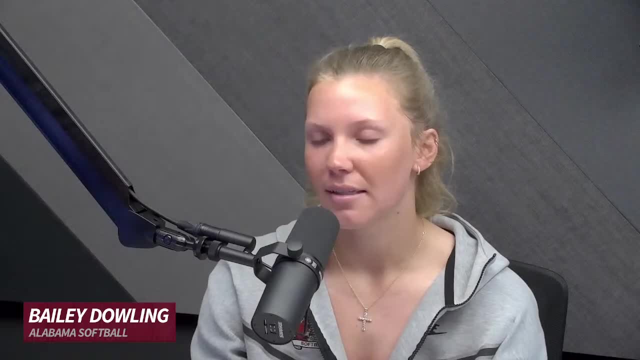 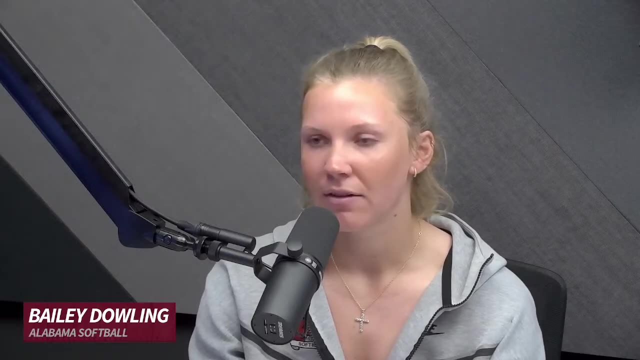 experience. so just having those things, I guess, taken away, it was really hard, and I remember that our high school had a lot of people that were there and they were like, oh my god, I'm going to get a night where, after everybody, had found out that you won't have any spring sports, or you know. 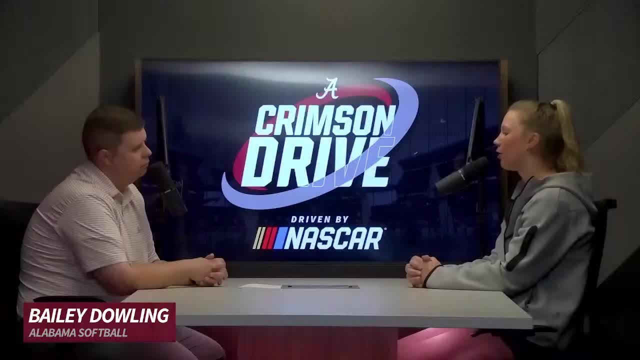 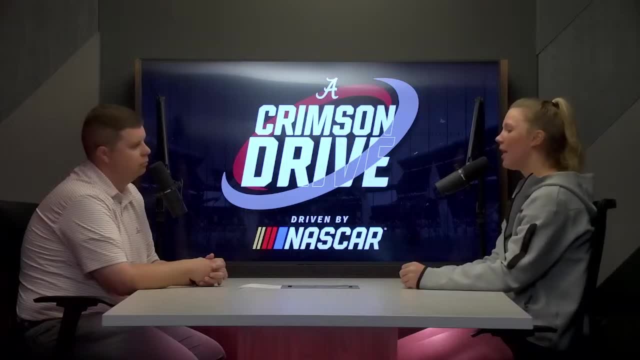 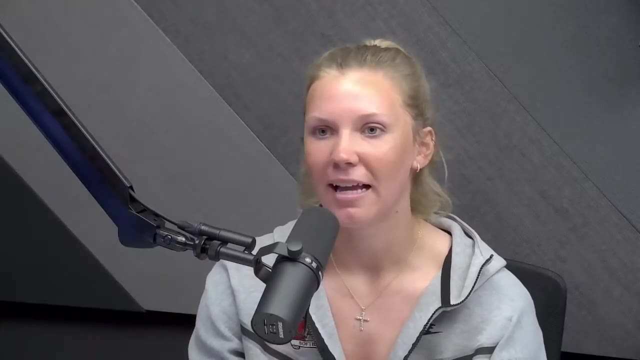 we won't be going back to school. our softball coach had taken all our jerseys and put them on like a pole or a stick or whatever, and whatever our position was, they went and put them out there on the field. so that night anybody from St Joe could come by and, like, I guess, give thanks for. 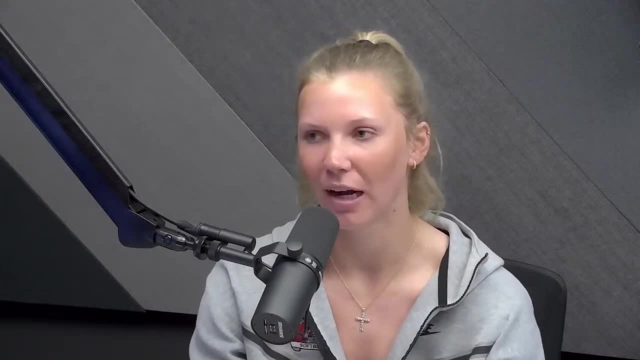 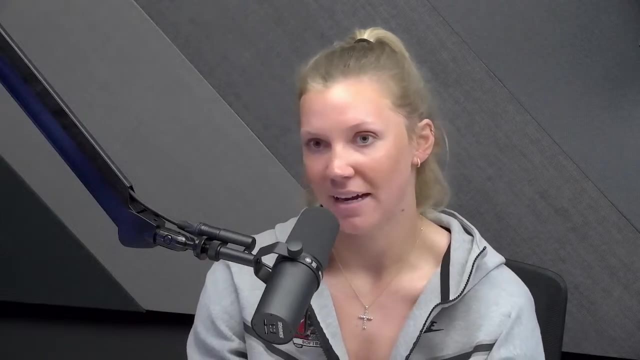 like everybody, all the seniors are going to be there, and they're going to be there and they're whatever, and just show them support. and we got to, I guess, be out there for a couple hours and just experience that without even having anything to do. so I'm thankful for that and just everything. 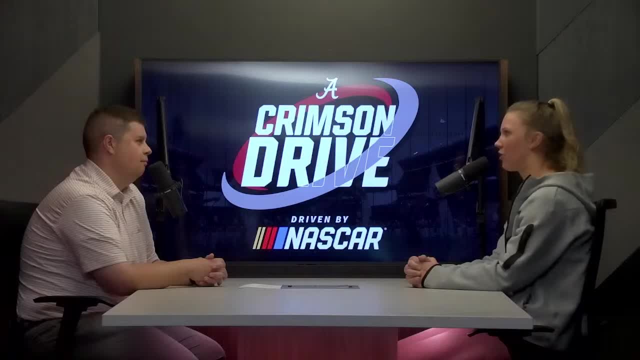 our high school did, when we didn't have an opportunity to finish our season or, I guess, really even start it. so I mean it was cool that they had that opportunity to give us. so that's a whirlwind of a spring dealing with all that and then over the summer and getting ready for the 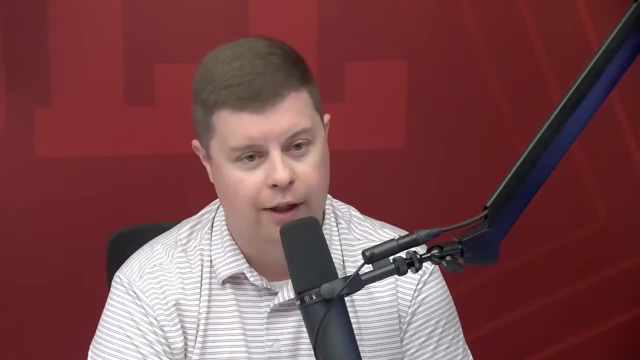 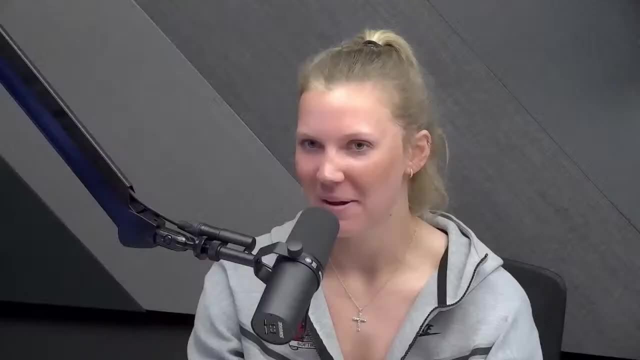 fall season and getting ready to move here to Tuscaloosa, Alabama. what was that transition like? finally joining the softball program? it was really awesome and honestly, I was so excited just to be on my own because my family is very close and anytime that I had a travel ball tournament it. 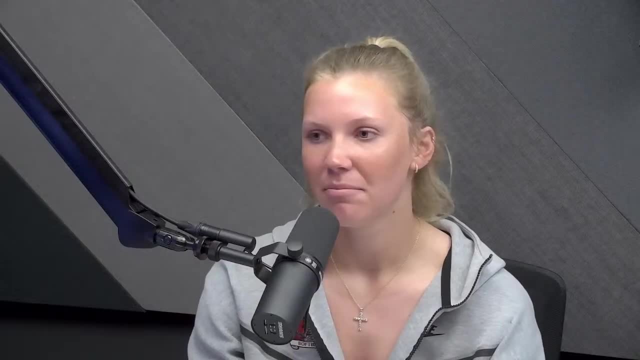 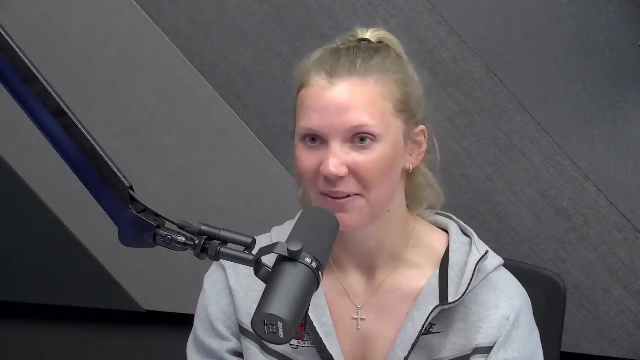 was always me and both of my parents, and so we were just always together all the time. and I want to, I want to take that away for anything, but when I'm actually on my own, it was fun just to sit and I felt like I was just in a whole different world, like it was a new Bailey, even though it 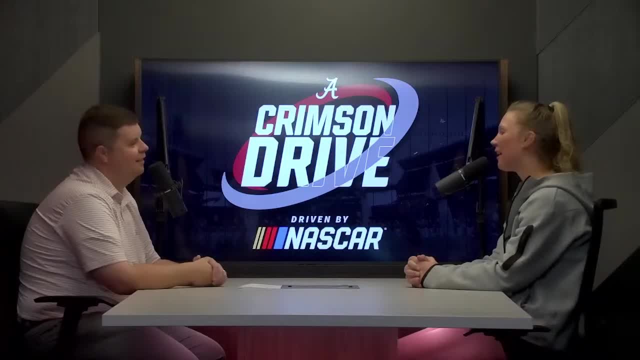 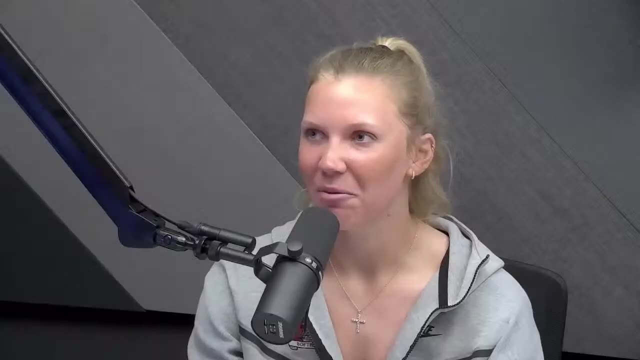 really wasn't, it was just exciting. but yeah, I remember just being really excited to be off on my own and kind of just have that new, new moment to adjust and show my responsibility. and yeah, I don't really honestly remember much because after I'd gotten hurt I feel like all those memories. 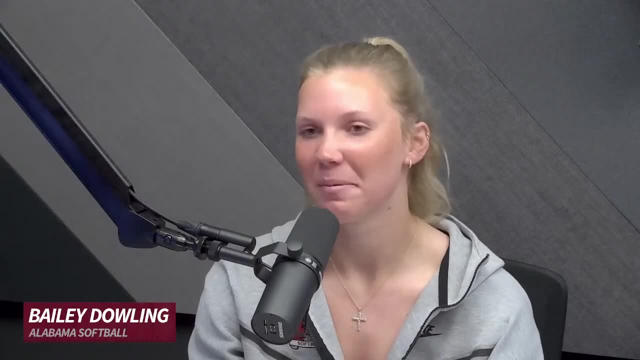 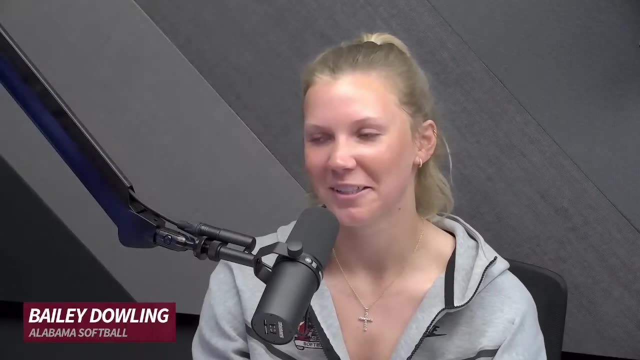 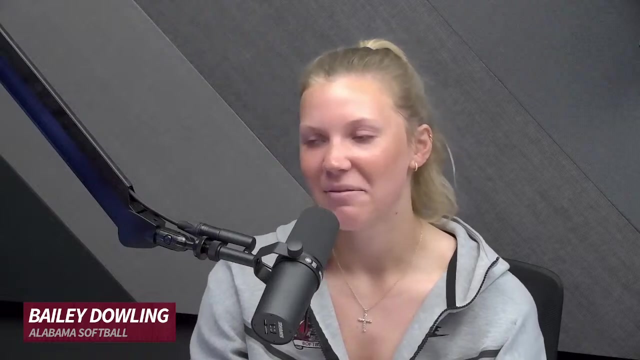 were a blur, but yeah, I do specifically remember that part. who were some of the leaders on the team that took you under their wing? Claire Jenkins and Bailey Hempel, for sure, and it was really cool. Claire actually came back our Virginia Tech weekend at home and we got to hang out. and then Bailey and her parents came. 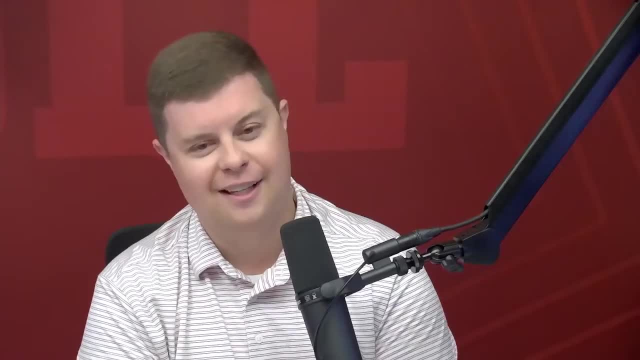 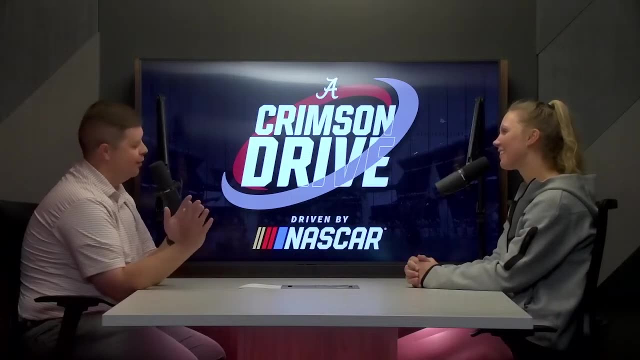 back for my senior weekend. so it was an Alabama fan, as we learned. and then you get to know him in the recruiting process. everything's really positive, but then he's got to coach you at times. what was that transition like? going from you know Murph, that's trying to sign you versus. 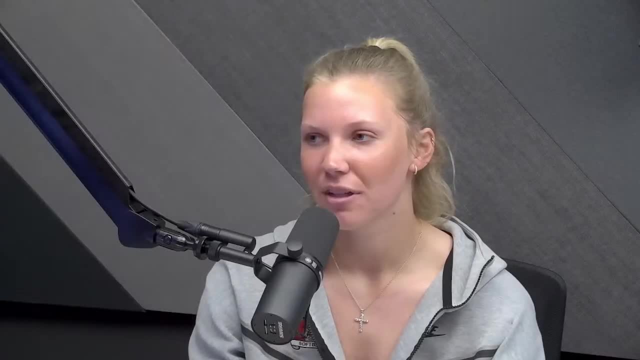 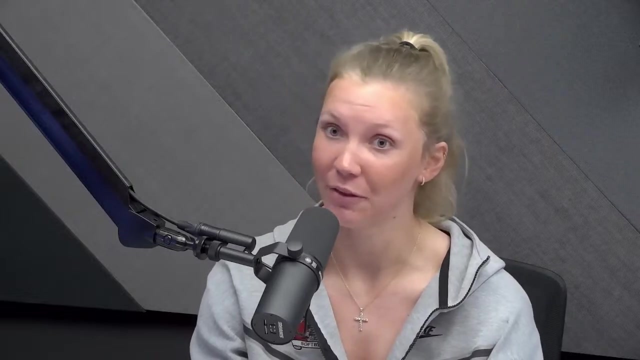 not your coach. well, they always preach, you know, like person first, athlete second, and that is really true here, and just how they recruit you, they're the same person as how they're coaching you. obviously there's times where they have to get on you and they're not going to get on you and 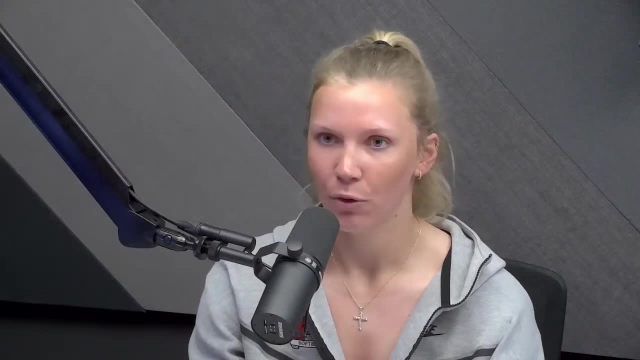 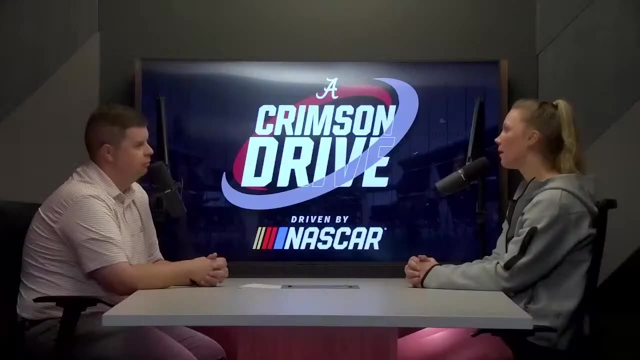 they're recruiting you, but they never changed of who they are, and I think that just shows a lot and speaks a lot about who our coaches truly are as people, because you can put on a show- and you can- you're recruiting somebody and be completely different when you're coaching them, and that's. 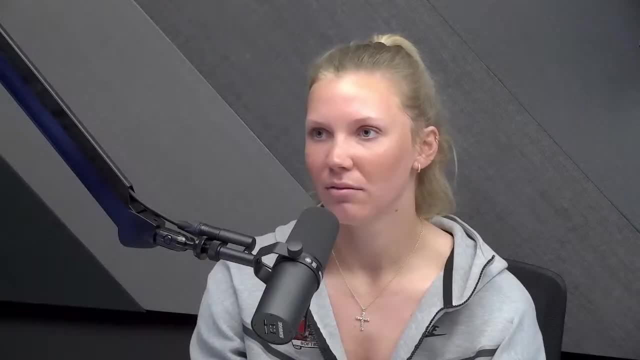 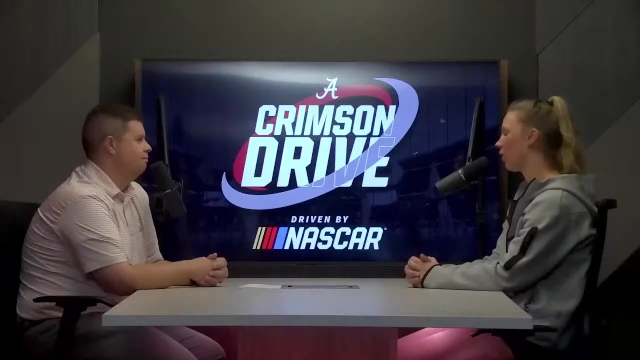 not the case here, and I think that's just one of the one of the many reasons why I love it here and why this is home, because I'm getting better as an athlete here, but they're teaching me how to also be a great person, and when I leave here, those are what I'm going to take with me, not worrying. 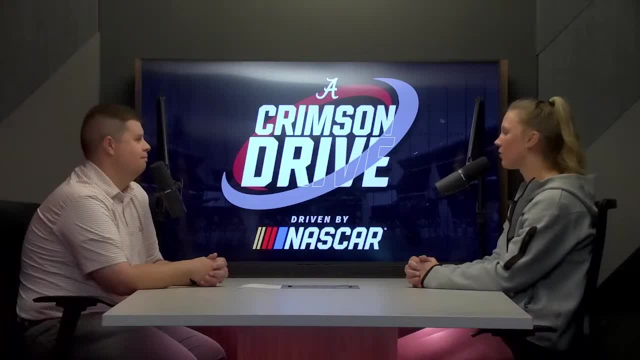 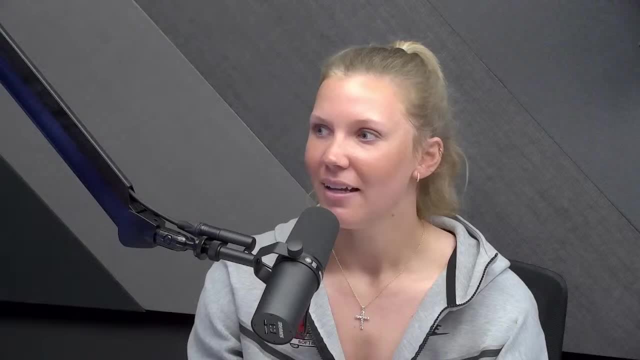 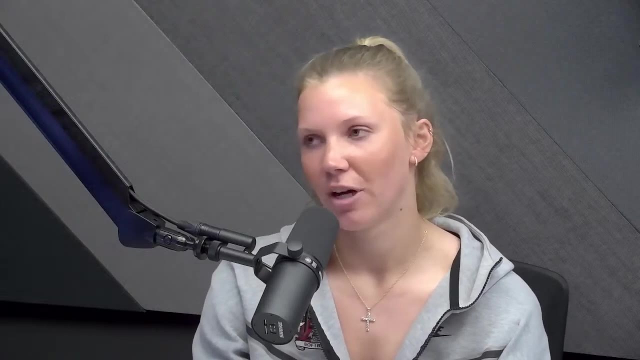 about my stats or what my records were here. so I think that's really cool. when was the first time you heard the word mudita? oh I, honestly, it was when I was being recruited. there was a specific moment that I remember, but it was when I was being recruited and, um, when you get here, you have to learn how to think on your 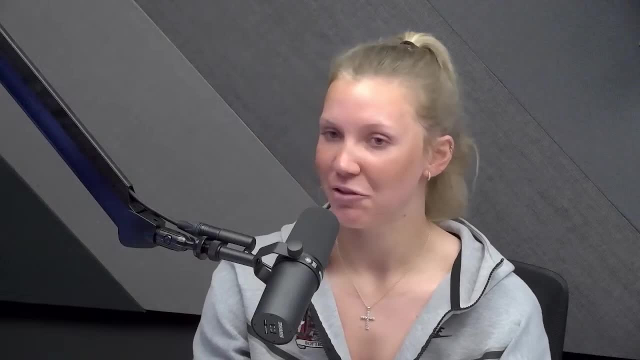 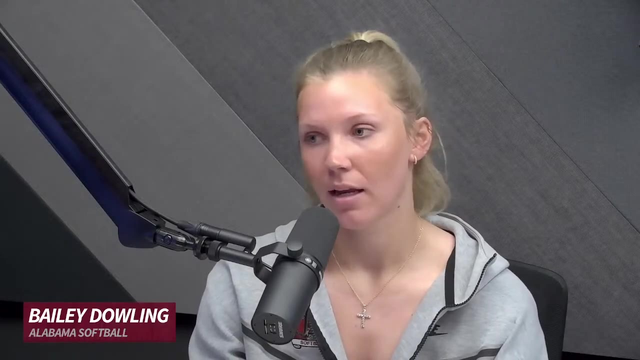 toes, because we'll have classroom moments and our um clubhouse are just on the field and once we're taught something, we're expected to be able to do it, and we're going to be able to do it. and we're going to be able to do it. 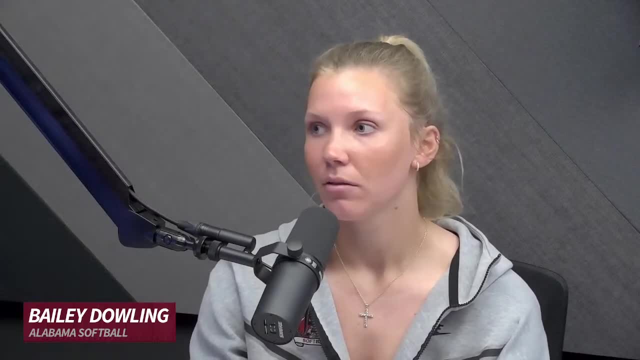 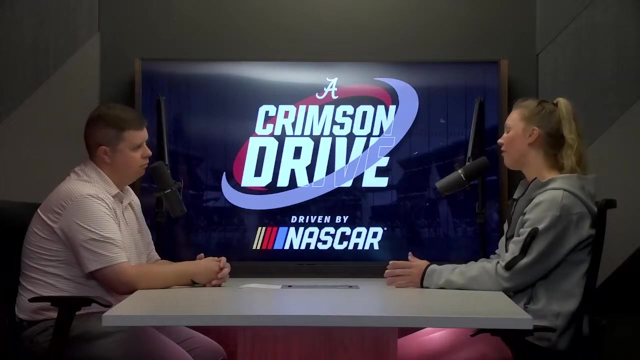 and we're expected to like, not, I guess, remember it, but like just know what you're watching or what you're listening to and, um, learn the game that way. so when we're in practice of Murph is teaching us something in five minutes, you better, you better, remember that or at least like understand what. 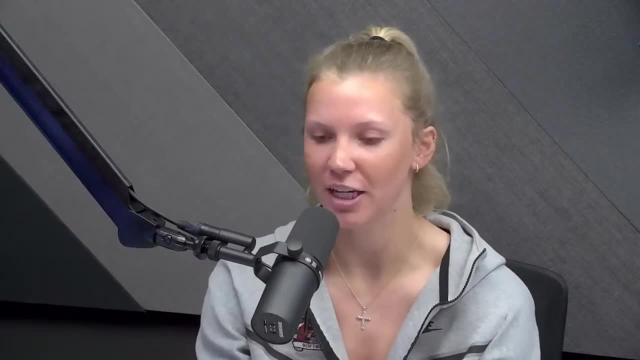 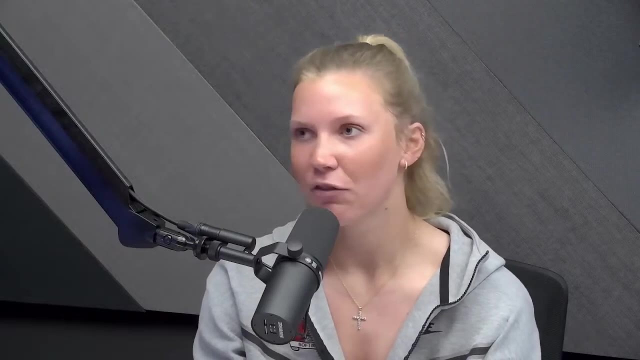 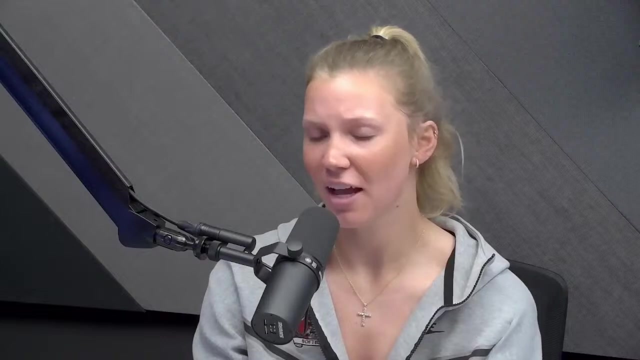 he was talking about, if that makes sense. so he knows you're always paying attention and so when he had talked about mudita and a couple other things like being a servant leader, I never fully understood, like it just never really hit me. so I wasn't thinking on my toes quick enough because 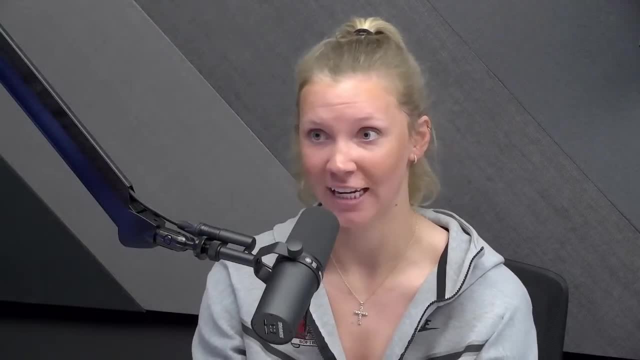 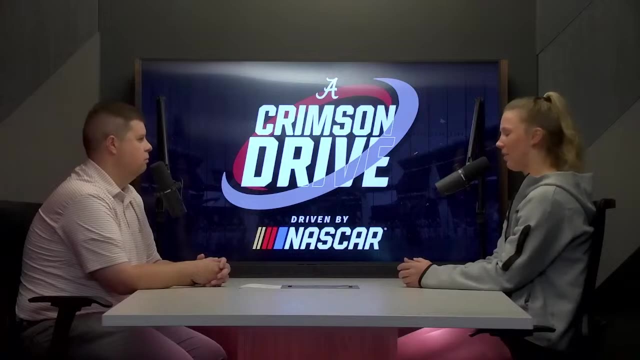 I'm in high school or like middle school at the time and I didn't understand that that's just how you need to be, you know, when you get older, like that's just a responsibility, you know thing. and so then when I got here I was like, oh, like I need, I need to know. 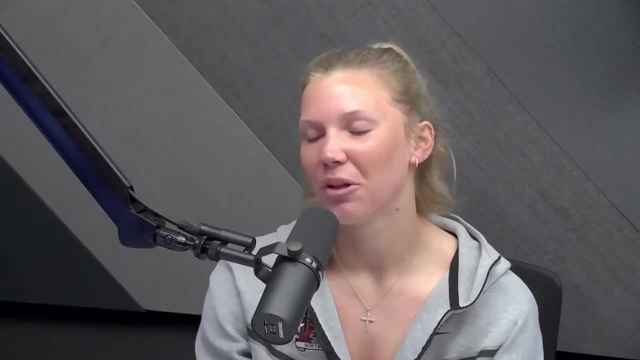 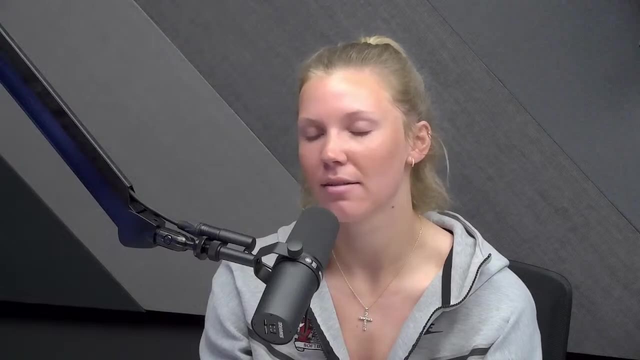 all this like okay, but yeah, no, I think that's just really cool, that that that's been around for so long and then that's a part of our um, our family here and just part of this program, because that's what makes it good again. it's about having joy and other success have. 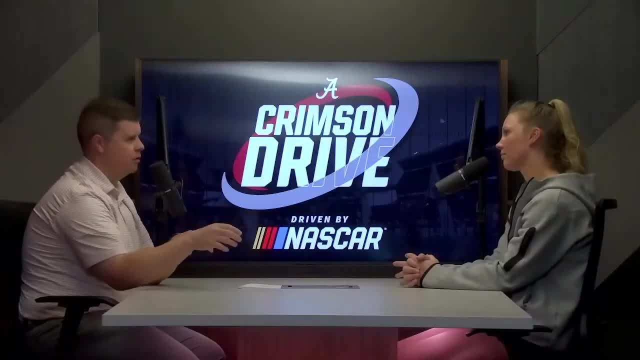 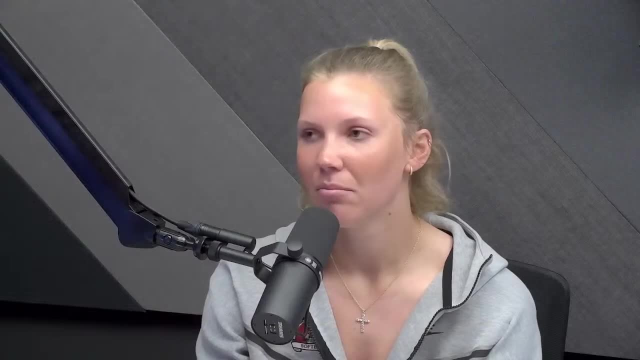 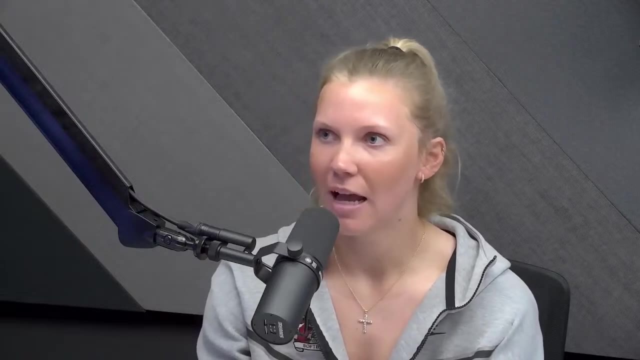 there been moments where you've had success and you really feel the mudita from certain teammates. any time that's really come up in your career. oh yeah, there's. there's a lot of moments, honestly. um, a couple of them are from freshman year and then some of them are from last year, and there's been 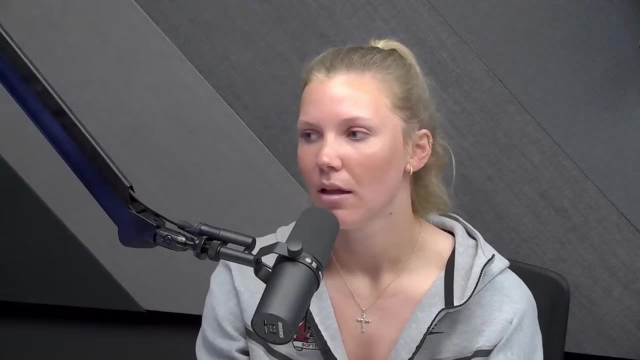 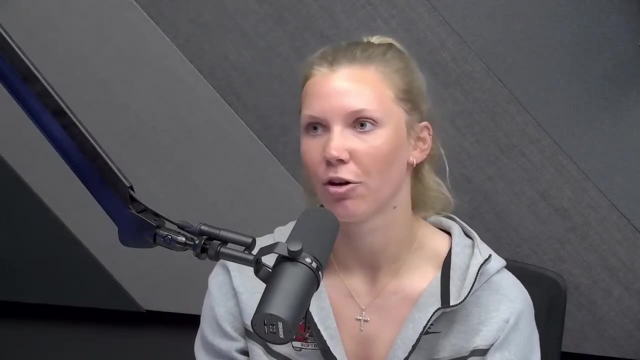 a couple this year too, but one of them is from last year and there's been a couple this year too, but one of them I really remember was, um, when we played FSU at Clearwater last year- um, it was the beginning of our season. it was kind of like opening tournament ish, and Kenley Cahalan had 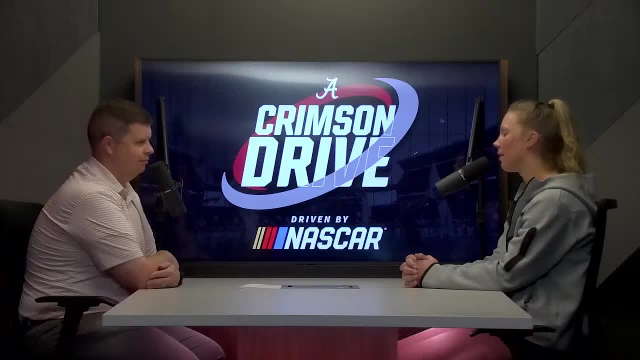 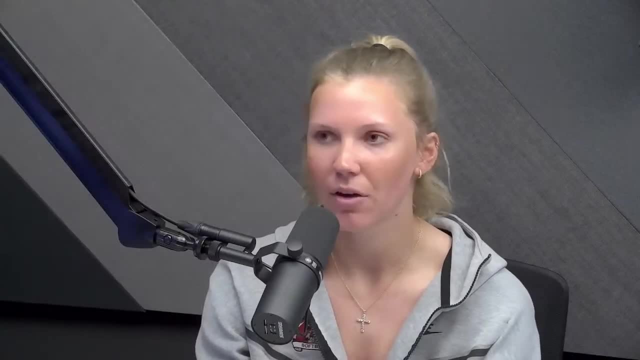 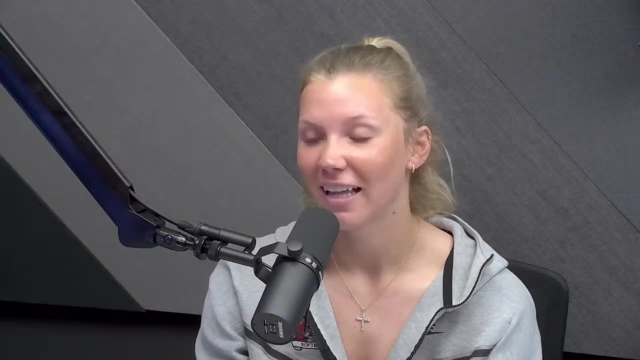 just hit a home run and we were up by one and that whole tournament I just wasn't, wasn't doing my best or how I normally would do. and then I got up to bat and I hit a home run and without that we wouldn't have won. and in that moment I remember just- and there's pictures of- 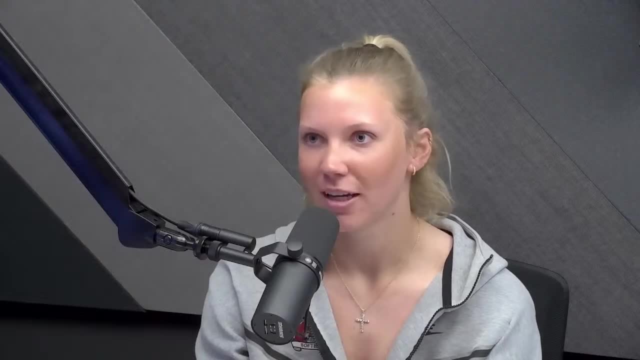 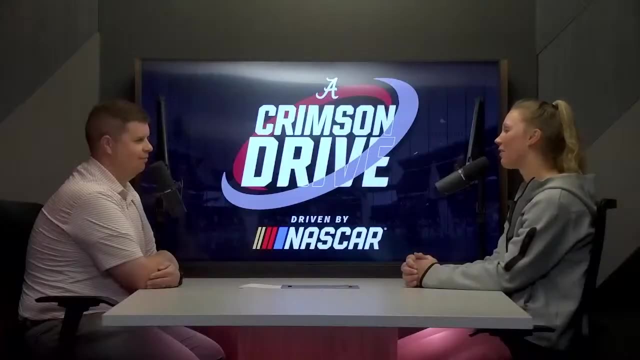 it too, but just every single person and everybody who had helped me get there to that point, it was just. it was really cool to see that and how they supported me and just their excitement, and that just again shows what this program is like. yeah, great moments all throughout that 2023 season and 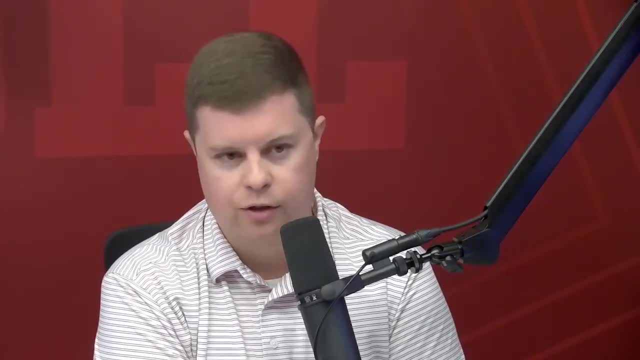 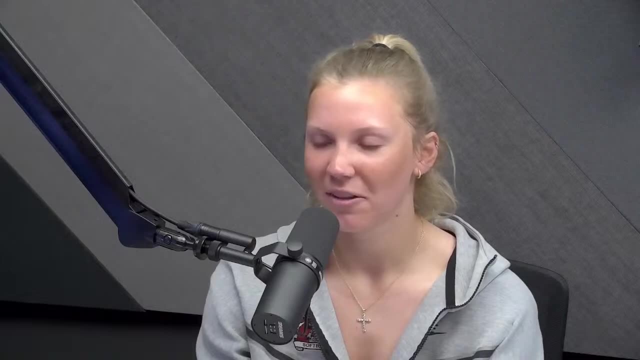 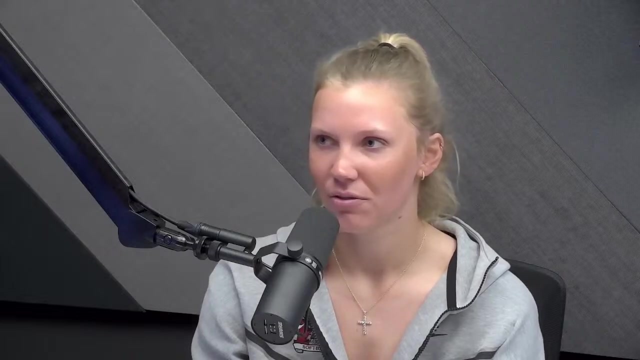 obviously the Montana injury in the SEC tournament, but able to come back for the regional, the super regional, how meaningful was it to punch your ticket to Oklahoma City for the World Series? it was awesome. honestly, I really don't have words for it, because our season was such like just a wave like we never we'd have good times. and then next thing you know, like 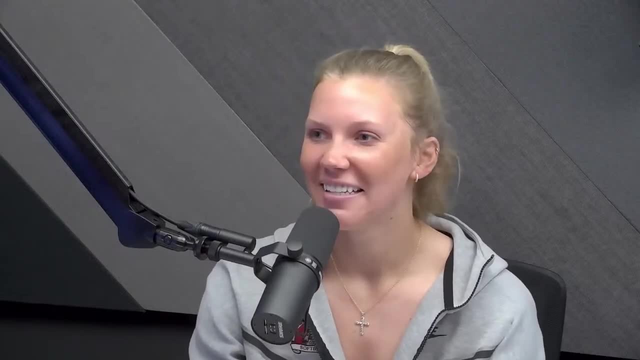 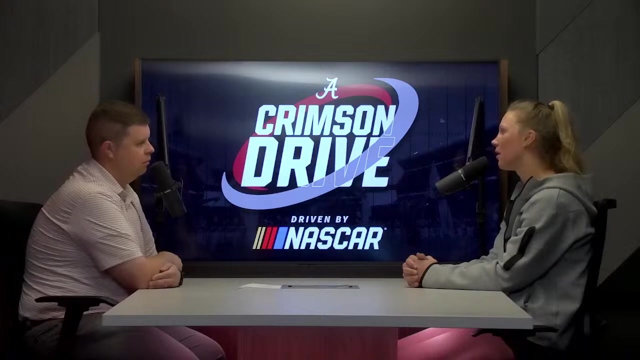 we're, we're down, at the bottom of the wave and so just being able to go to the World Series and the fight that that team had, nobody gave up on each other and you know, especially through regionals and Supers, because overall, like each person had their moment. 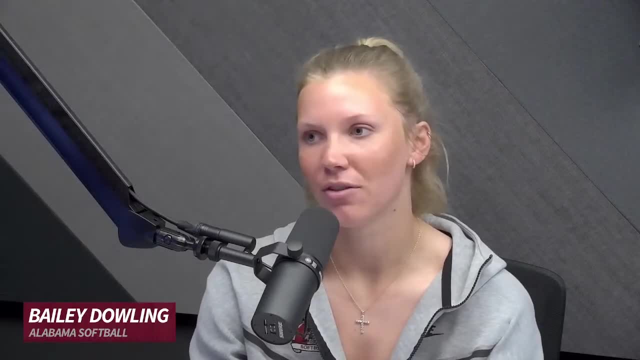 and we stuck together as a team when we could have just been done and I think that just showed a lot- and especially for our senior leaders at the time- like having Montana just fight through that. it was a really great experience for us to be able to watch and just have her, as a teammate, show us like what. 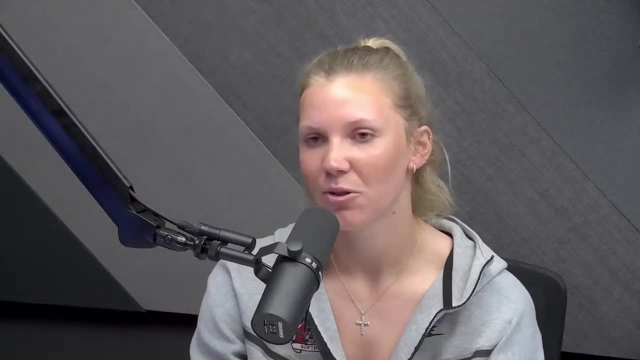 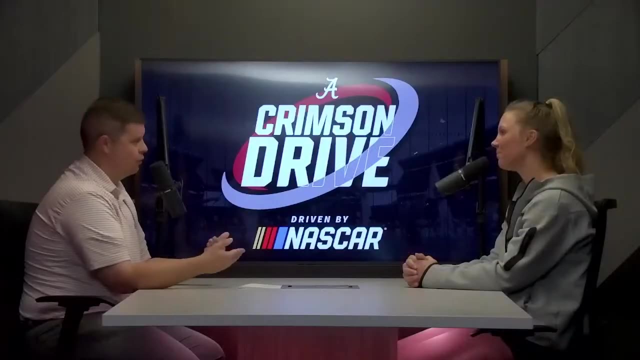 facing adversity is and like how you take it on. so I thought that was cool, and for you I mean it had to be. you talk about fulfilling a dream: getting to play for the Crimson Tide in the first place, but how about at the World Series? I know those games didn't go the way you wanted, but just 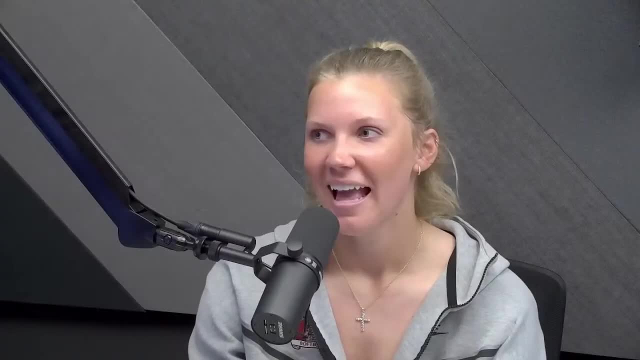 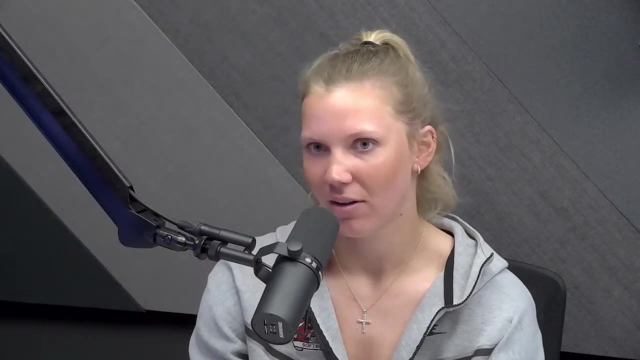 stepping into that Stadium sold out crowd. what that mean to you. it was very crazy because my freshman year we had went and obviously it was hurt, so I never got to do anything thing. the most I got to do was play catch with Claire, because she also did the same thing I did. 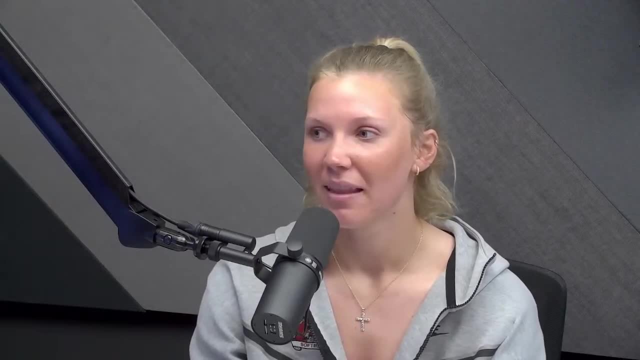 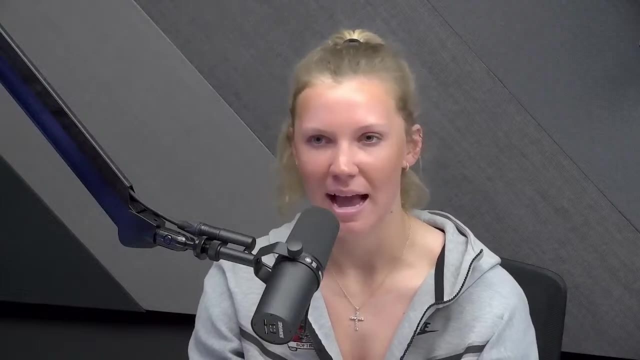 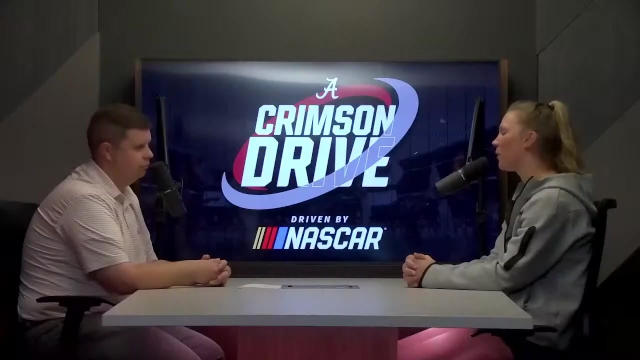 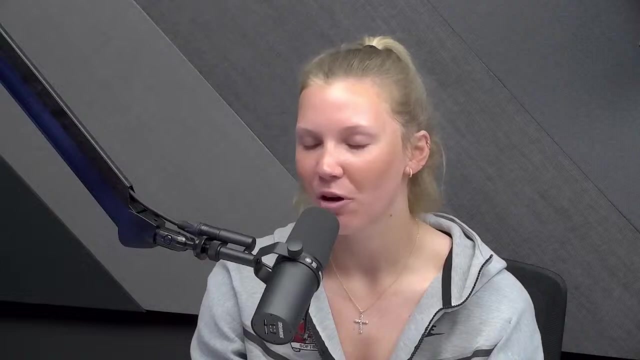 and that's all we got to do. um, and I remember going my freshman year and I was just like wow, but it never really sunk in because I wasn't out there, I just I wasn't playing, I was just there, you know. and then when we got back last year I was like this is every girl's dream. like I grew up. 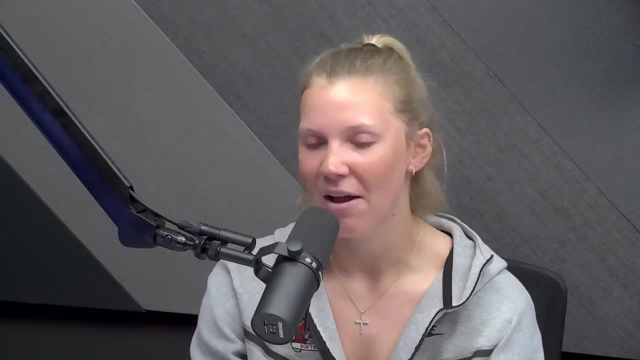 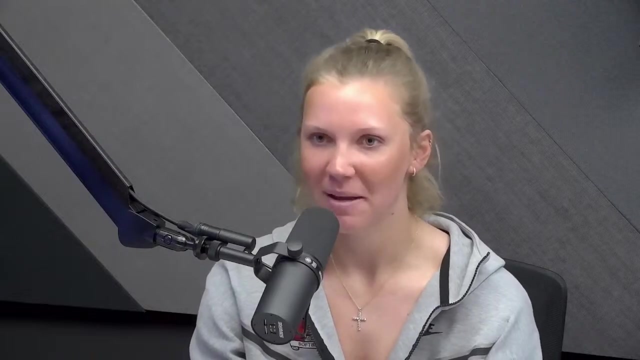 watching this and watching people get here and was like I want to do that and now I'm here. it was. it was just so crazy, because sometimes when we're practicing here at home, I'll just be in the dugout putting my cleats on, like wow, like I made it, like my dream came true, like I worked for it and I got. 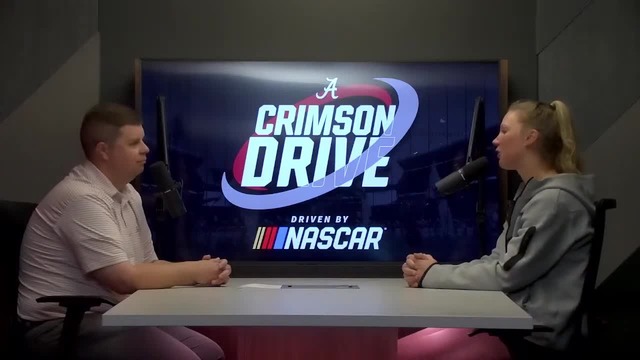 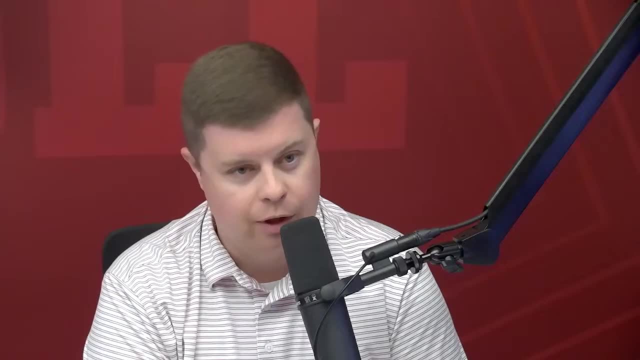 it and then the same thing at the world series. so I think it's just really cool and shows you know what hard work will get you mentioned before. uh, you hold the career record for Illinois- a high school home runs. you've hit a lot of key home runs here in your time at Alabama- a lot of great hits just. 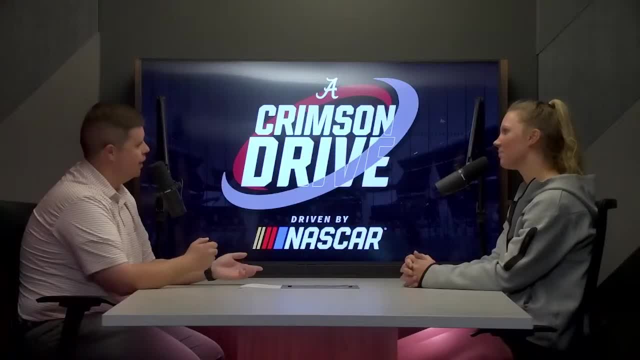 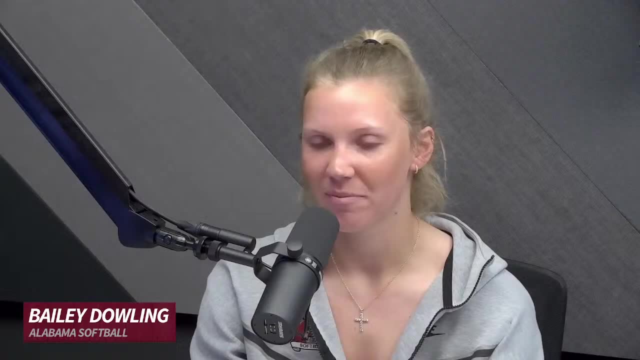 tell us about your approach as a hitter. is your swing pretty similar to how it was in high school? how's it evolved throughout the years? my swings changed a lot in my career- here for sure, just because of my knee and my sophomore year I was not close. 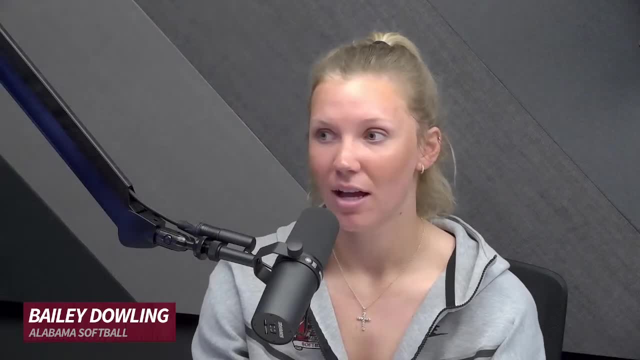 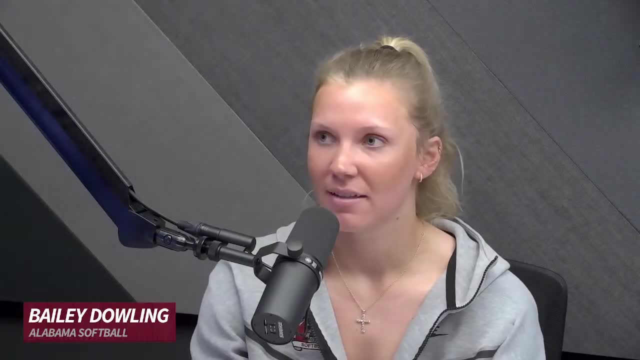 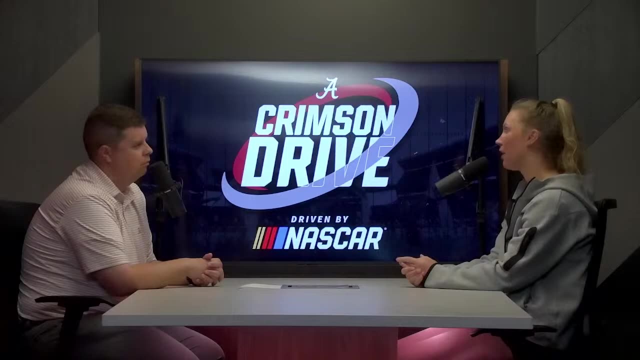 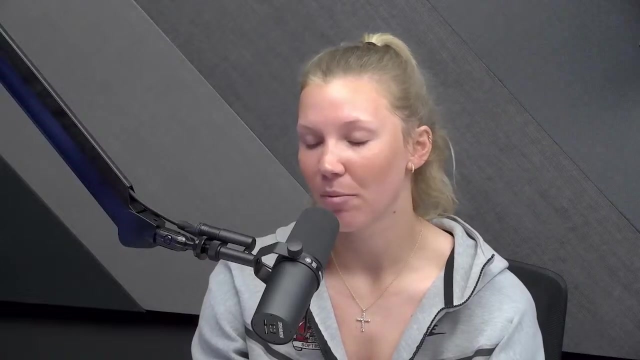 getting my knee to work and function, if that makes sense, and so my swing had to adjust to how I was feeling like day to day. if my knee didn't feel good, then I wouldn't be comfortable in my stance and it had to change, and so I never really felt like um. honestly, if you go back and 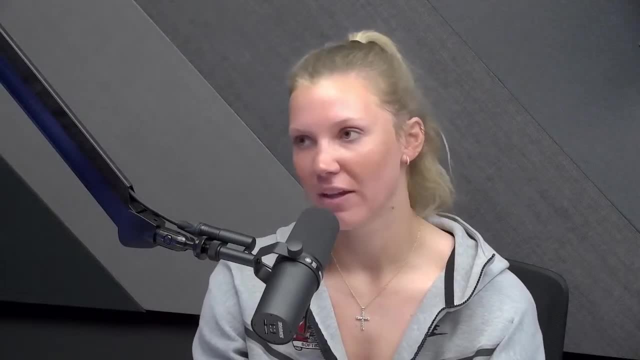 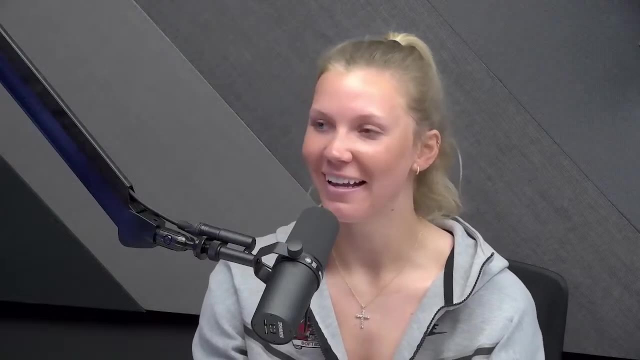 in my opinion. but it's definitely a lot more this year- like it was in high school, I think. So I mean that's good now. It at least looks a lot prettier. but as a hitter I shoot more for. 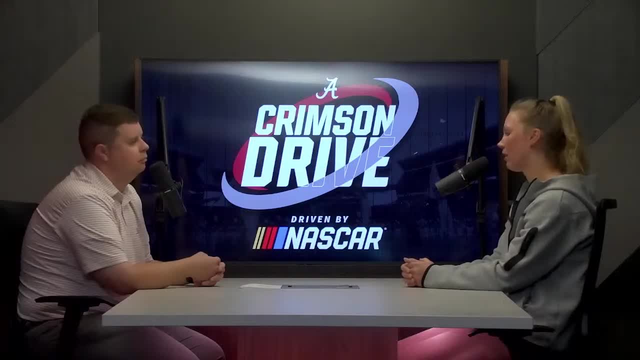 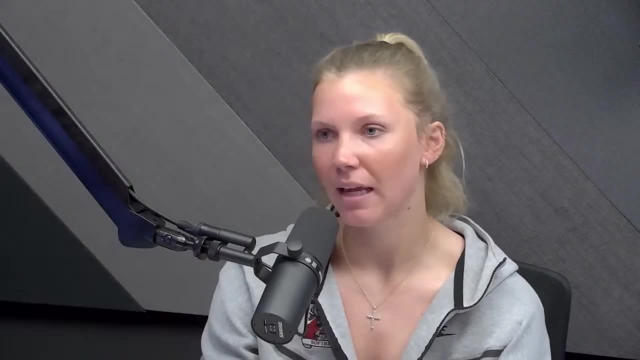 just line drives and like getting my swing off and hitting the ball hard on a line rather than hitting home runs, because when you get up there it's just between you and the pitcher. You can't be thinking about your outcome or like what you want to do up there, Like you have a plan. 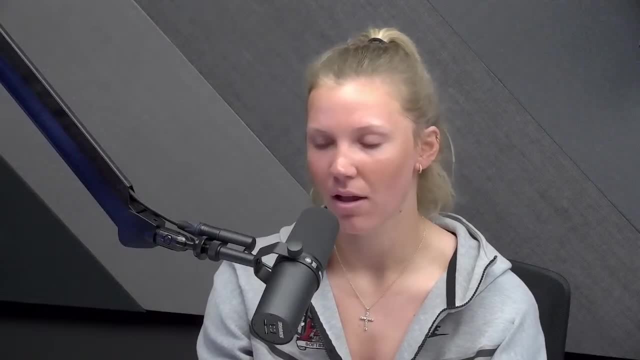 and when you step in the box, your goal is to execute it, Nothing more. So, yeah, when I get up there, it's really just to see a pitch that I can get my swing off on and like hit it hard. 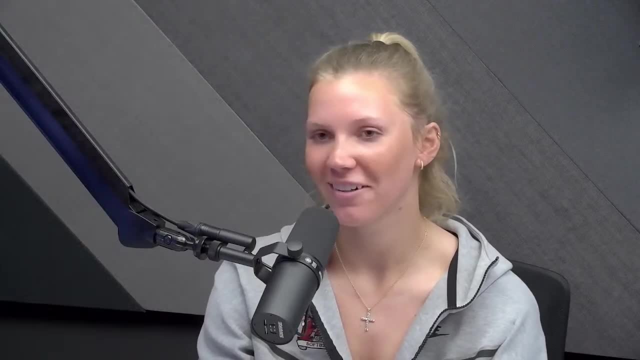 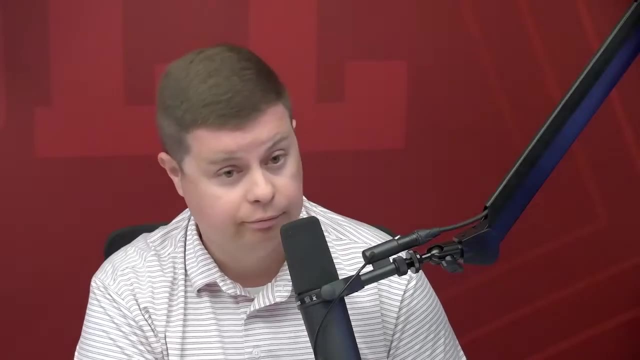 So- and I think that that's worked for me pretty good so far- So Absolutely, To get prepared for all these at-bats. how important is video study or some of the analytics that we're now seeing all over softball? The analytics part is really cool because you know now they're creating. 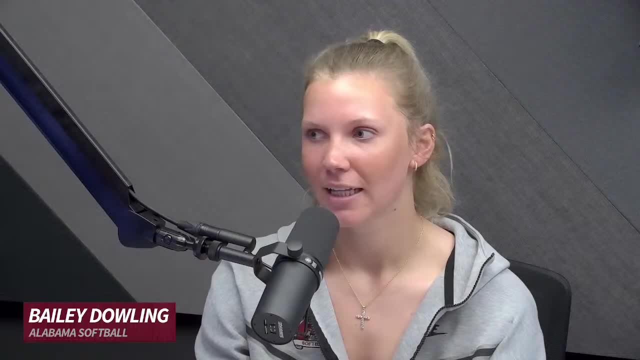 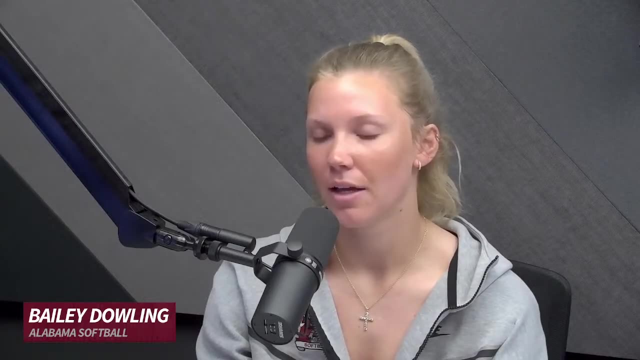 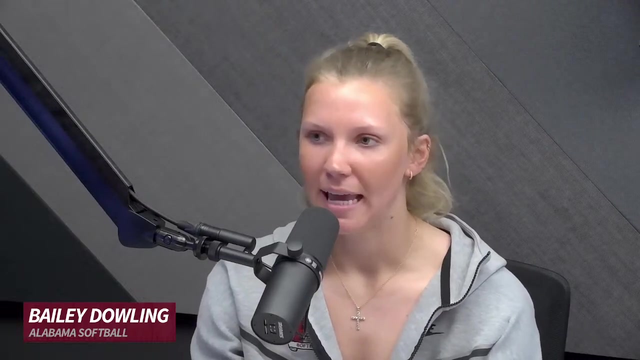 pitching machines that you can make. So I think that that's really cool and that's something that I utilize a lot just to get at-bats and like see pitches that I'm going to see in a game and figure out what plan you know I want. 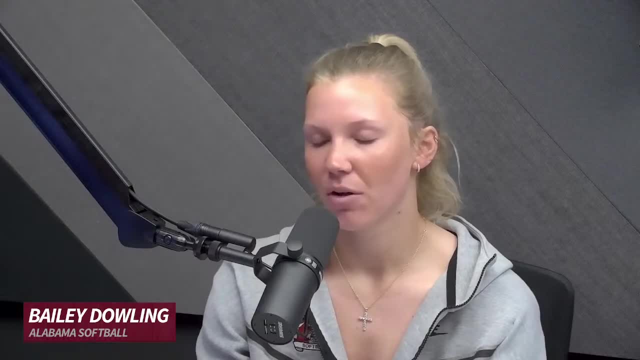 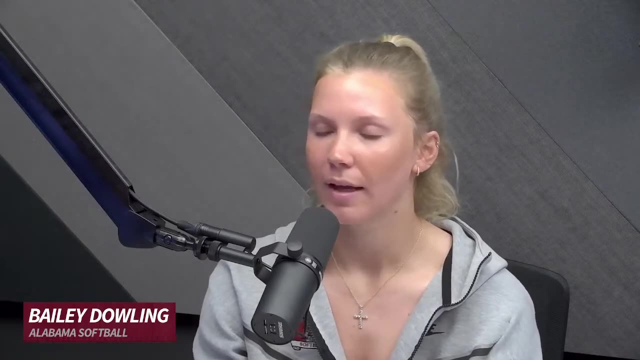 to take when I get out there. But that and just watching film and seeing how pitchers, you know, I guess, what their mentality is. So I think that's really cool, Like you can see that based on their body language and just how they go about. 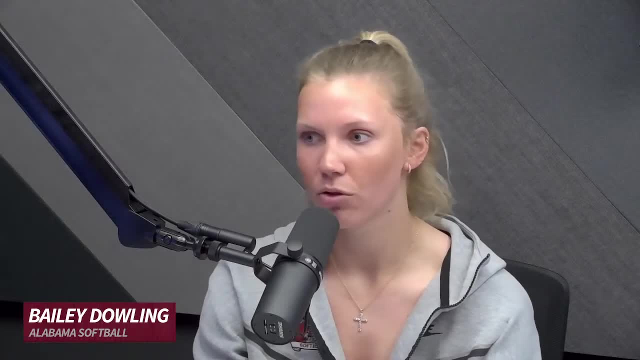 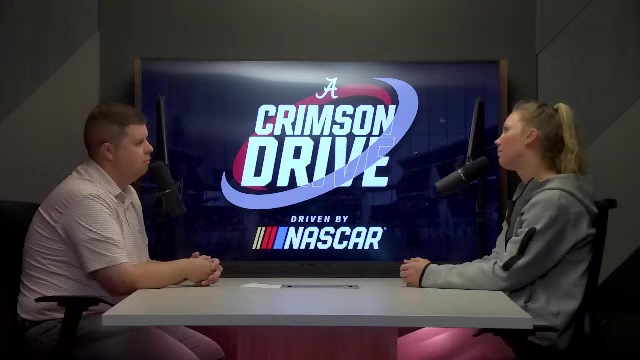 their pitches and like what's their best and what's their worst, And it's definitely very important at this age because you really have nothing else. You can't go out there like it's a travel ball and just you know wing it. So yeah, we do that a lot in practice and just on. 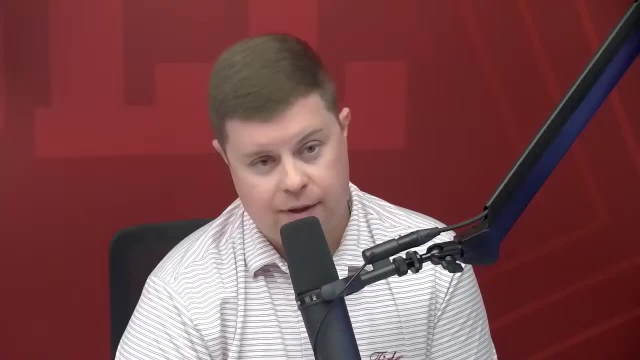 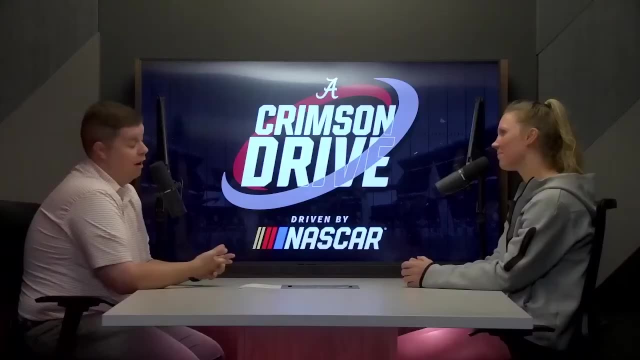 your own watching film. So So time on the road for the Crimson Tide. Crimson Tide this past weekend at Kentucky, but now you get some home games coming up at the Rhodes House, First of all against Ole Miss, Texas A&M. After that, just starting with the 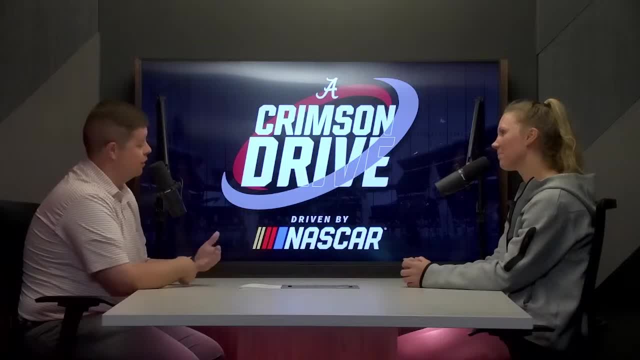 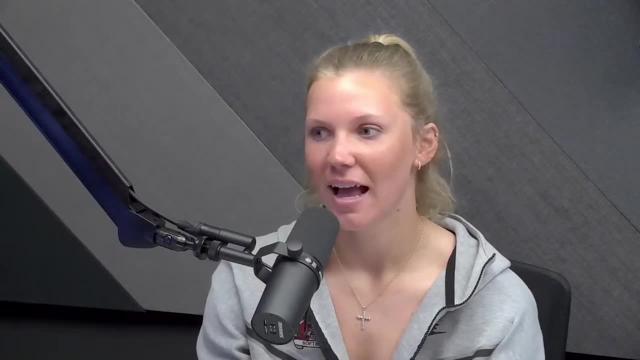 Rhodes House. what do you love about the home environment? What do you want to see from this fan base as you continue throughout your senior year here in Tuscaloosa? I love how packed it always is and just how when the fans are cheering you on like they are on. 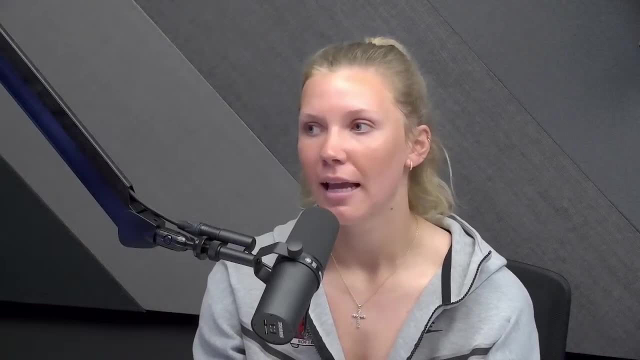 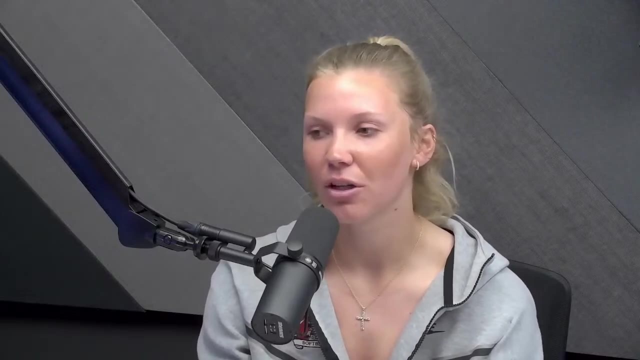 top of you And a lot of the stadiums that we've played at, it actually feels like they're on top of us, But once they're cheering like they are right there in the dugout with us. I think that's really. 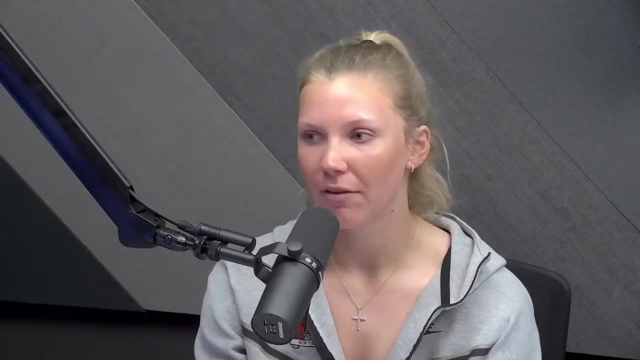 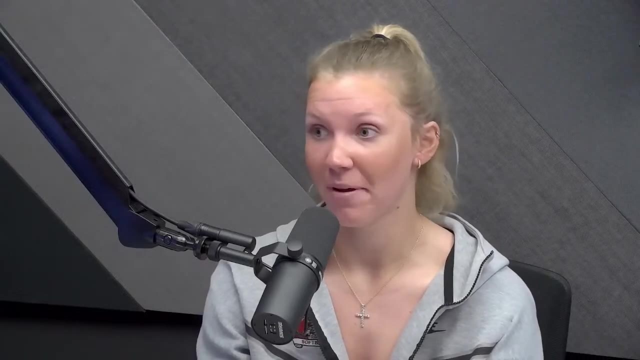 cool And we get a lot of fans. You know we have, if not the biggest- I'm not sure what Oklahoma's is now- but I think that we have the biggest stadium and we get the most fans, And so I think 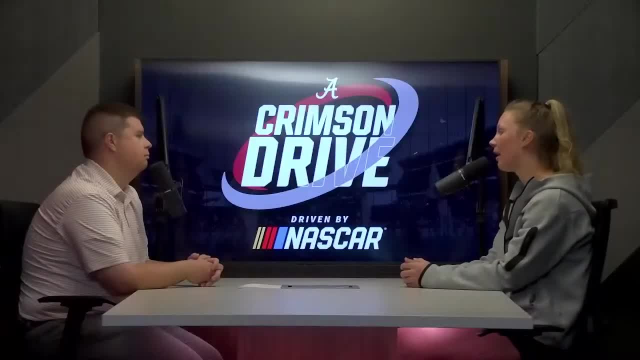 that that's really cool and just shows our support that we get. And so, yeah, I get really excited about that. when it's a packed house, because that's a big part of it, That's not a lot of teams get that. And when we get to Oklahoma, that's what it's going to be like. 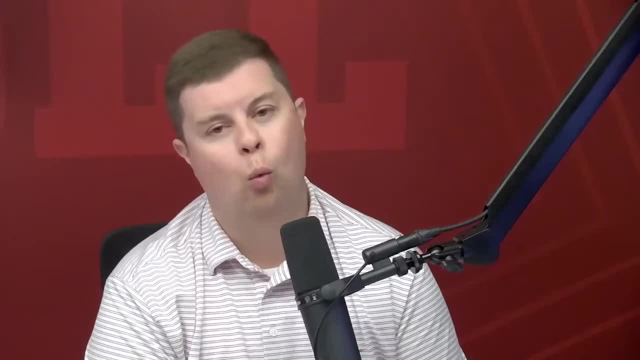 And so I like practicing it before we get there. That's certainly good. What is this team capable of? Obviously, it's been up and down through the first few weeks of the season, But as you get ready to start this month, April, what's going? 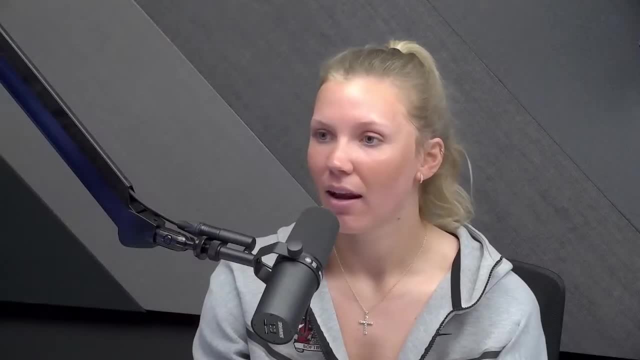 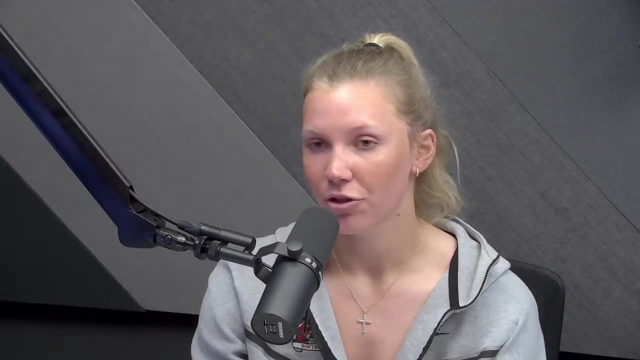 to be most important. Well, we have a lot of grittiness and we're never out of a fight. We always find a way to punch back, And so I think that that's really important. Just shows, like, who this team is and what we have. 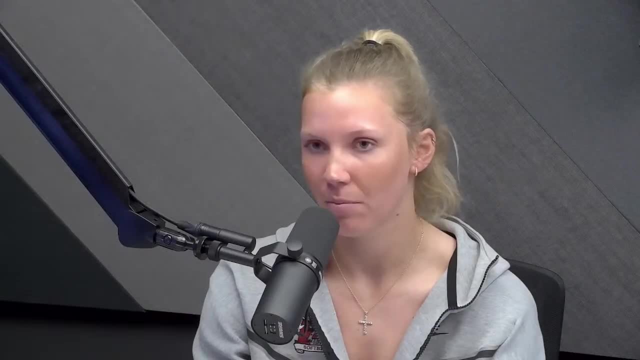 But I'm excited just to see how we bounce back from what we've gone through, because we keep talking about how we're going through learning lessons right now, Like we're always learning something from what we're going through, bad or good- And so I'm excited to see how we utilize 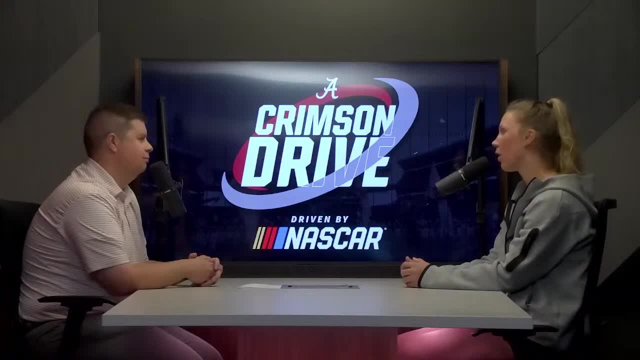 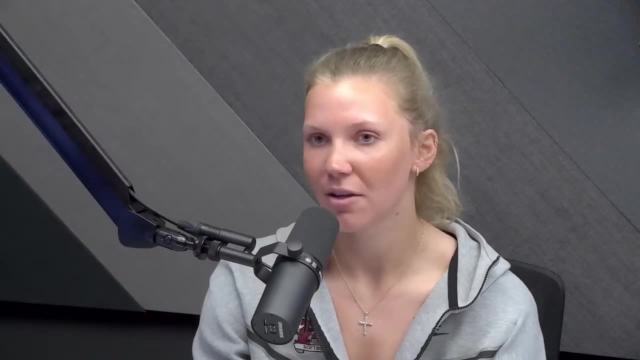 that and just go about these next couple of weekends, because we are at home And so we get a couple of good practice days before we play. And, yeah, I'm just excited to see where that takes us. We're fired up as well. Bailey Gowling. 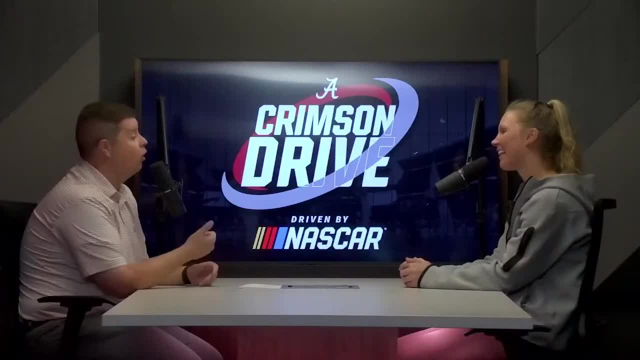 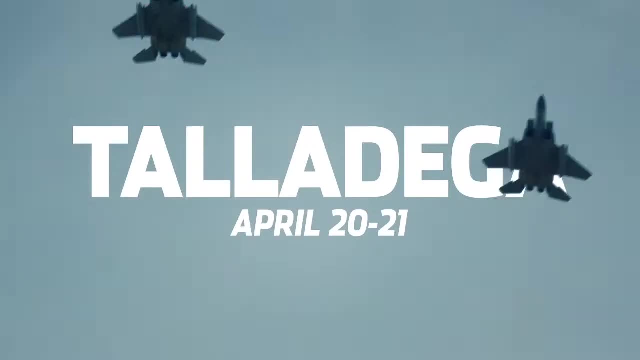 Thank you so much for your time with us here today on Crimson Drive, driven by NASCAR. All the best to you and the softball team the rest of the way, Roll Tide. Thank you, Iron Maiden's place. But in order to take it all home, you need nerves of steel. 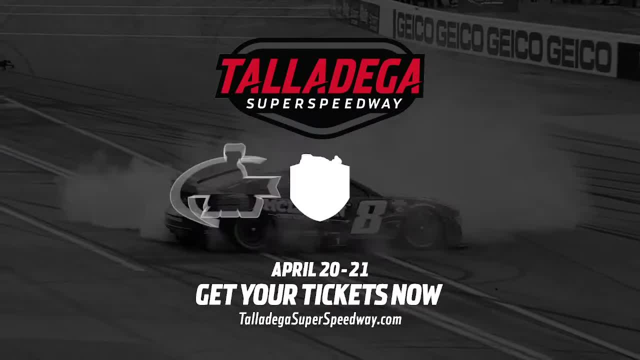 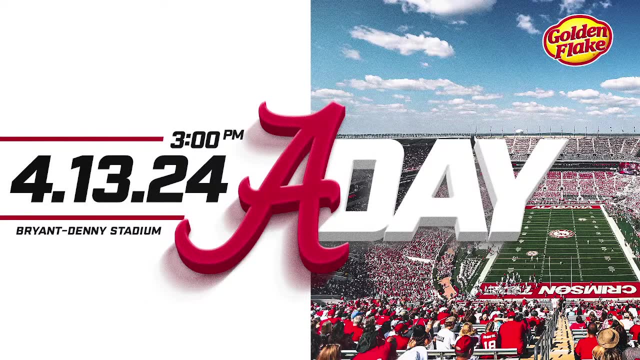 The big one is back. Get your tickets now at TalladegaSuperSpeedwaycom. Fans looking to enhance your pregame A-Day experience, visit Champions Lane next to the Walk of Champions from 11 to 3 pm on A-Day, April 13th. 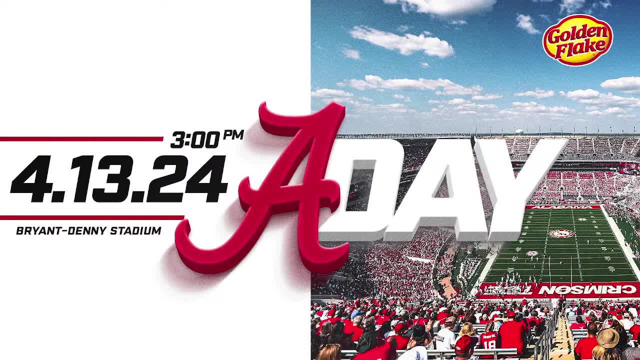 Champions Lane is free and open to the public and will feature live music, A display of Alabama football trophies and awards presented by NASCAR and Everwood, Autograph signings with current Alabama student-athletes and former Alabama running back, Trent Richardson. We'll also have 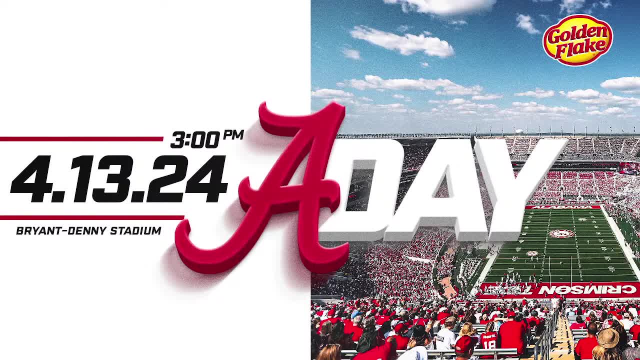 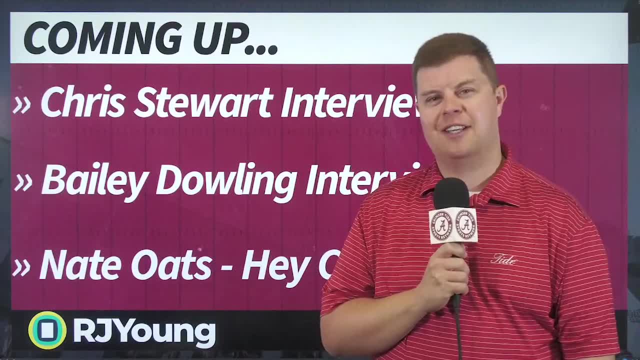 a NASCAR pace car, food trucks and other interactive displays. Visit ChampionsLanecom for more details. So from Brian Denny Stadium we go to Baumhauer's Victory Grill here in Tuscaloosa where, on Monday, we really had a party. Yes, we did have, of course, Hey Coach. presented by Alpha. 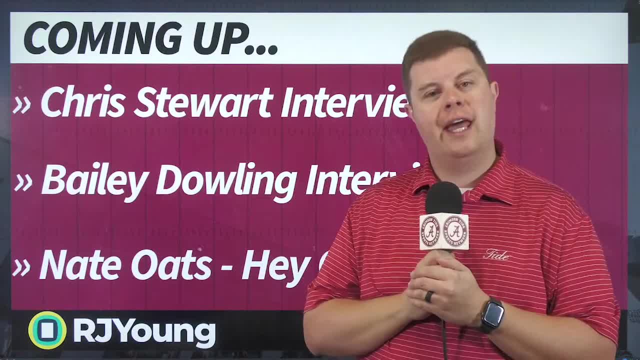 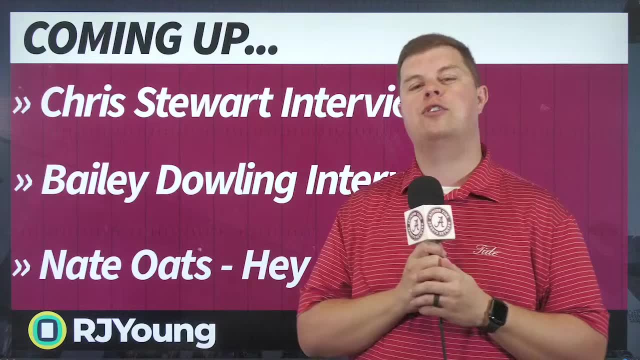 certainly a Final Four preview show, as Chris Stewart had the chance to interact with some members of the men's basketball team, and then the head coach of the Crimson Tide, Nate Oates, who brought along a trophy: the NCAA West Regional Trophy from 2024.. And we hope there are more. 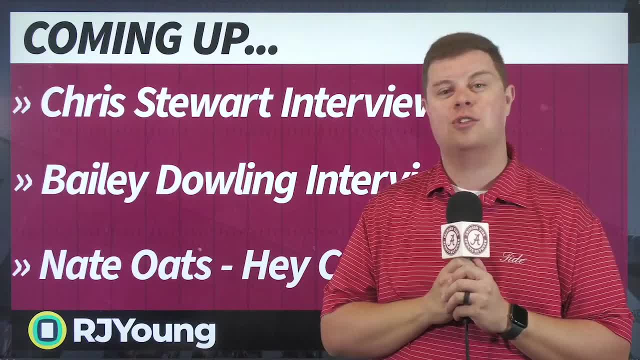 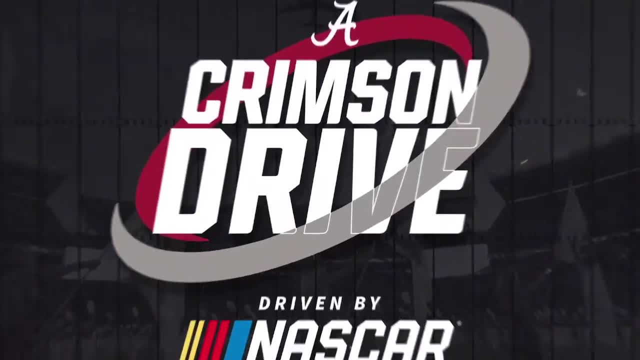 trophies in store coming up for Nate Oates, But here's a look back to his conversation with Chris Stewart talking about the wins over North Carolina and Clemson and looking ahead to Alabama in the Final Four Five years ago tonight I am told we sat here and did this show. 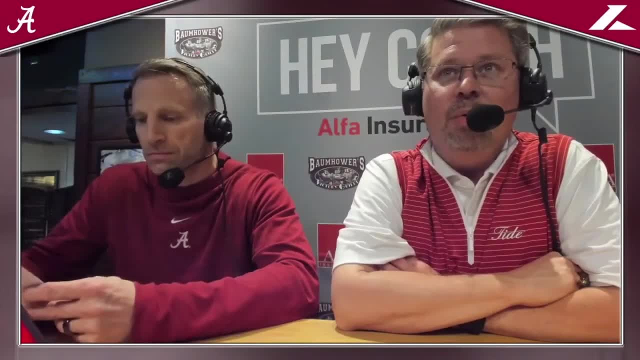 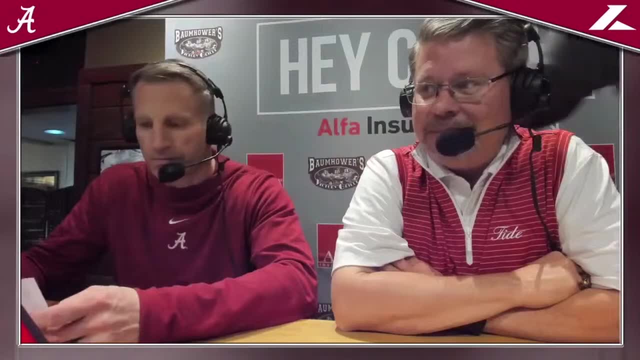 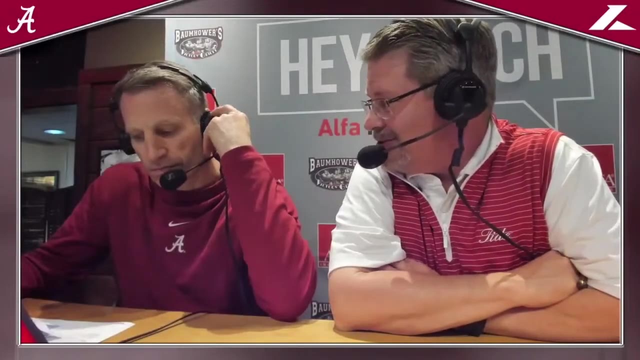 and a new guy named Nate Oates got a very warm round of applause as he came in and sat down and joined us. It was a pretty big round of applause back then. It was even bigger tonight. a standing O. You've actually earned this big applause tonight, Coach. Congratulations. First Final Four. 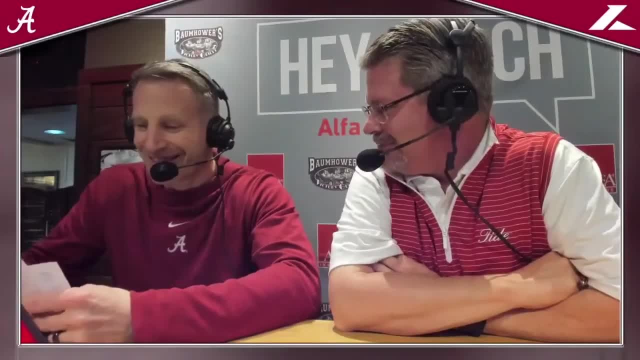 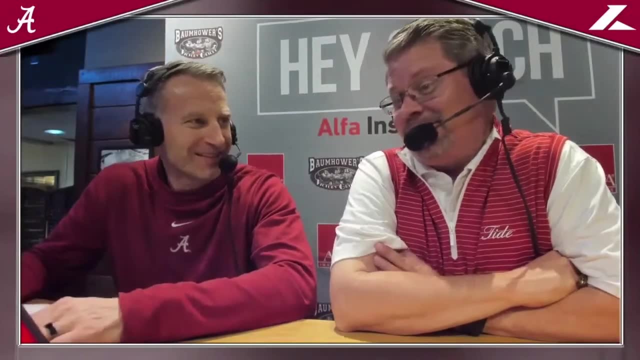 birth in school history. Hard to believe, Yeah, a little crazy. Five years, It's been five years, Amazing. Took us a while to get here, Finally got here, though It took us a lot longer Than five years to get to the Final Four. Coach, We're here. You've done your part. 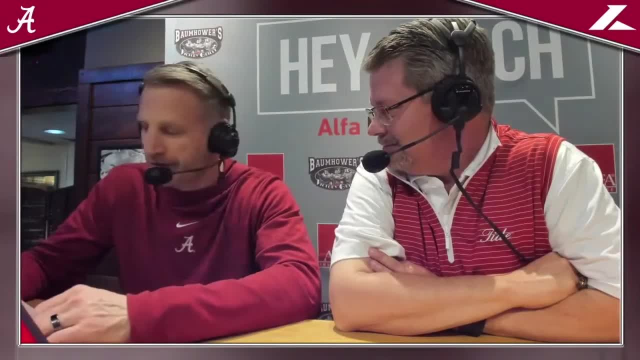 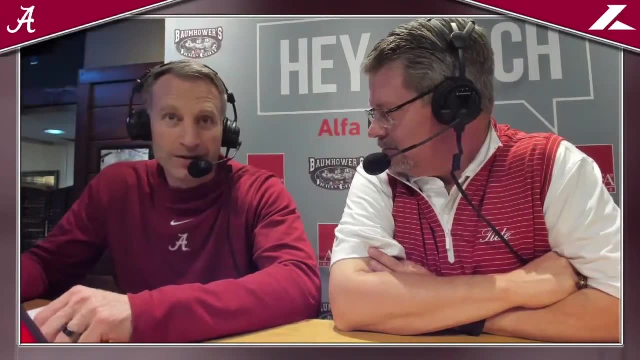 Yeah, we- you know it's hard to get there- Shoot. we've had a few teams that could have made it. We finally got here. Our guys have pulled together at the right time. We're playing our best basketball in March, like we try to be Shoot. it's amazing. I mean we've got. 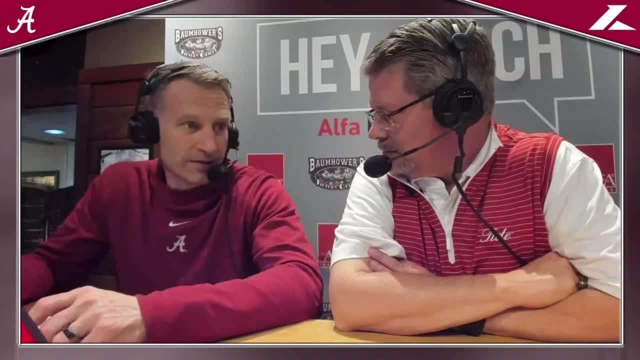 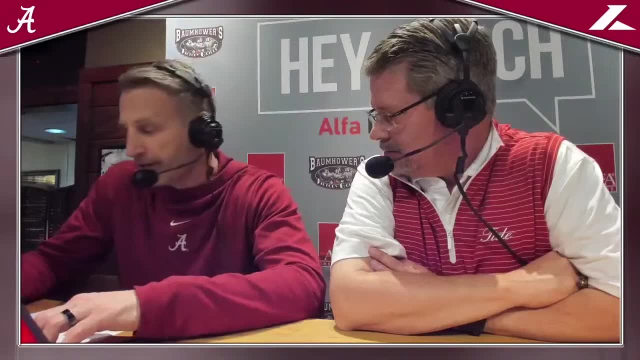 contributions from all different people to get us here. You know you go from that Grand Canyon game when Diabate came in. You know we were down about five minutes ago and Diabate came in and made big plays for us. We got. 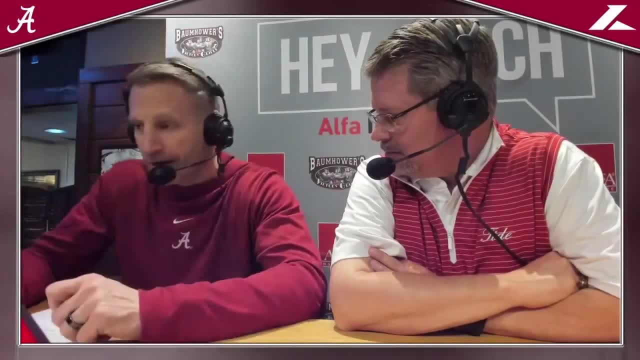 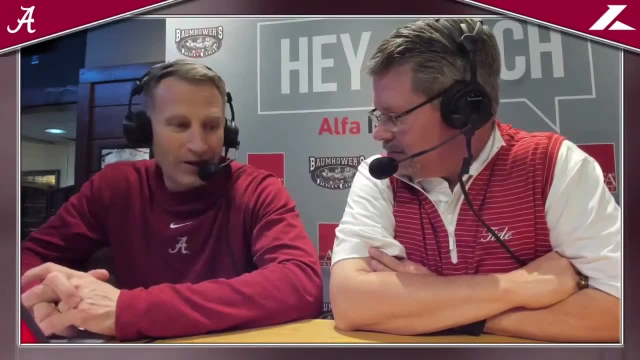 to win and thought our guys really kind of rallied around him. You know Sears made the point: we don't win this without him. And then the next game we get to play North Carolina, where Jaron's from Chapel Hill And you know I was hoping he'd have a great game and he was solid for us. But 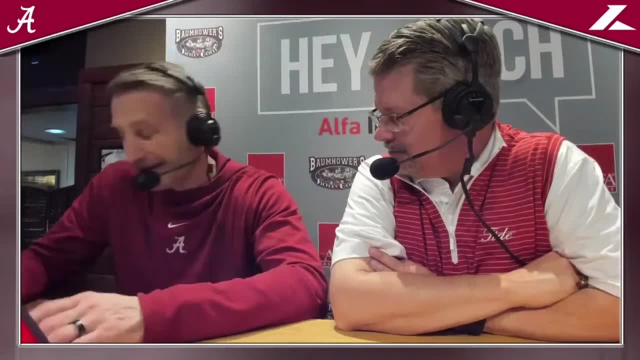 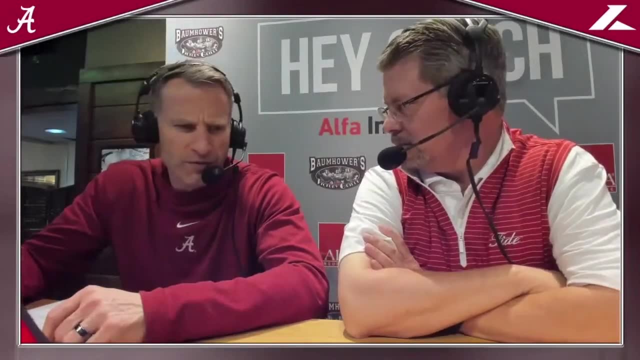 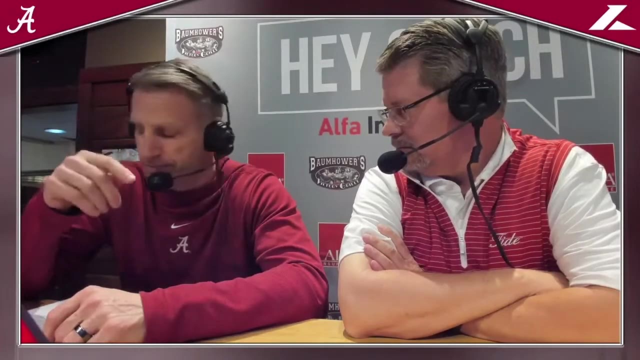 you know we had Grant step up and had a huge game. I mean there's the 24-12-5 with his five blocks, I guess 24-12-5 against a single-digit seed. There's only been four players in the history of the NCAA tournament to do it. He's in pretty good company, Shaq. 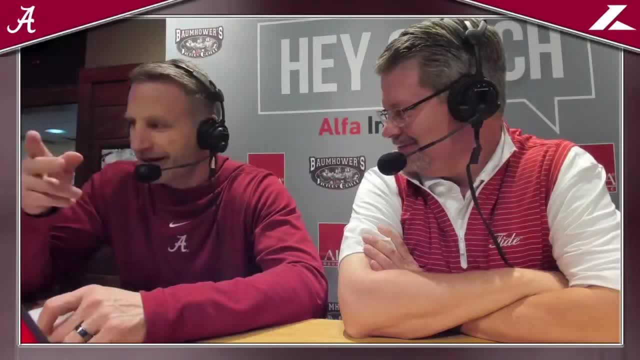 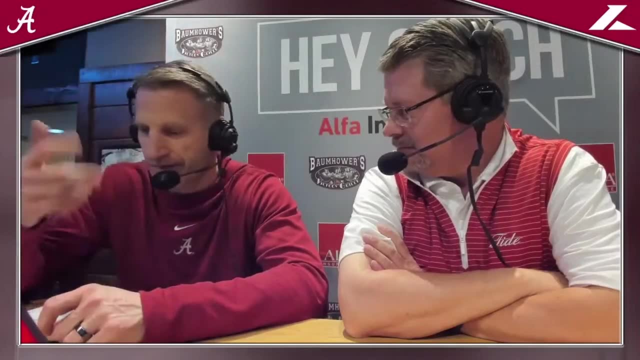 pretty good player: Shaquille O'Neal Shaq, And Tim Duncan not a bad player. He turned out all right. And then Channing Frye, So it's who played in the NBA a long time too. So Grant Nelson, Channing Frye, Tim Duncan, Shaq, the guys have done. 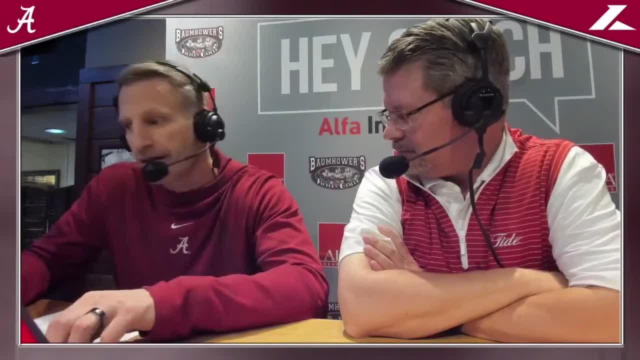 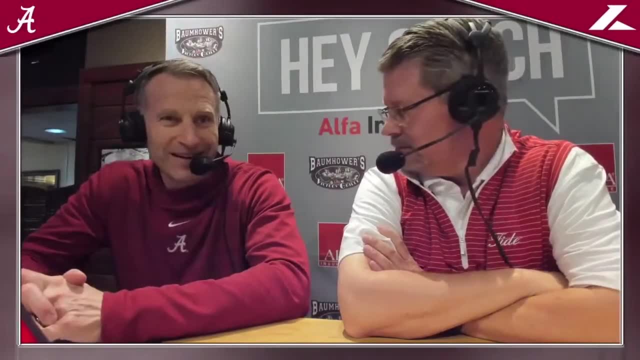 what he did against North Carolina. Not a bad program, but do it against. And then Jaron stepped up for us the next game in a huge way, at five of eight threes and at 19 points. Did not look like a freshman and you know. 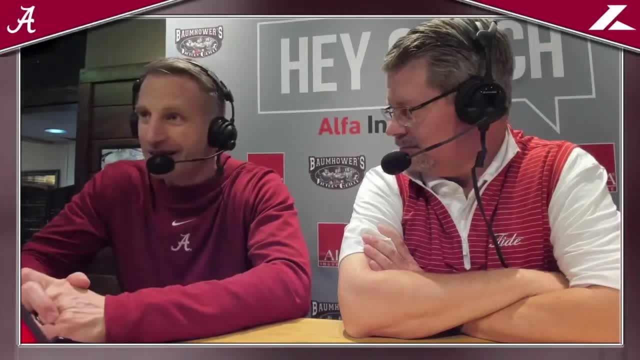 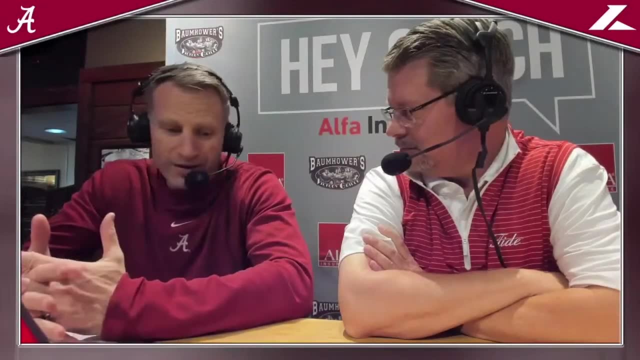 looked like he grew up a lot to get us to the Final Four And I mean I didn't realize until today. I was looking. you know, I try to move to the next games in this. Ryland. as good as defense as he played and as many shots he hit. Ryland had eight assists in our 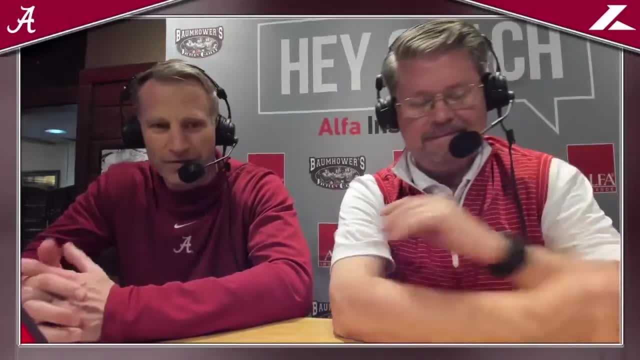 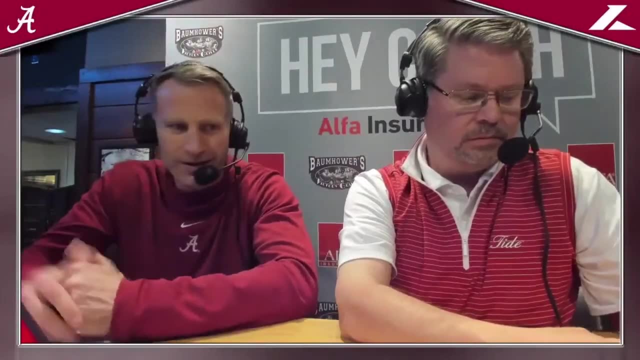 last game, which that passed me up until we were in video today, And I just kept seeing we were going through that. We kind of pull our blue collar plays and our highlights league. We do every game to kind of reiterate what we're looking for. And also, I just kept seeing 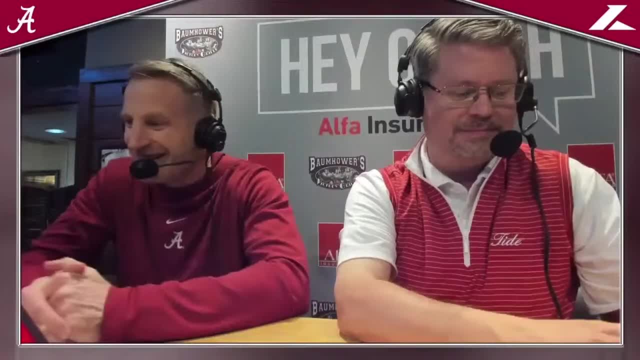 Ryland's pass shot, pass shot. I'm like, how many assists do you have? You know he had eight assists. So it's like different guys you see stepped up. I didn't even realize in the game some of the stuff that the guys did. 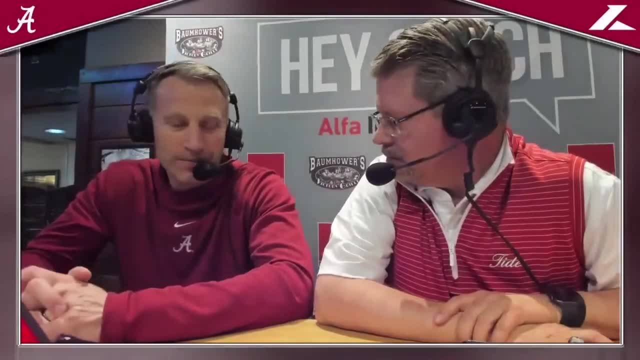 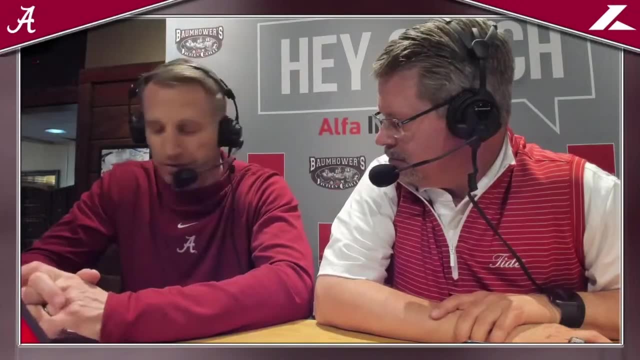 But yeah, we had some guys really step up. You know, Sears leadership's been as good as it's been Nick Pringle's leadership stepped up. I mean he man, he had double, double, double digit rebounds, multiple games. I mean he's played well for us. So different guy, you know. 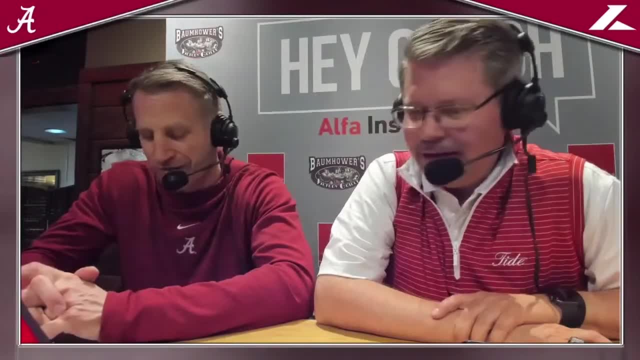 who knows who's going to step up. We're going to need a lot of guys to step up against UConn. They're pretty good, But we're here, We're playing. There's only four teams left playing and we're one of them. 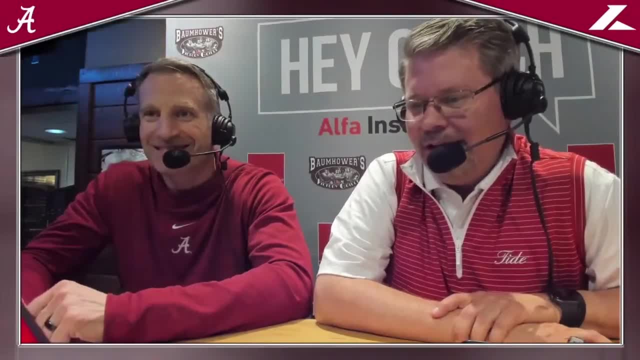 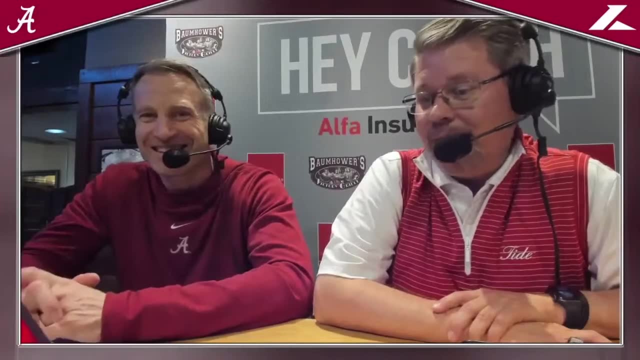 It's amazing You talk about all those guys- And I was guilty of doing this on the radio broadcast- but we almost forget at times. oh yeah, by the way, that Mark Sears guy ain't bad either. The West Region most valuable player: 23 points. 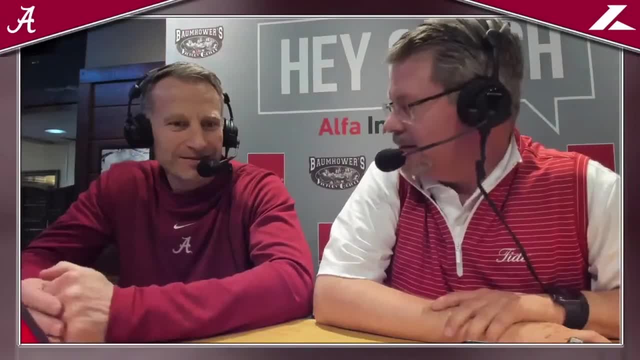 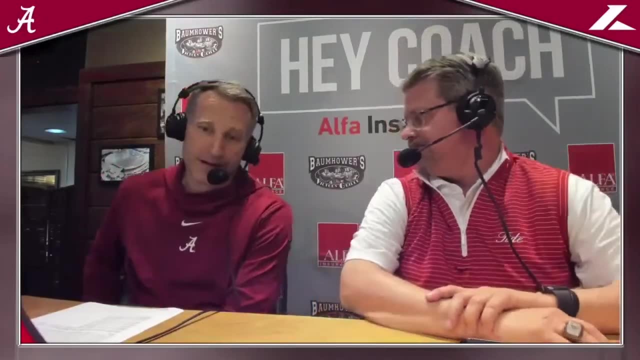 He just he somehow finds a way to get to that number, or close to it, every single night. But his game has become a whole lot more than that, hasn't it? Yeah, I mean he, like we've said it, kind of he can almost sleepwalk his way to 20 points. 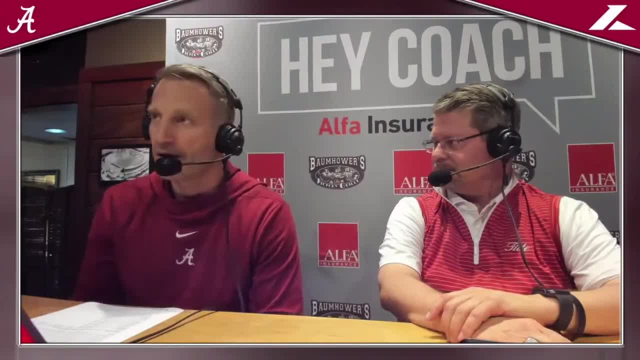 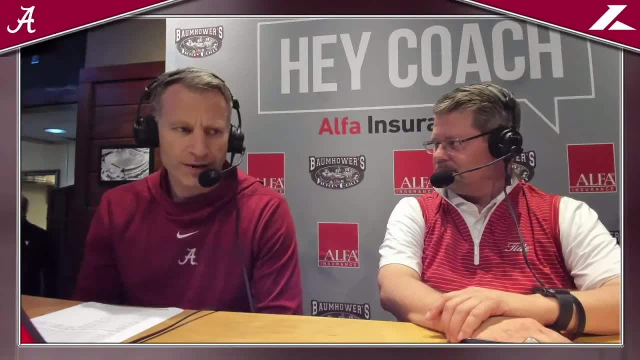 I mean, he's got a bad game and ends up with 20.. You know, and he this last game he was a little frustrated. What did he miss? his first seven shots Or something like you know. he came over. He's a little frustrated. I'm like like Mark. 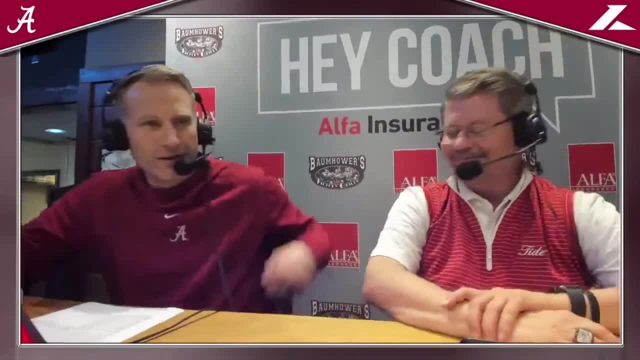 you'll be fine, Like you'll get to your 20.. We're going to be good Like get an open shot, You're going to hit him, You shoot. Who knew he was going to hit seven threes in the second half? 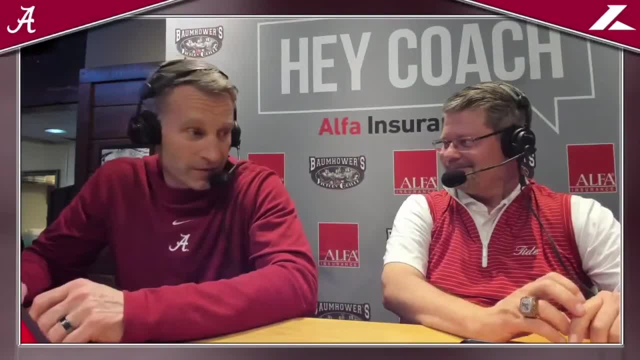 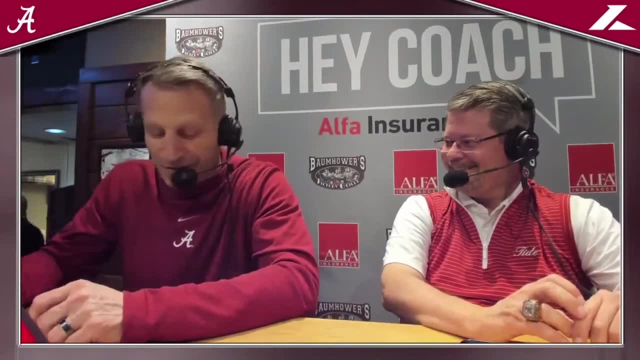 I mean he came alive and like, shoot that one, he hit from deep. He was at the logo, He was. It was a little like Dame Lillard Steph Curry range back there, But no, I mean he's. 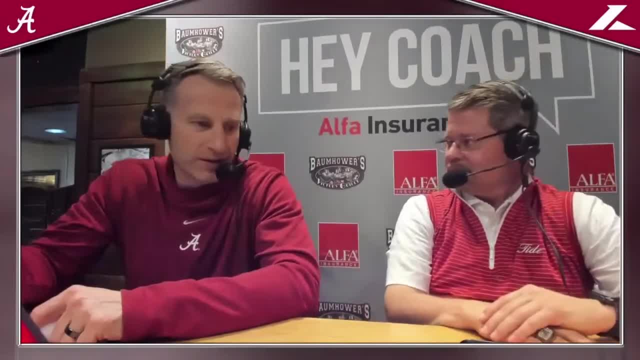 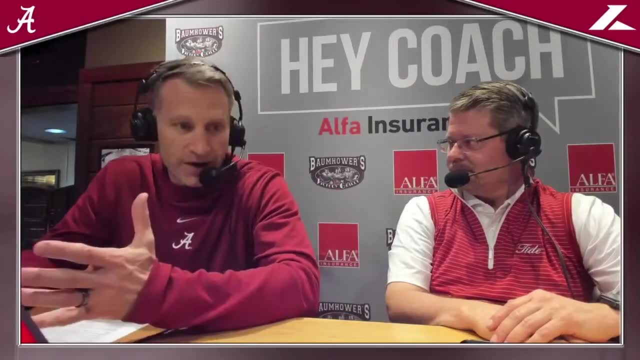 he's been. I think people around here have gotten used to the fact that he can scored at the level he does because he's just been doing it for so long And he had, whatever it was- 20,. what is he? 23 of his last, 25,, 22 of his last 24.. He's at 20 points. 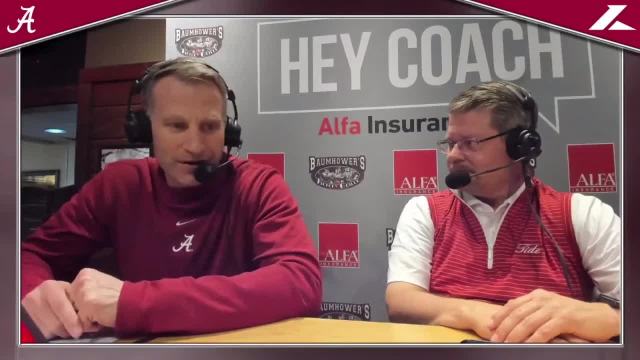 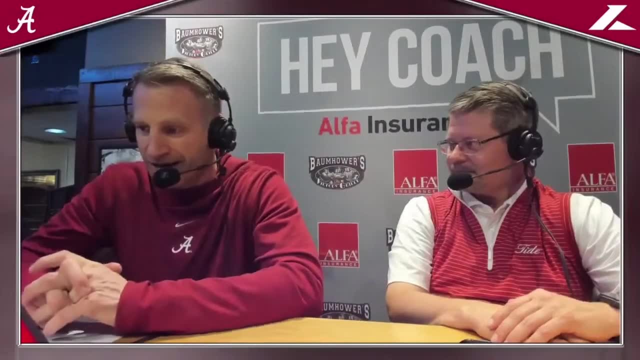 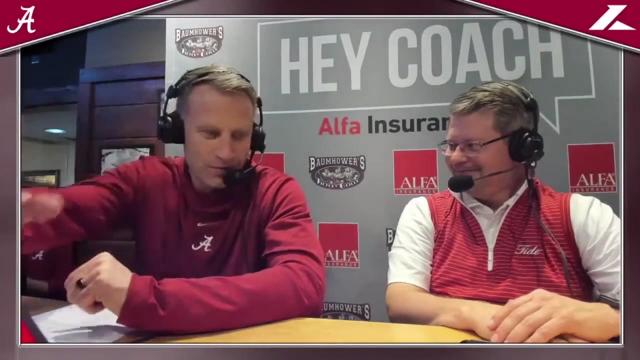 something crazy like that. So you know, and he's from Alabama, you know, super happy for him, His family's from here. So we're here. We finally got. we could not have the other school in the state having the only final four in the state. That was not, that didn't sit well. That had to change. 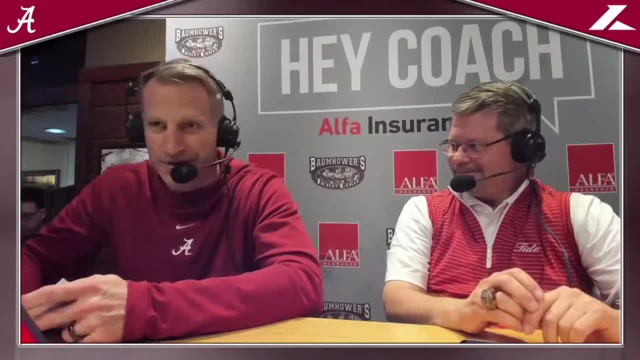 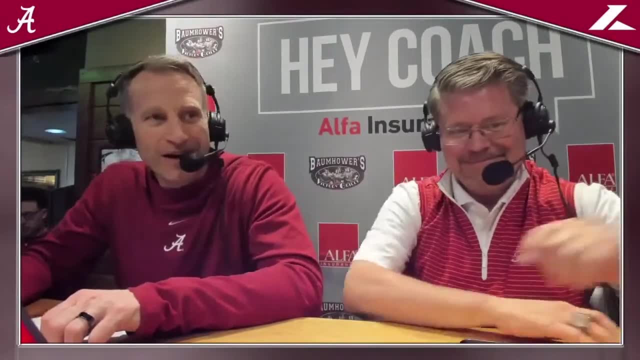 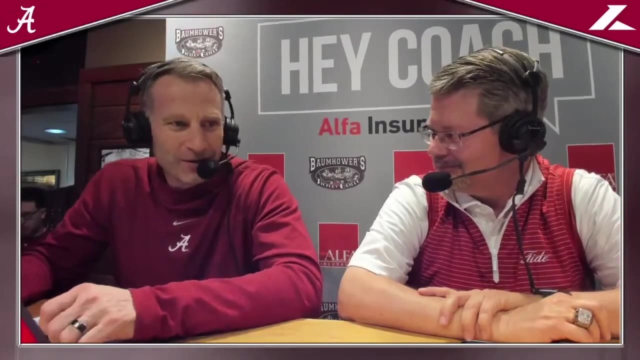 I'm sorry It took five years to get a change, but we got to change. We couldn't have them having the only final four in the state, So we now have one. We're got our hands full trying to get out of that first game in the final four, but we're going to. we're going to give it everything we got I've. 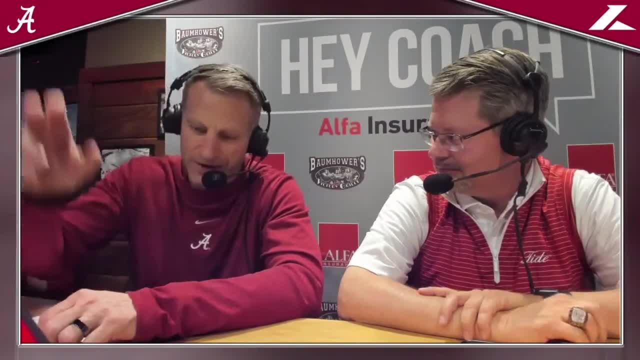 made a quick pit stop. watched a lot of videos this afternoon. quick pit stop here. go home, watch a bunch more video. tonight We'll get a game plan together. Our staff's been on it. We've got some uh. 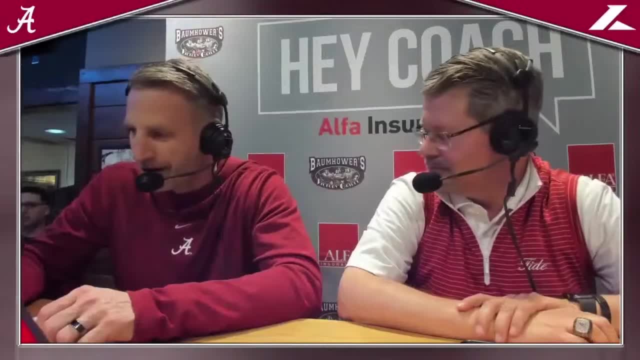 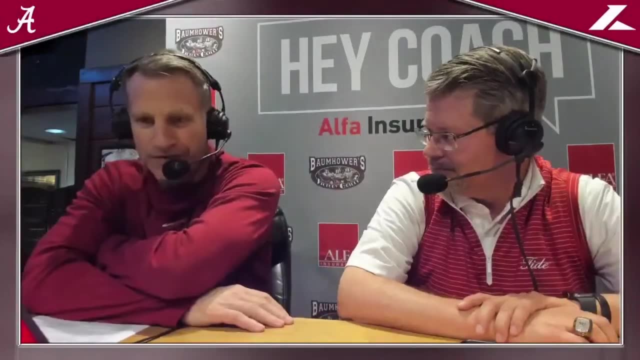 basketball junkies on staff that that have put together some pretty good game plans. We'll we'll get a good game plan in place, And then we've had the players step up game after game after game. So I'm pretty confident We'll have some guys step up on Saturday. 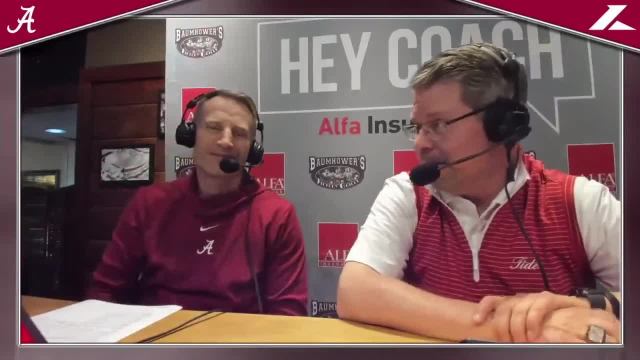 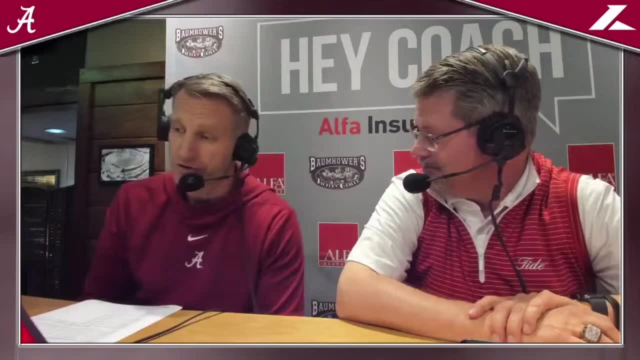 Coach, if they play their best game, they're, they're great. But we've said all along, Alabama's best, on both ends of the floor, is one you'll take your chance with, isn't it? Yeah, for sure, I mean. 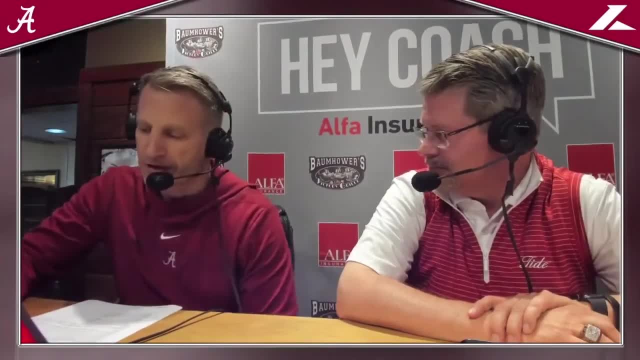 it's. you know we we haven't had. you know we've had a top three defense in the country two out of the last three years- Uh, before this year. we haven't had that this year, but but our defense in the tournament. 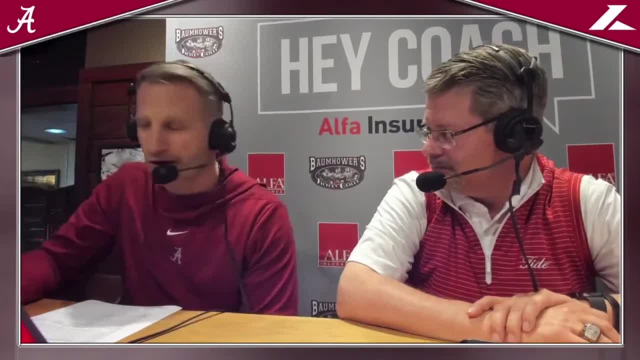 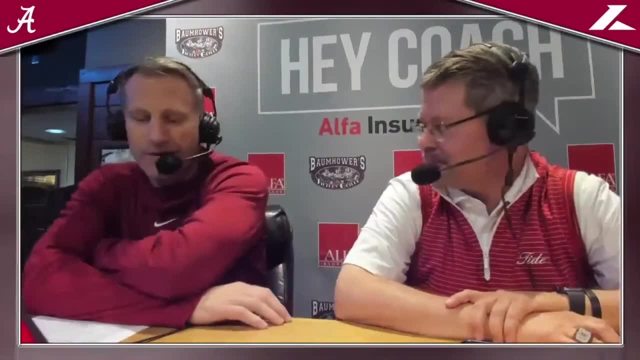 has looked like a top three defense in the country for a majority of it. So we're we're we're getting it together at the right time. You know I if we're playing our best, I mean we've had a little variability in our play this year. We've looked really good. 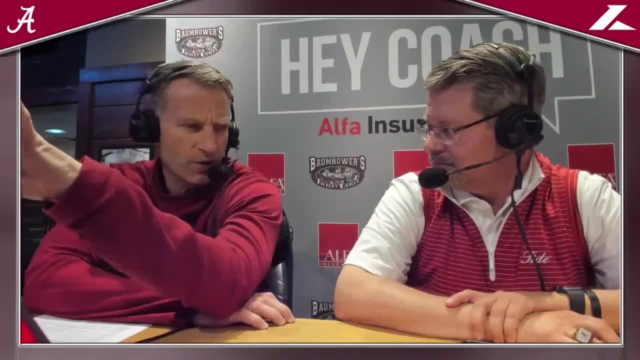 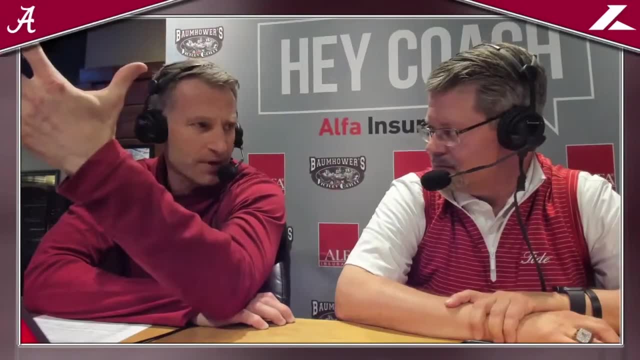 but we haven't had like the really bad losses Like we had two years ago. we, we, we we've lost some games and haven't played our best in those games, but but every loss we've had has been to a pretty good team, Right Like. so you know our, our metrics were always good. 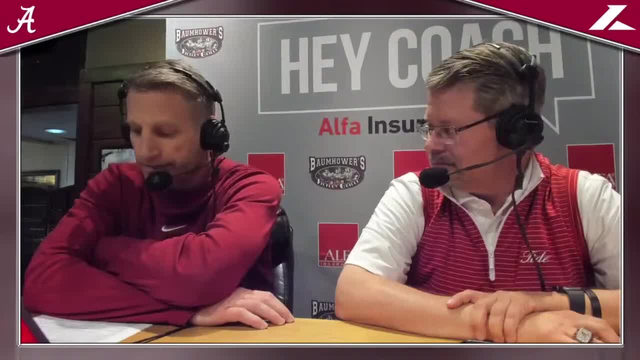 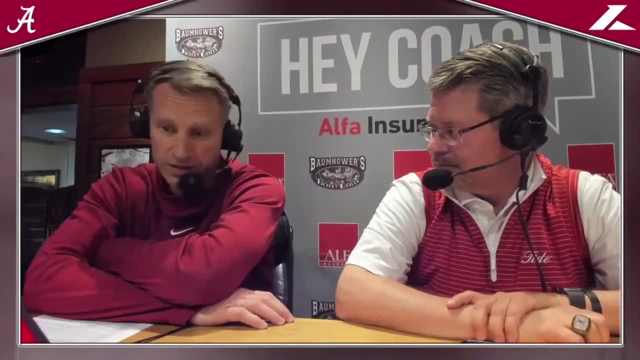 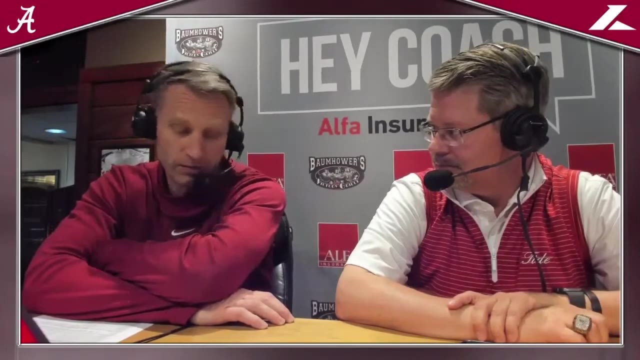 through the year. Now, now we're peaking at the right time and you know, shoot we. we've played Purdue, We played Arizona, We've played Creighton, We played Tennessee. We played some of the best teams in the country. You can kind of go through all those. you know. now we're. we played Carolina. 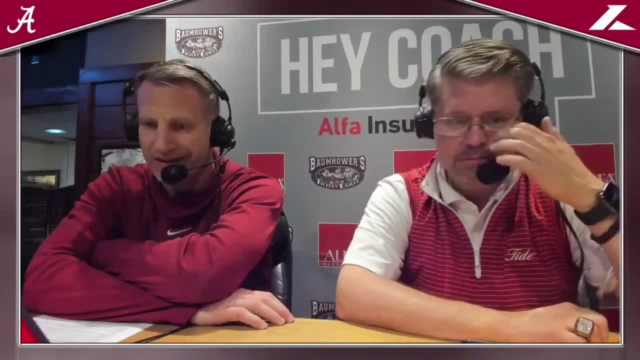 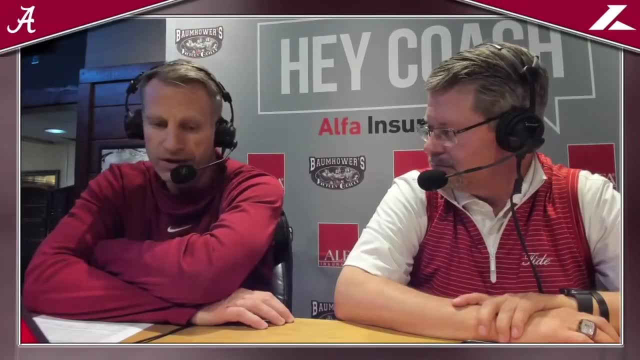 It was a one seed beat them. You know we we've played some quality teams and been right there in the second half up nine on Purdue in the second half. you know the Carolina game shoot. they won the ACC. It's pretty good league Like we. you know we beat them to get here And to me that. 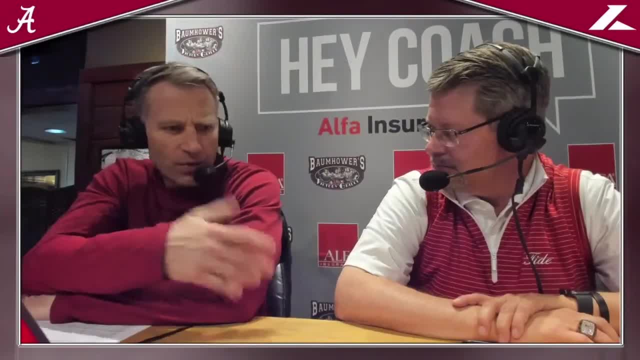 wasn't like a huge. obviously it was an upset. you know we weren't, but we weren't, they weren't favored by that much And we, we, we, everybody assumed we were going to be in the game Like. 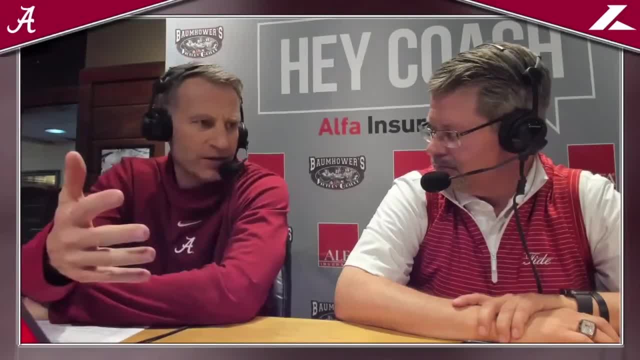 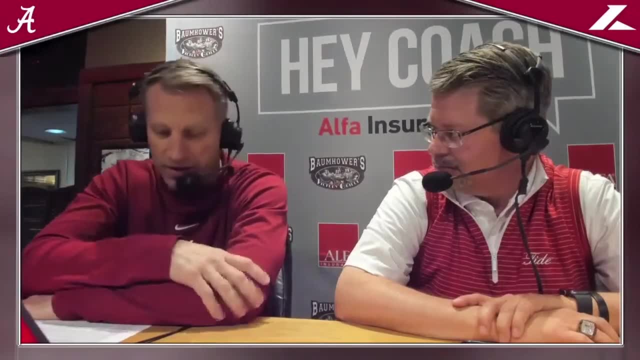 we'd played our. our schedule allowed us to be comfortable playing the best teams in the country. We're going to be comfortable Now. UConn's been playing much better than everybody They're. they're really good, So we're going to have to play well. but I don't think our guys 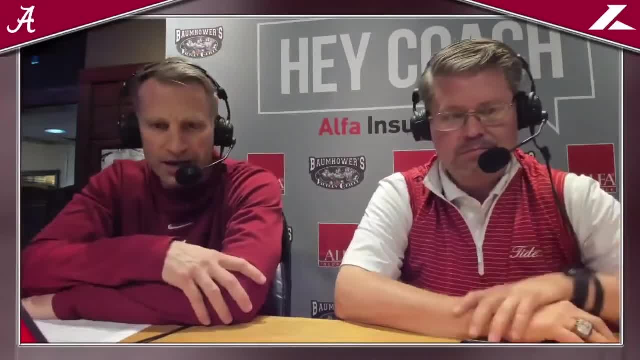 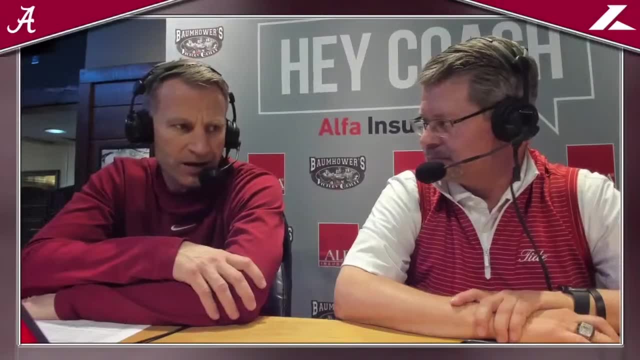 are going to come in intimidated. That's not it Like we. we played some really good teams. Now they're better on both sides of the ball than than most of the teams we played. but we're going to get a game plan together And I can think our guys will come in ready, ready to play with them. 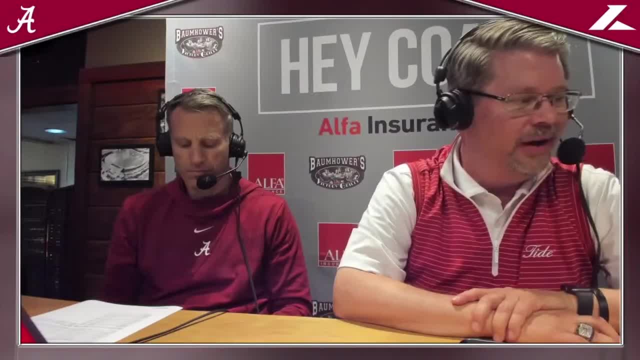 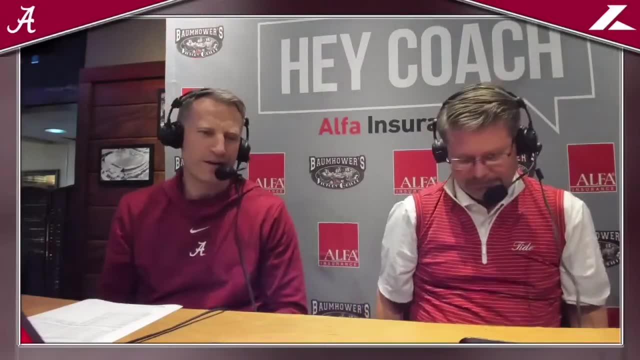 And Grand Bay is where we go to find Peewee and get our first caller of the night, Peewee. go ahead with coach, Coach, congratulations, sir. Thanks, Peewee, Great to hear from you again. One of the better, hey, coach. 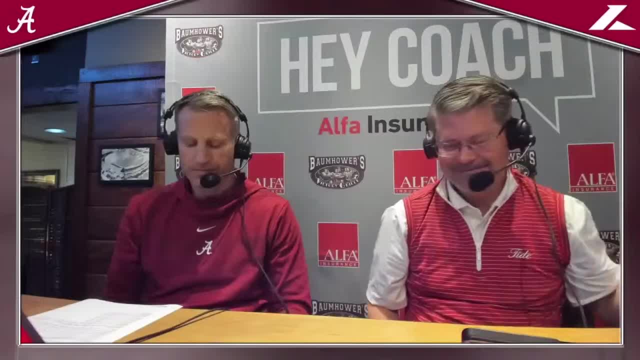 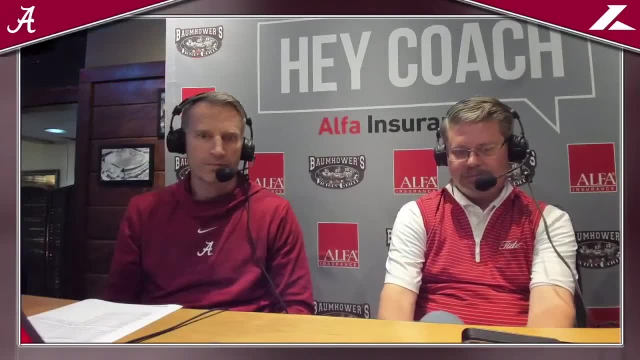 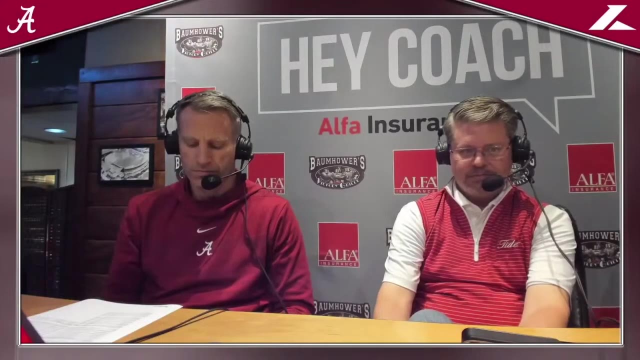 You know, I hear you, you've got your own little club that you joined when you become a coach in the final four. That's very elite club. Congratulations to you, Congratulations to all of our players, especially the ones out there. You know everybody. I know how hard these guys have. 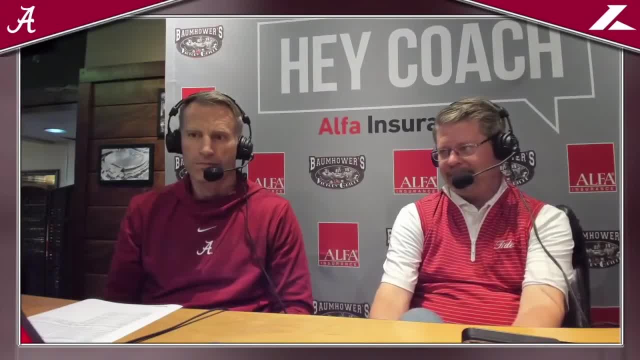 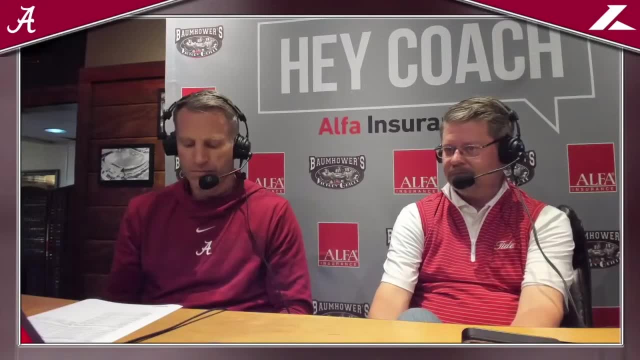 worked. I hope they understand how much very proud we are of them And we got a donning task in front of us, but I think we can do it. So get out there, play our game, push it up transition point. Maybe we can run these guys. 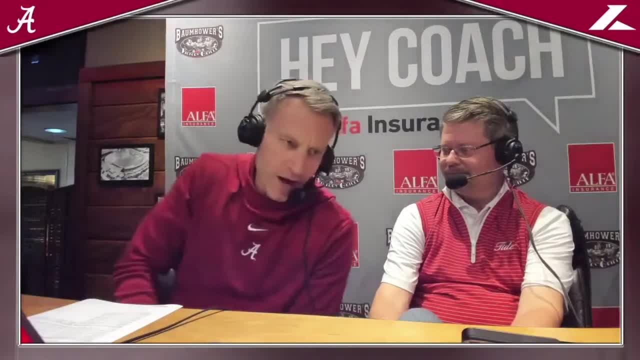 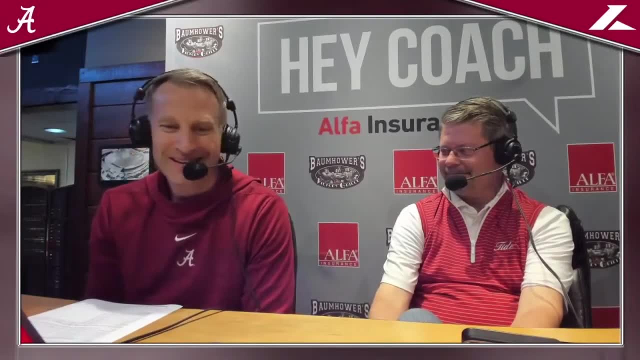 into the ground. I don't know We're going to, we're going to try to run them. They're pretty good in transition themselves. They, you know I, you know the, the, the, the higher scoring the. 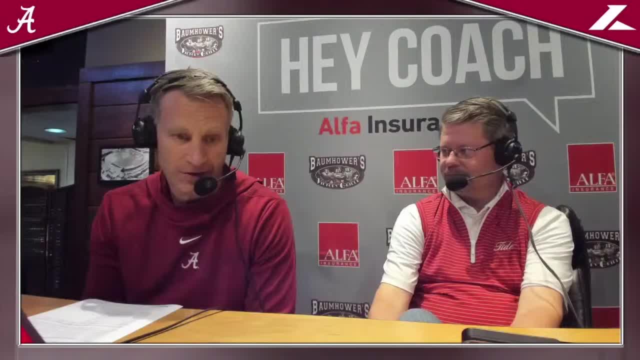 game, I think the better off we are, but shoot. if you watch their Illinois game, that 30-0 run they put on they, they, their transition game looks really good too. So we're going to. we're going to give it a go though. 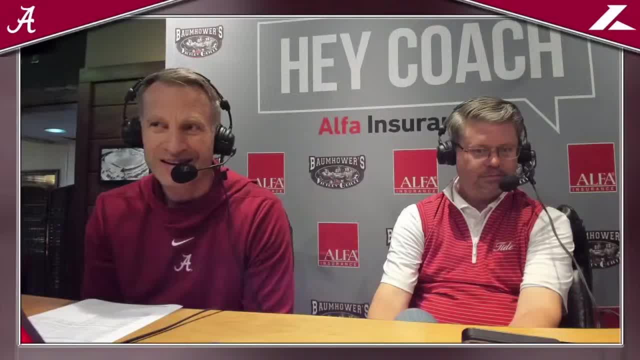 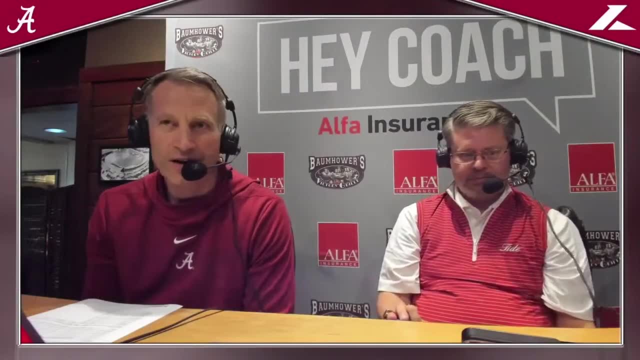 I appreciate the comments. Did you have a question, Peewee? Yeah, I was wondering about Latrell how he was and what's he looking like for this weekend. You know what He's looking better. He still wasn't able to practice today. You know he's still. 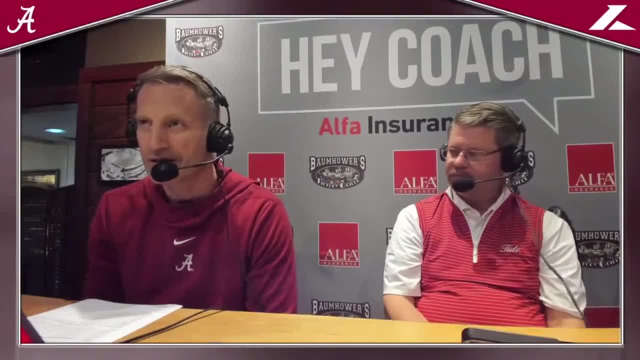 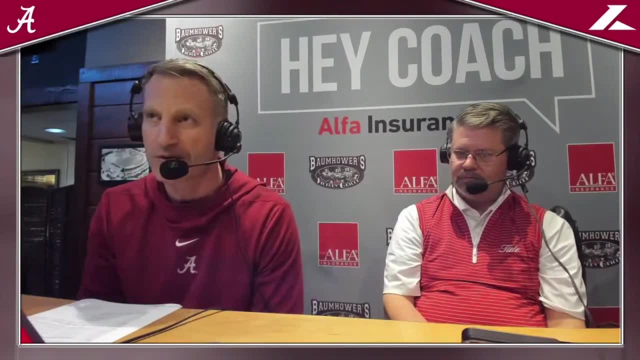 being evaluated every day. but, like you know, with the head injuries, further away from the injury you get, you know, the more likely you are to be able to play. So I think with the week between games he hasn't played. he didn't play all last week. 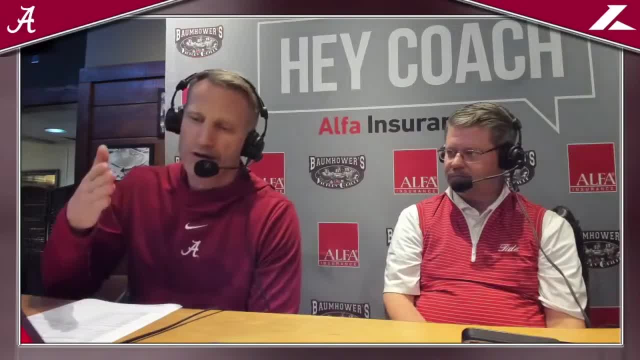 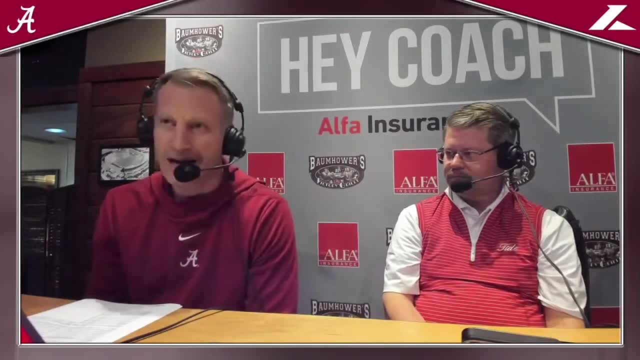 You know I, I think we're going to get. you know he's got, he's got to be able to go through skill workout, then be able to practice and then still not have any- you know, headache or whatever it is. You know the father, they've got the whole protocol and you don't want to put a young man's 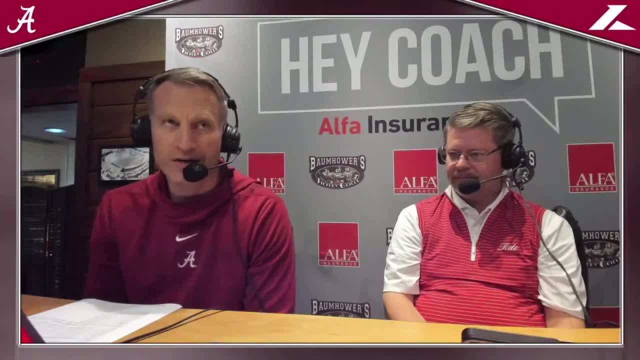 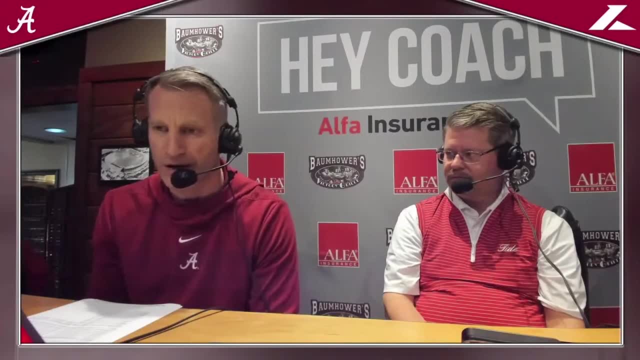 long-term health at risk for one game. So I think our doctor and trainer have been doing the right thing and keeping them out, But I think you know he's going to give it a go. He's going to get it in practice and everything goes, if everything goes well. 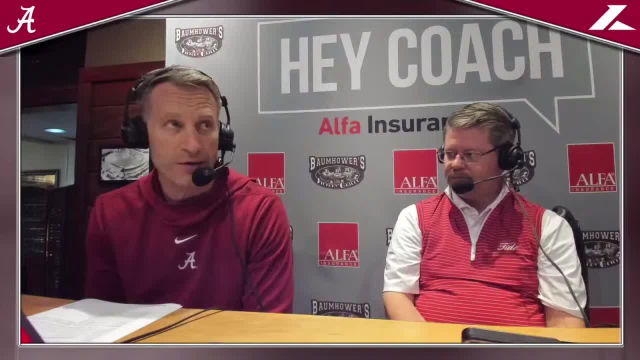 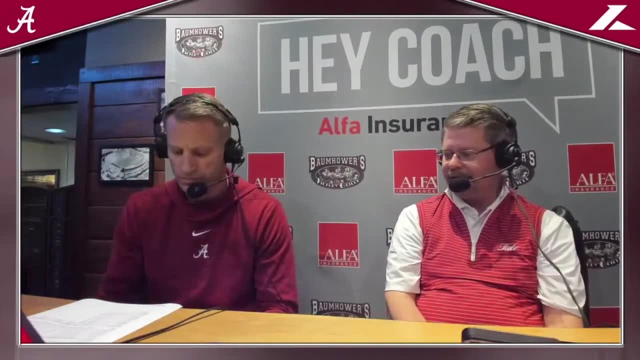 After the practice this week, then he's going to be able to go on Saturday- would be the hope, Coach, we we only have about a minute left with you. Tell us what the next couple of days are like. I know you travel tomorrow, but you don't play until Saturday, So how much of that is to 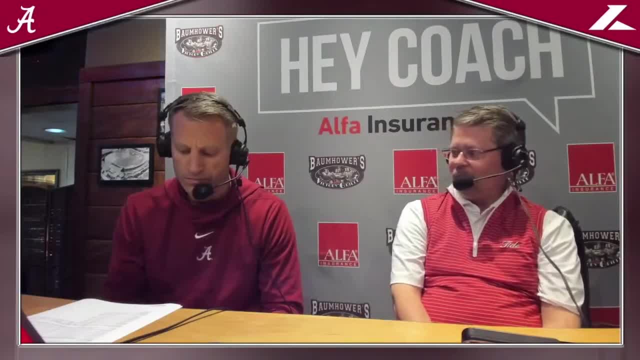 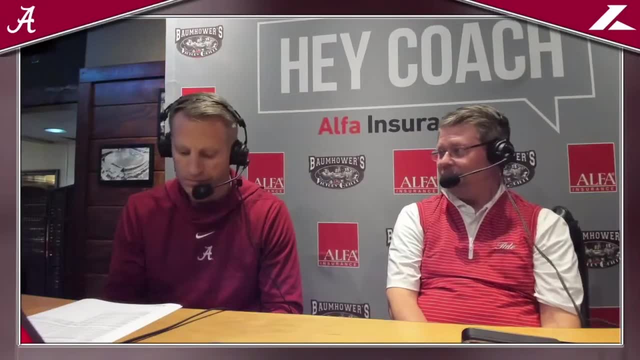 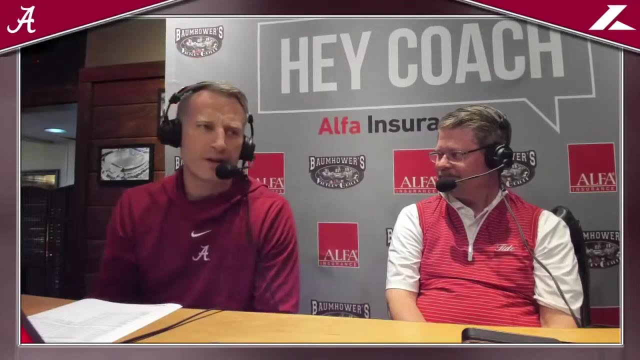 just try to get the legs back under the guys again, and the old radio announcers to get out there and get arrested a little bit early, but also to to take part in everything that's involved with a fight. You know what you know. we practiced a little today but went went pretty light. not much We're. 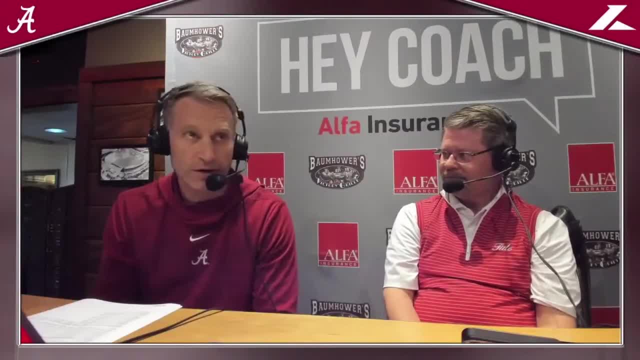 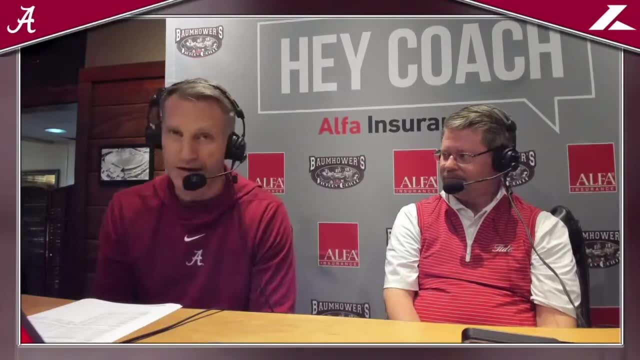 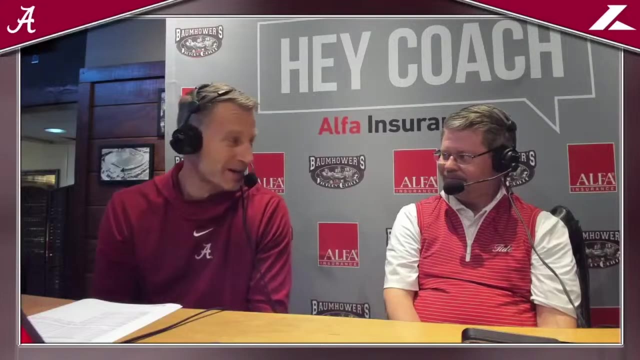 trying to. you know we've been banged up with injuries with Davin's foot, uh, Rachel's head injury, you know, Nick's foot's obviously, uh, not a hundred percent. He really sucked it up and manned up and played well Shoot. It was big for Nick because that Clemson game was against his 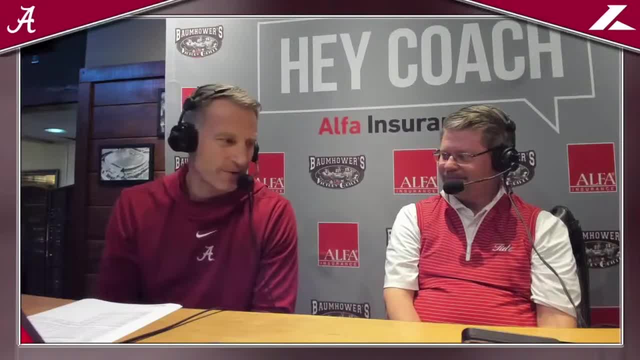 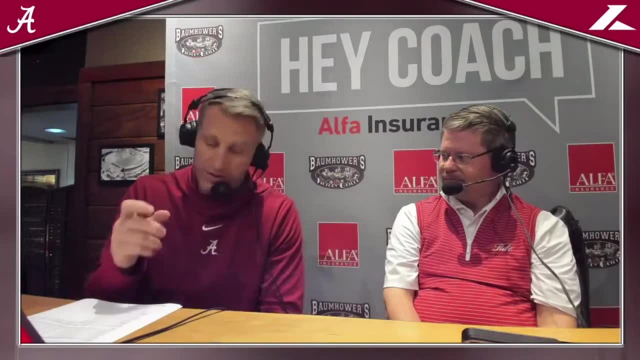 home state team. So you know, in South Carolina, but we're trying to get everybody as healthy as we can over this week while still not losing. I mean, there's a fine line: Can't lose your conditioning, Can't lose. you know how well you're playing, but still want to get healthy and get your. 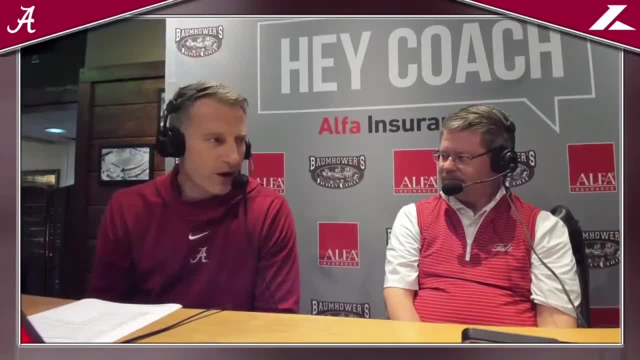 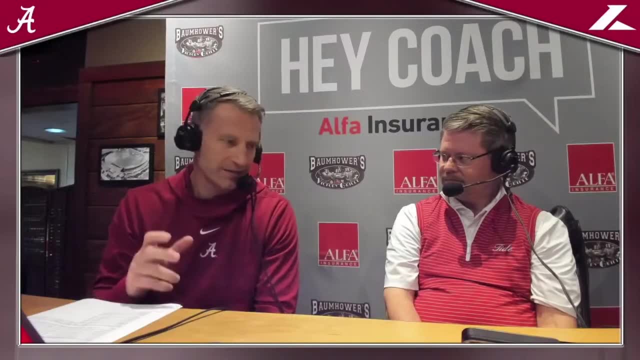 legs under you. So we went a little light today. Tomorrow will be our hardest practice. Wednesday we'll be there. It'll be kind of just a skill shooting day, Not not a real practice kind of an off day, but our guys even on off days getting the gym and shoots. we'll have a gym available. 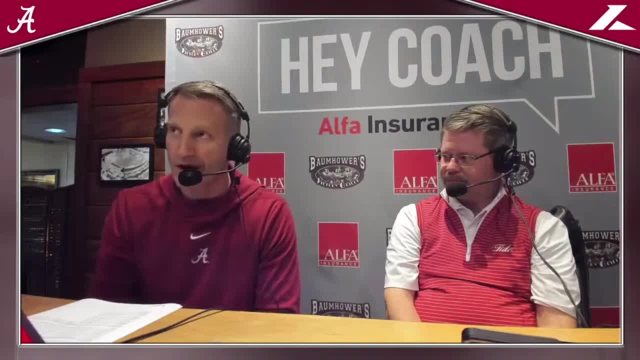 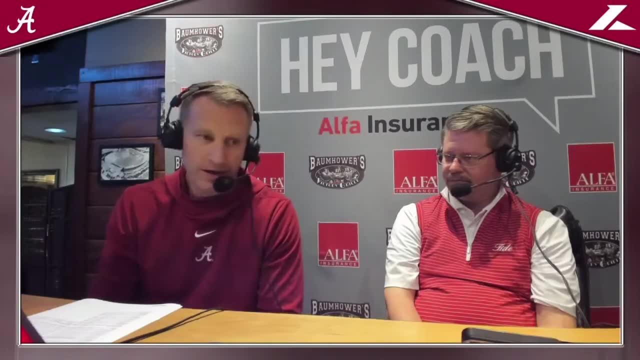 for them to get and shoot. Thursday be fairly light, Friday even though it's a little bit lighter, and Saturday we got to go, So hopefully our legs are fresh. We're playing our best basketball come Saturday- Uh, cause we're going to need to be. we've got a daunting task in front. 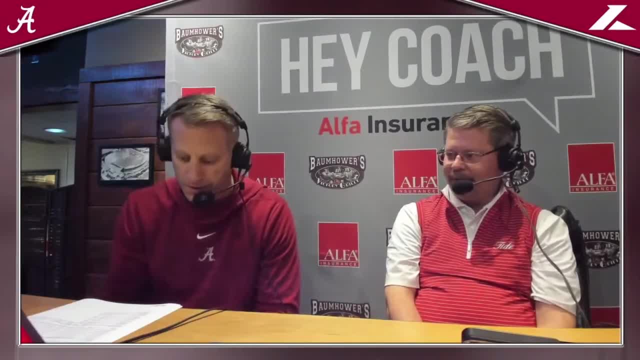 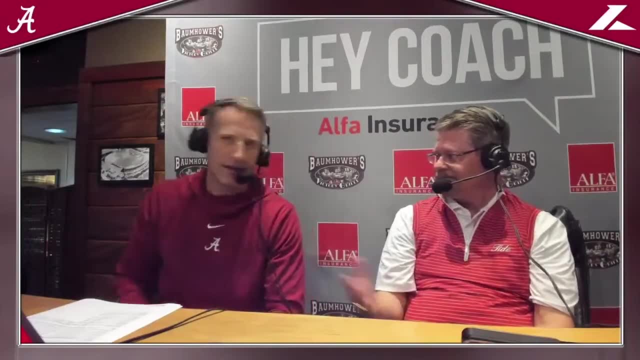 of us with the way you guys playing right now. Well, I hope we see you next Monday, but I hope it's not here, Cause it would mean that we'll be getting ready for national championship game. Thank you And congratulations, Appreciate it. Thank you, Appreciate you guys coming out Roll. 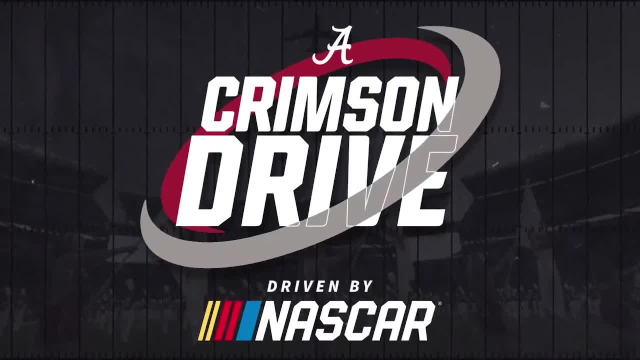 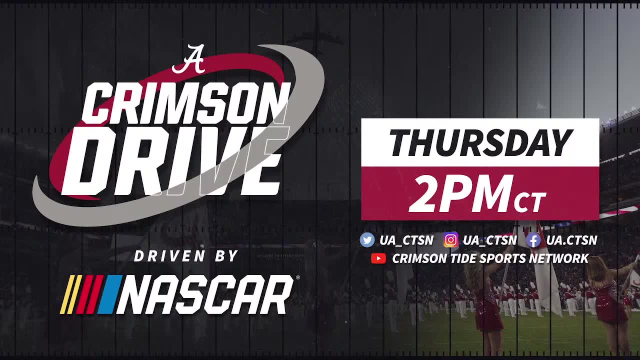 tide, roll tide. Coach Nate Oates with us. NASCAR is returning to one of its most iconic tracks: Energy, the excitement and the powers. drivers battle it out at Talladega super speedway for the guide co 500 on April 21st. lock in your tickets today at Talladega super speedwaycom. 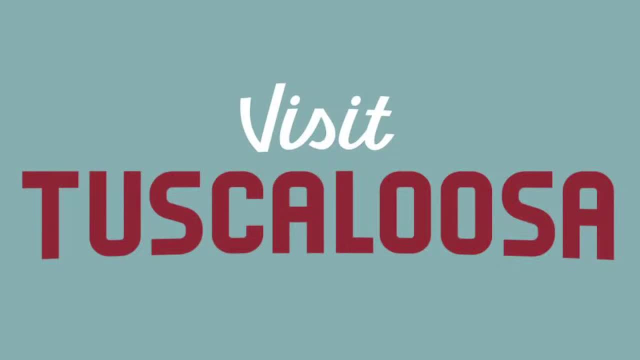 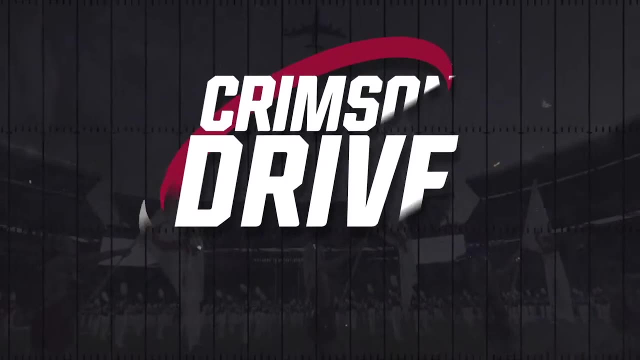 Crimson drive, always sponsored by visit Tuscaloosa as well. Visit Tuscaloosa, your go-to resource for all things Tuscaloosa. check out their events calendar at visit Tuscaloosacom. Well, a busy weekend ahead for Crimson tide athletics. It's time to take a look. 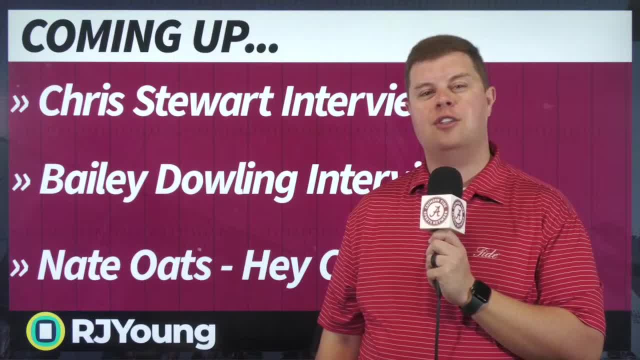 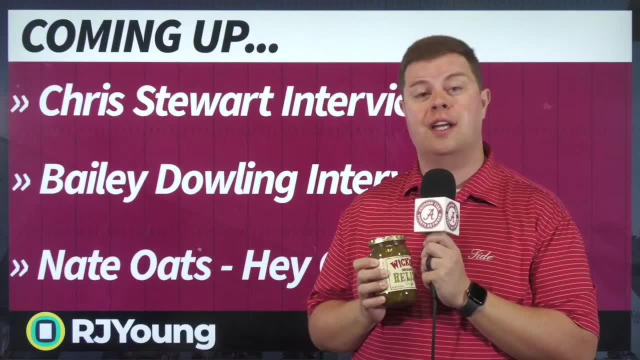 at what's coming up on the Crimson tide sports network with our upcoming schedule. brought to you by Wiggles pickles. They are wickedly delicious. We have the relish with us on set here in Tuscaloosa. Here's what's coming up across the Crimson tide sports network. coming up later today, A new 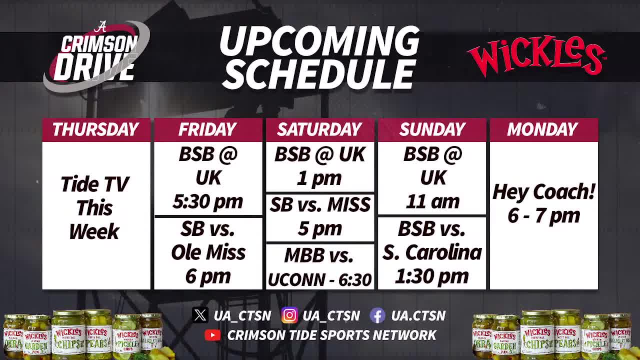 episode of tide TV this week will be available on demand on the Alabama athletics YouTube channel and our TV affiliates around the state And then, coming up this weekend, baseball at Kentucky, starting at five: 30 tomorrow, central, and then softball at home against Ole miss at 6 PM And. 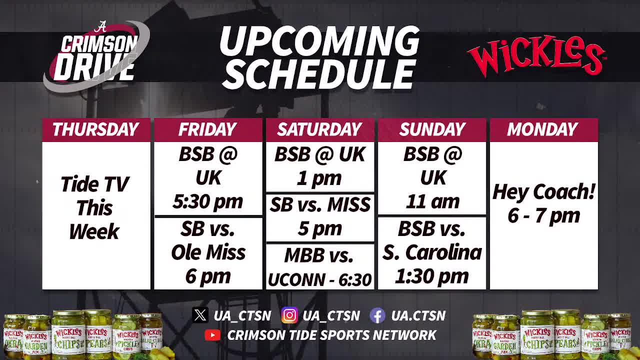 then on Saturday, a really busy day as Alabama baseball will be playing earlier in the day at Kentucky softball at five o'clock And softball should be done in time for men's basketball- Alabama against Yukon in the final four. Our radio start time is 6: 30.. The tip off scheduled for around 7: 39.. Also depends how the first game goes. 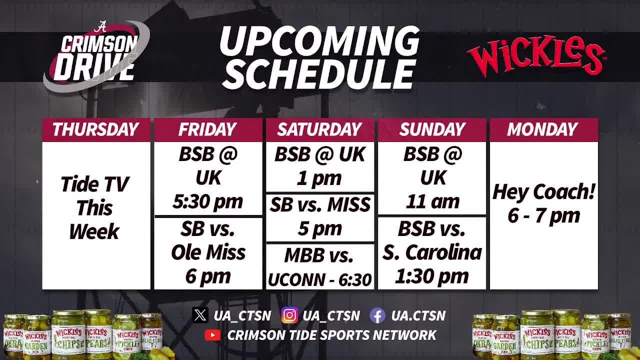 between Purdue and NC state. Then coming up on Sunday the baseball team, with an 11 AM start time against the Kentucky wildcats softball, will wrap up a series against Ole miss And then on Monday night we will either have Hey coach or we will have the national championship game. If Alabama 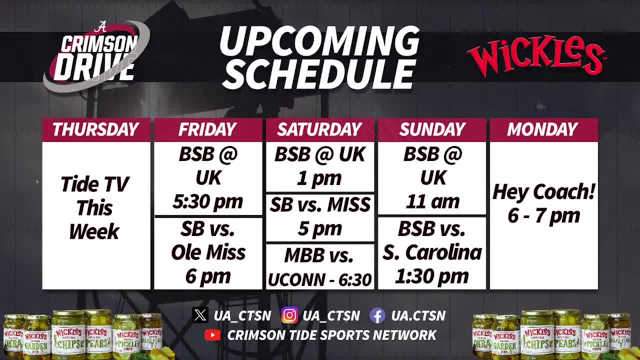 and men's basketball does play in the basketball national championship. we will have the national championship game. There will not be an addition of Hey coach, but we will have full radio coverage of Alabama in the men's basketball national championship game against either North Carolina. 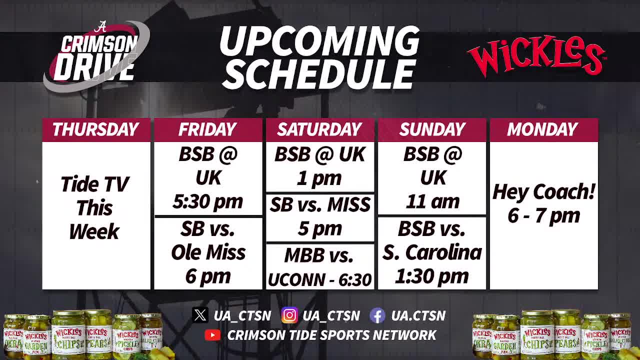 state or against Purdue. more information available on all of our social media accounts. Make sure you're following for a lot of clips and a lot of coverage coming up from Phoenix, from Lexington, and here in Tuscaloosa for Alabama athletics. And that's going to wrap up this edition of crimson. 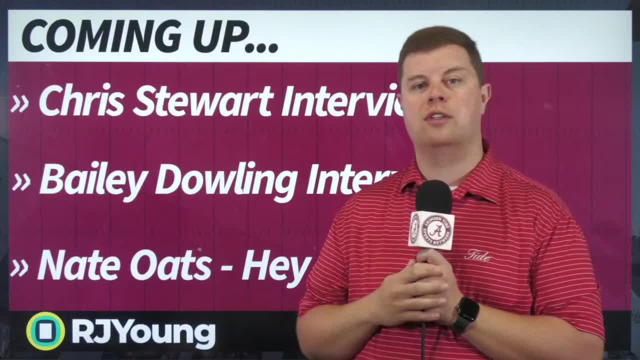 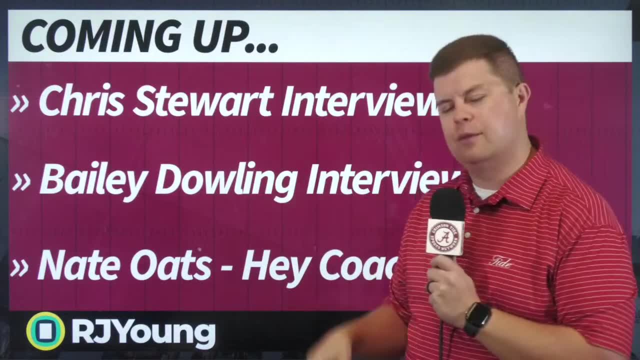 drive driven by NASCAR. special Thanks to our guests: Chris Stewart, who joined us at the top of the show from Phoenix, Bailey Dowling, who again joined us, and the advantage of Alabama basketball And, of course, Nate Oates, head coach of the crimson tide. best of luck to him and Alabama. 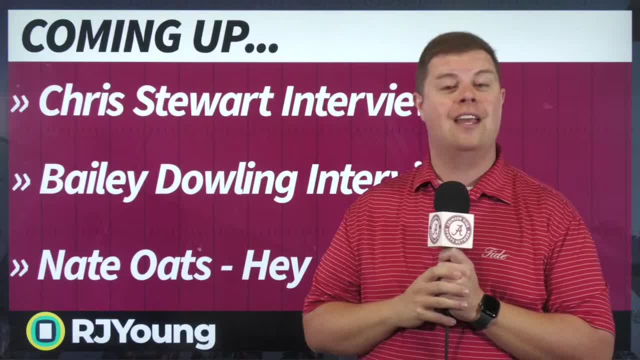 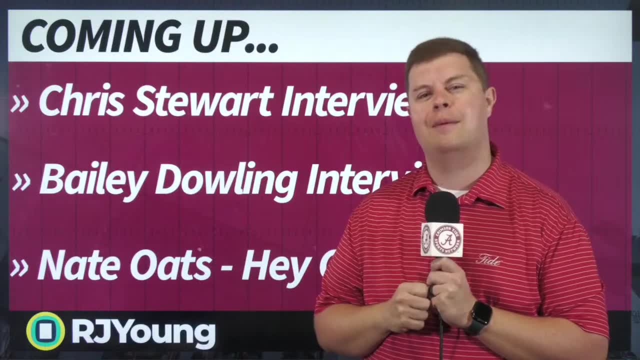 hopefully cutting down more nets coming up this weekend in Phoenix. Thanks as well to our video producer, Ethan carob, And he put this entire show together. Thanks to all of you for watching. Now let's gear up for a great weekend of Alabama athletics and, hopefully, a national championship.